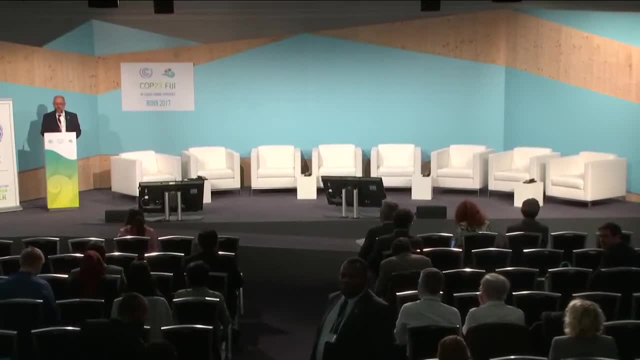 Minister Seriato is Minister for Agriculture, Rural and Maritime Development and National Disasters Management of the Government of the Republic of Fiji. We are very honored to welcome you, sir. As you know, Fiji has the presidency of this COP and this is what we call the Seeds COP. 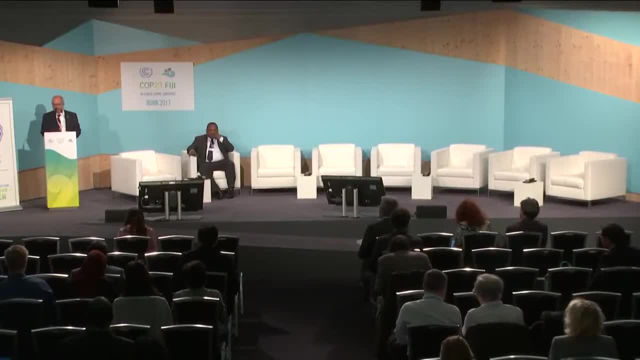 the COP of this year. We are very honored to welcome you to the small island development states. Why that? Because we are discussing on fragile ecosystems and we would like to listen from Minister Seriato, who is the champion on climate and leader of this Global Climate Action Initiative under the Secretariat. 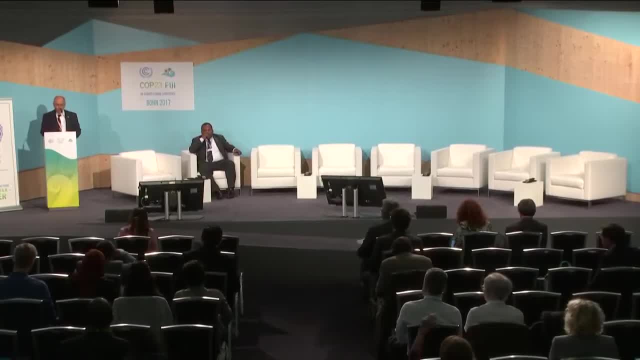 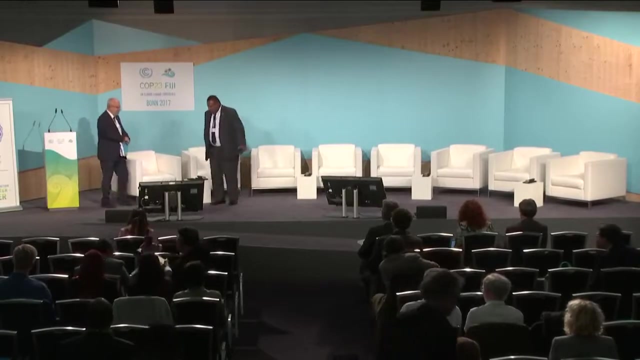 how soils and sustainable soil management could respond to the issues that we are discussing here today. Without further ado, Minister, I would like to pass you the floor. You can speak from there or from here, wherever you feel more comfortable. Thank you, Mr Moderator and Excellencies. 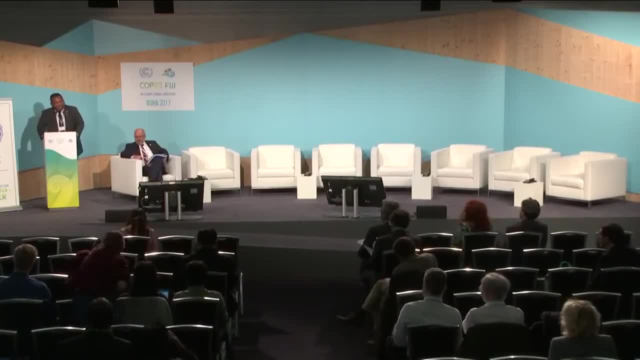 Good day, Guten Tag, And I am indeed honored and privileged to be here with you this afternoon For this very, very important event as part of the thematic day for agriculture. Excellencies, you all agree with me that agriculture is so important. 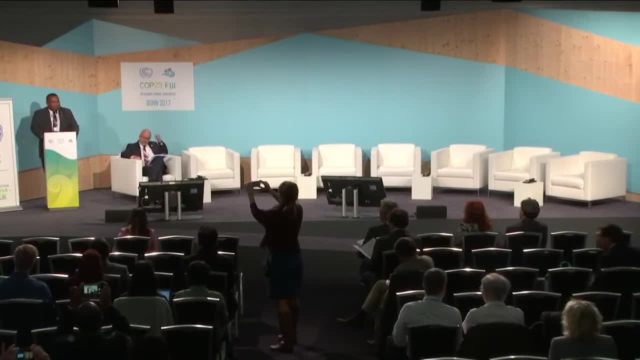 7.5 billion people on planet Earth needs to be fed And, most importantly, there is indication that the global population will again increase in the years to come, And therefore the challenge that we face is about providing food, And it's not only about food security but, most importantly, nutrition security as well. 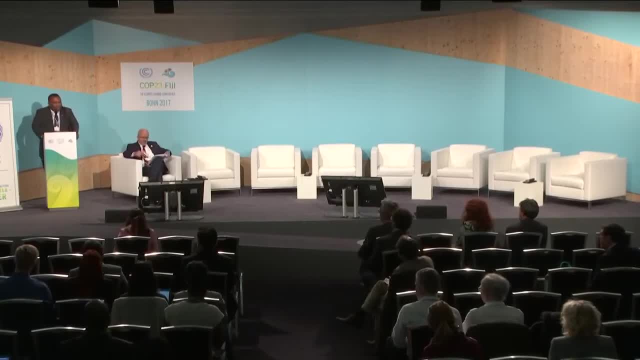 I come from a small island, Pacific Island country very vulnerable to the effects of climate change. I have been asked a few questions about climate change here in Bonn And I am telling the audience that you don't have to ask me about climate change. 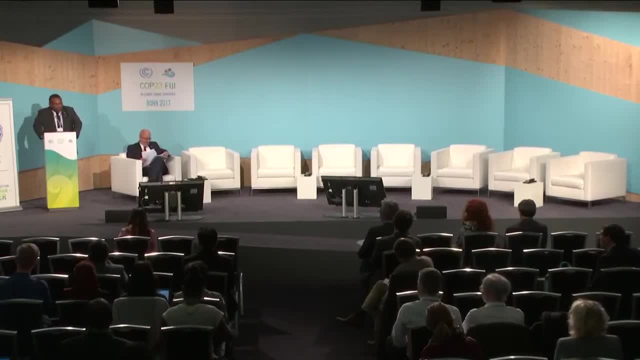 Because I am already experiencing climate change in the islands. It threatens us in so many ways, And for agriculture specifically. I'll talk about a few issues. One: it's the devastating effect of what we call climate-induced disasters. In 2016,, February 2016,, we had Cyclone Winston, a Category 5 cyclone. Prior to that, in 2015,, we had Cyclone Winston. In 2015, in the South Pacific region, we had Cyclone Pem, which devastated Vanuatu and other small island countries within the Pacific. For Fiji alone in 2010,, we had a Category 4 cyclone, Cyclone Thomas. In 2012,, another Category 4 cyclone, Cyclone Evans, And then in 2016,, Category 5,, Cyclone Winston. This is the new norm for us. The way we live is changing And therefore the way we do. development must also change. 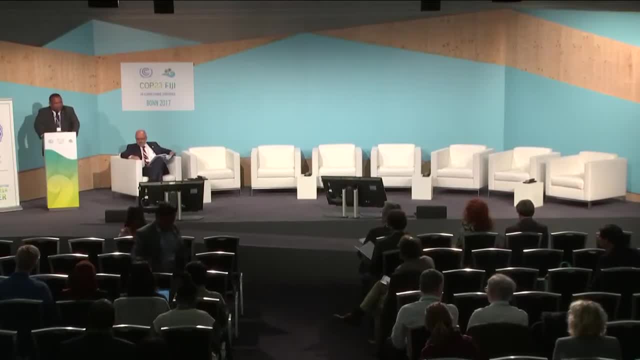 And the way we do. cooperation must also change. This is all important for all of us. I am saying that climate change has affected us small island vulnerable countries in so many ways. Cyclone Winston: the damage to the agriculture sector alone was more than 250 million US dollars. 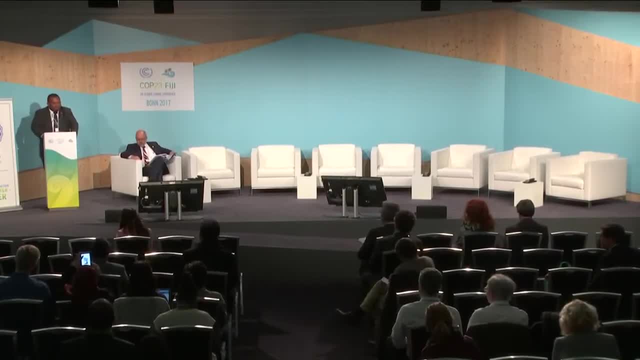 For a small, narrow-based economy like Fiji, this is huge as a percentage of our GDP And when it comes to recovery, it's a lot of effort. It takes a lot of effort and resources to recover from cyclones, from the devastating effects of climate-induced disasters. 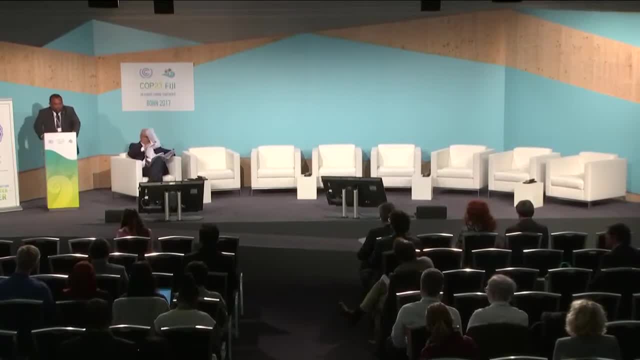 It affects the livelihood of our people, But not only that: social implications as well. People don't want to go back to their respective communities, So there it leads to internal migration and so many other things that come with it: Changing weather pattern. 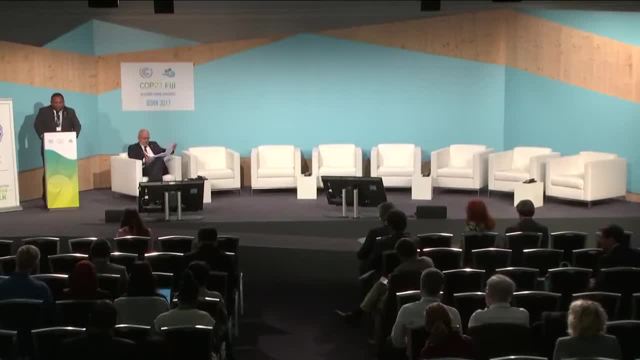 As we speak, in some parts of Fiji, prolonged dry spell for months. Livestock is dying, Crops are dying, Farmers are affected. This is what climate change brings Particularly to us, the small island countries: Saltwater intrusion. 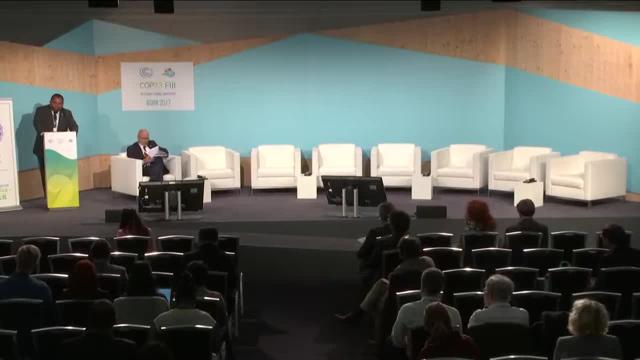 It also affects us particularly because most of our coastal communities they rely on agriculture for their livelihood. About 45% of rural Fijians depend on agriculture as their livelihood And it's the same in other small island countries We are here. 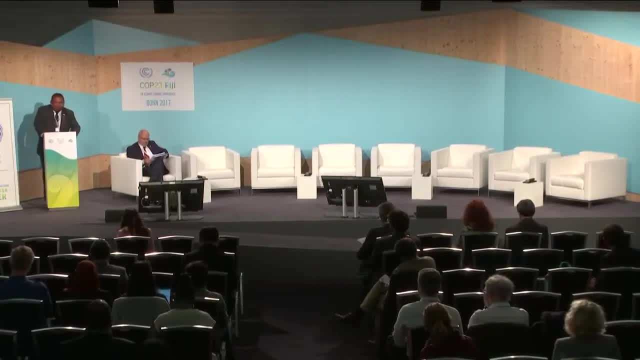 We are here on a very important topic on organic soils. Of course we all understand that we need to produce, but we need to produce at a minimal cost And of course we have to produce not at the expense of the environment. Of course there are negative impacts of agriculture. 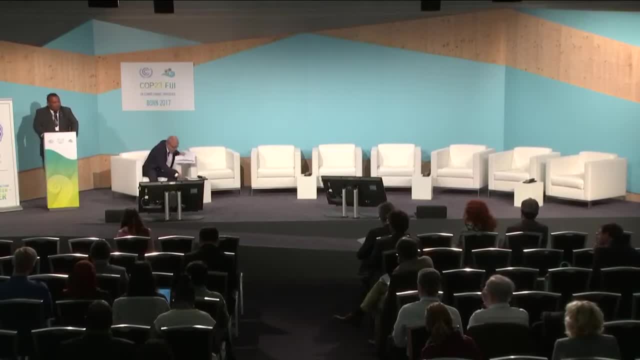 But agriculture- also on a positive note- can also contribute to reducing global warming, And this is why we are here: Excellencies for the solutions And for smallholder subsistence farmers, particularly in the small vulnerable islands that I have talked about. these are options for them. 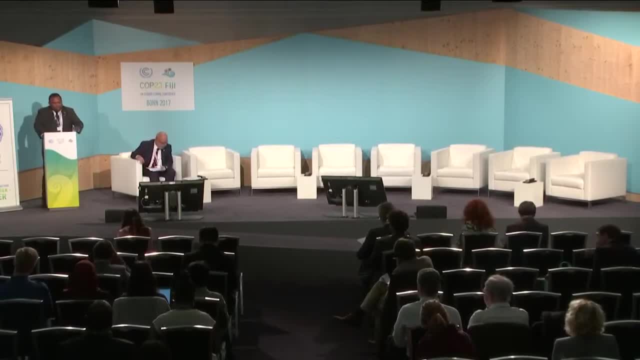 So that they can still produce, but at minimal costs, And at the same time contribute towards reduction in the global warming as well. So I don't want to bore you because I'm not a panelist, But I just want to thank you all. 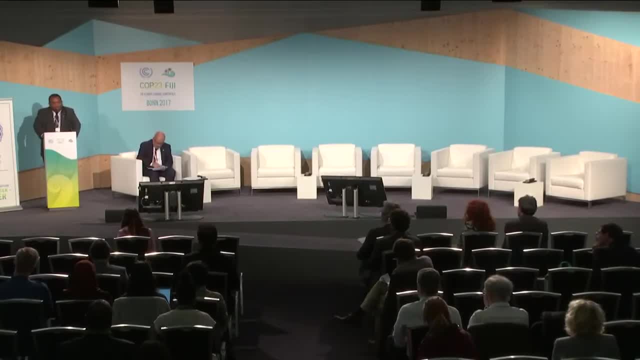 For your attendance And thank you for your support to these climate thematic days. And again, I call on all of us: Let us all unite for climate action Together, Further And faster. Thank you, Many thanks, Your Excellency. 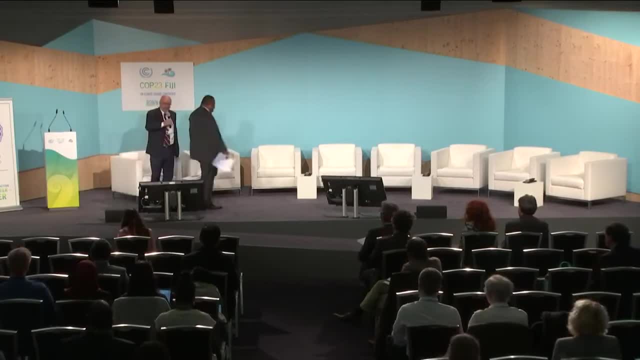 I wonder if you could join us a little bit more. I know that your agenda is extremely busy, But we have two presentations to set the scene And then we are going to sit for a panel And I would like to invite the two presentations. 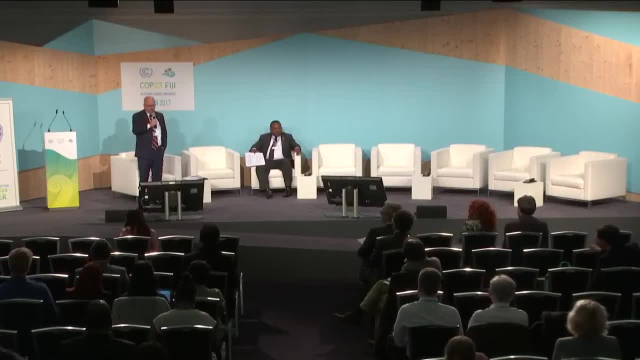 One is on the general aspects, on the global aspects of soil organic carbon, And the presenter is Mr Luca Montanarella. He is the chair of the Intergovernmental Technical Panel on Soils And works at the Joint Research Center of the European Commission. 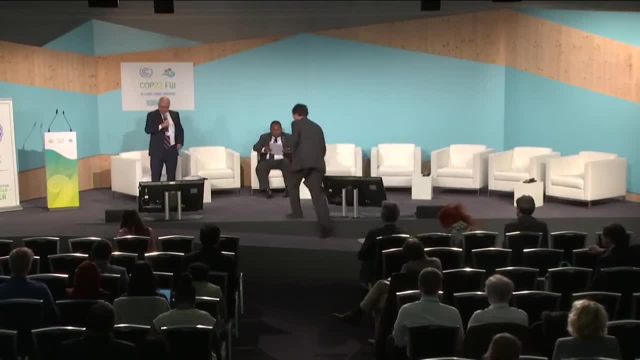 Am I correct, Luca? Am I introducing you properly? You are most welcome. You can use that podium If you are more comfortable, And I wonder if we have the PowerPoint uploaded. I hope so. There is one. Yes, there is one. 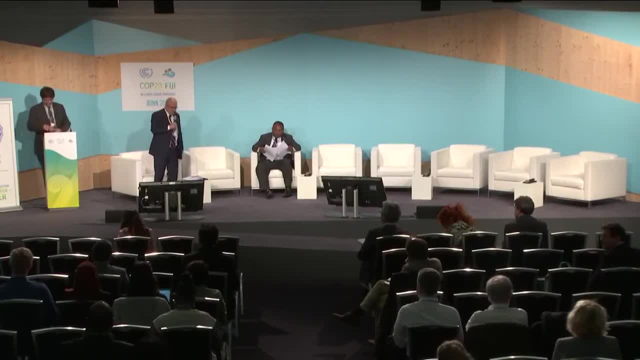 So the colleagues are going to make sure that it comes up And then, after Luca, we will have a presentation from Mr Tekini Nakidakida. Am I correct, Tekini, With your name? Yes, You may want to join us at once here. 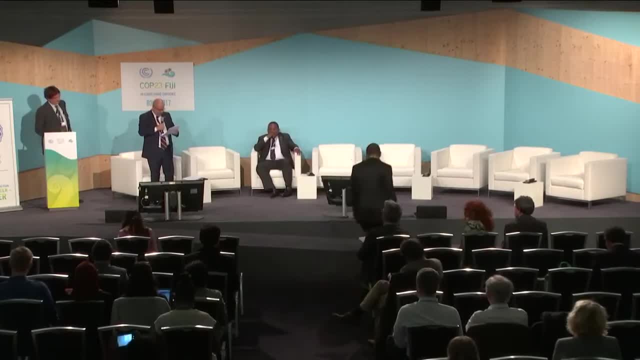 Because we can see the presentation in the screens And Tekini is also from Fiji. He works at the Ministry of Agriculture, So please you can escort Mr Minister there And not feel alone, And Tekini will talk to us about soil management and climate change mitigation and soil organic carbon in the Pacific Islands. 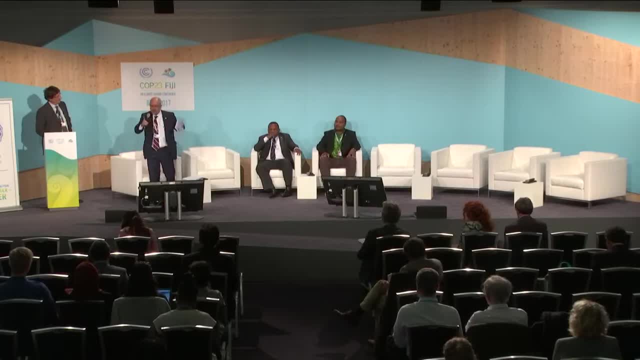 After these two sessions, we are going to bring a panel And we are going to try to do the panel as much interactive with you as possible. So, Luca, the floor is yours for setting the scene at the global level. Thank you. 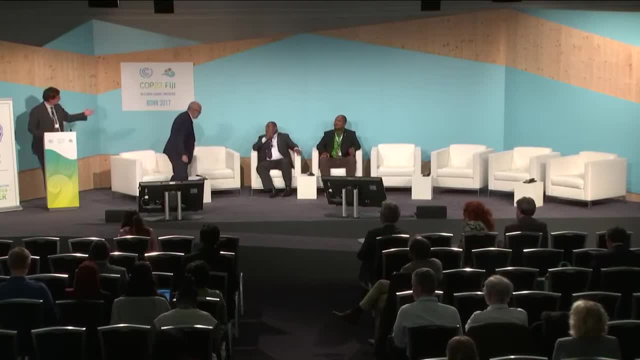 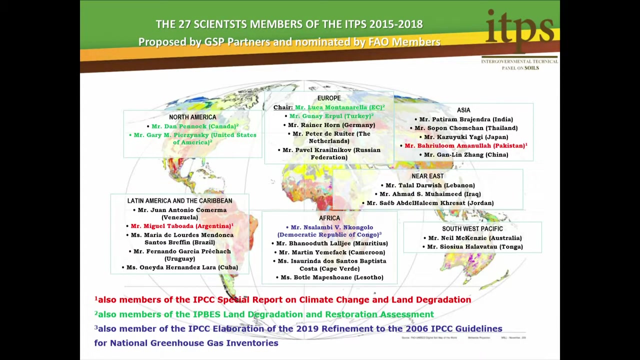 Thank you very much, Eduardo, And good morning everybody. honorable minister, ladies and gentlemen, I will very briefly introduce to you the outcomes from a symposium we organized jointly as a collective presentation of the panel that I'm here representing. As Eduardo was mentioning, I'm working at the European Commission where I'm dealing with soils. 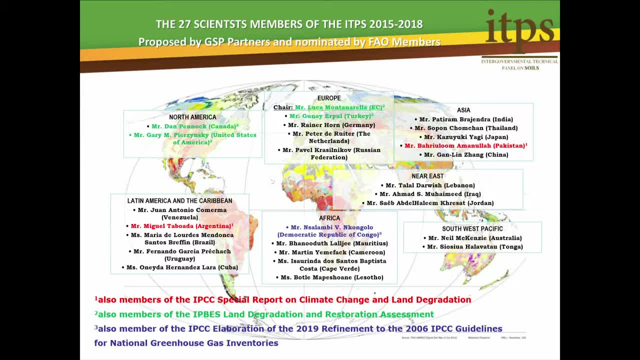 But I'm also currently chairing the Intergovernmental Technical Panel on Soils, which is a body embedded into the Global Soil Partnership hosted by FAO, And the panel is made up of 27 colleagues, scientists nominated across the globe. 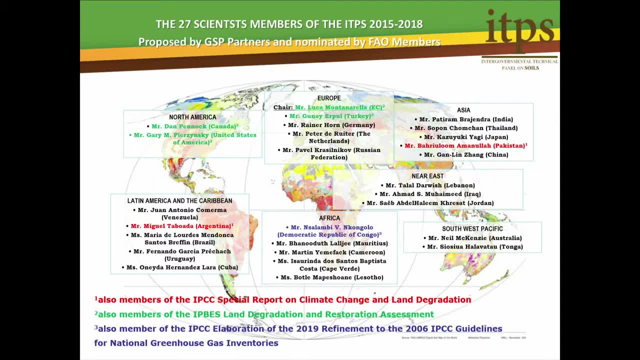 Some of them are also involved in IPCC and in IPBES, So we try also to ensure the cross-cutting collaboration with other similar panels dealing with similar issues, as soils are a cross-cutting issue and needs to be dealt in a multidisciplinary way. 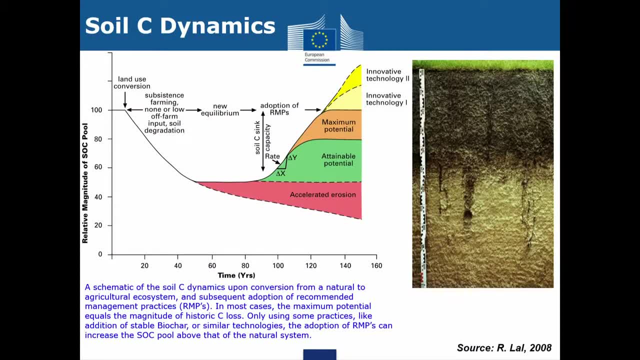 I will spend two words before I talk about the outcome of the conference. First, I want to mention the importance of what we are passionate about in our work As soil scientists. we are passionate about soils, And when we talk about soils, this means we are passionate about what happens below ground. 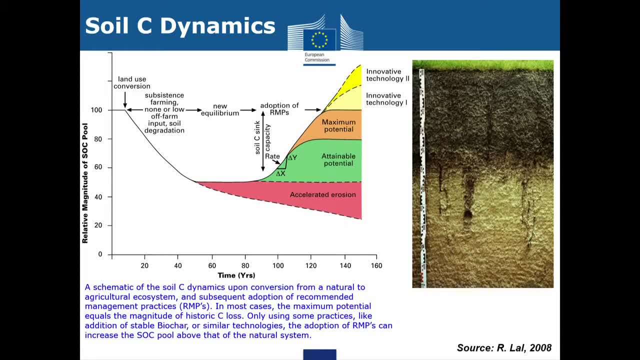 Particularly in this session. we are passionate about what happens to the organic fraction which is in the soil profile, So the organic matter that you will find when you dig a hole in the ground. This organic matter is well known to the scientists because it has a very complex equilibrium. 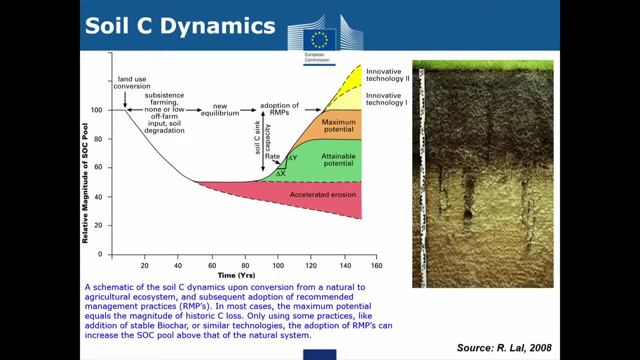 What is particularly interesting is to understand the relation over time, under different management practices, of the organic carbon pool in the soils. In this graph that you see here, you see the amount of carbon in relation to the time And if you go on a natural condition, you will have a certain level of carbon in your soil. 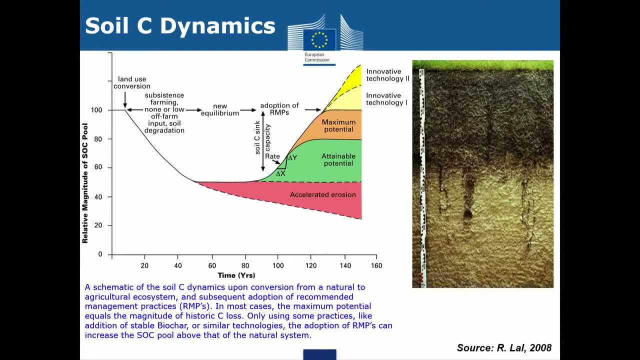 And if you start doing some land management of any kind, you will have a change, And usually this change is a decrease of soil organic carbon over time. Still, you stabilize your carbon again at a certain level. that will depend on your management practice. 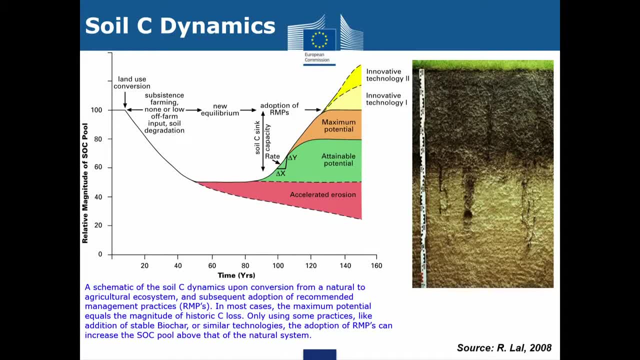 If your management practice is not a good one, you will continue depleting this carbon. This is the red part of the graph that you see there. If your management practice is a positive one, you will build up your carbon again, possibly to the level of the natural climax situation. 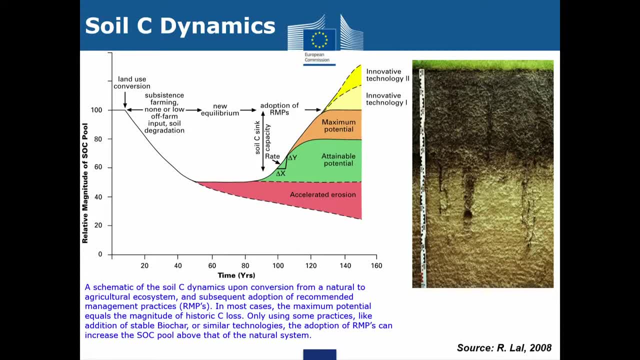 But maybe with new technologies- and I will also mention that- you can even go beyond the natural capacity of soil to store carbon And accumulate above the natural stable amount of carbon that, in that condition in that site, can be stored in the soils that you are currently managing. 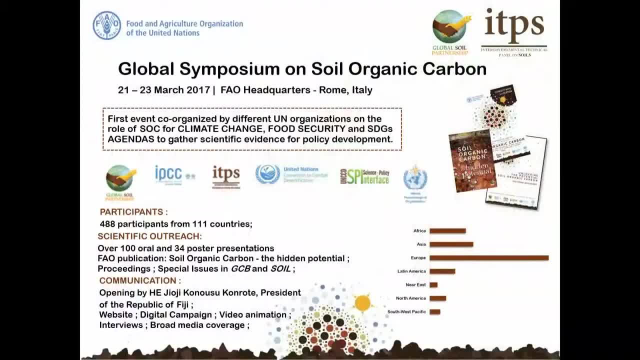 Now, all this just to introduce that we had a very important event this year, hosted by FAO in Rome in March- 21st to 23rd of March- And the interesting bit of this event was that, for the first time, we had a joint event between different organizations on this cross-cutting issue that is soil organic carbon. 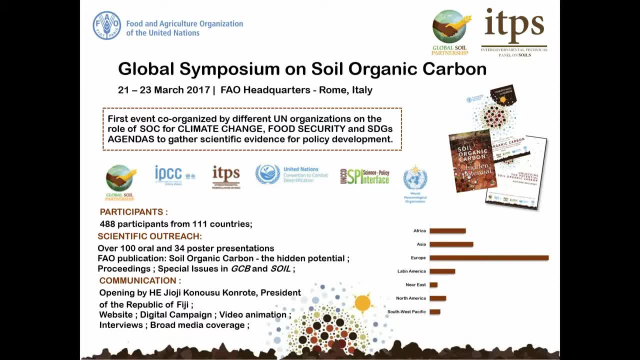 Carbon management at global scale. It was somehow coordinated effort from the different panels from the scientific point of view. So the intergovernmental technical panel on soils which I'm chairing, but also together with IPCC, IPBES and the Science Policy Intervention of the United Nations Convention to Combat Decentrification. 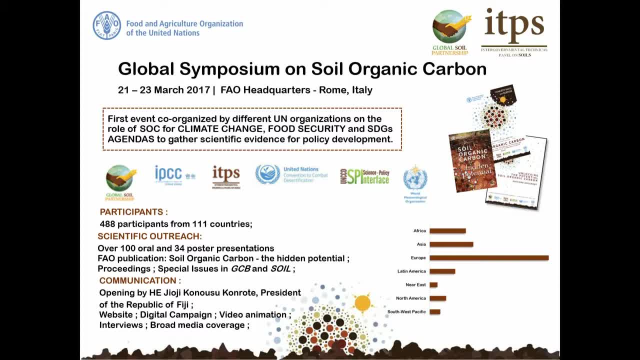 And it was hosted by FAO, and I think it was a big success in this sense because it allowed to bring together nearly 500 participants from more than 100 countries And, particularly, it allowed to bring together scientists together with policy makers. We were enjoying the opening statement by the president of Fiji and also the presence of the two executive secretaries from the United Nations Framework Convention of Climate Change. 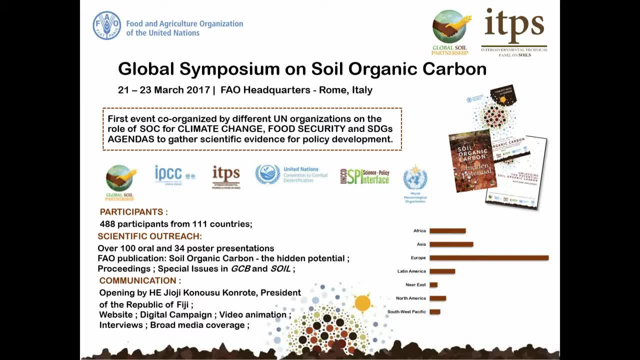 And also from the United Nations Convention to Combat Decentrification, The two conventions that are particularly, let's say, active in the area of soils and particularly of soil organic carbon management. All the outcomes are available. I mean I don't spend more time. 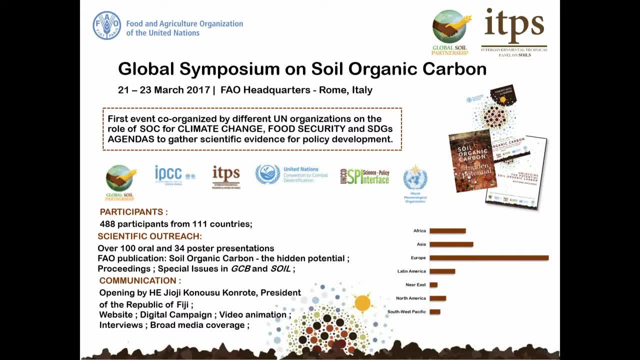 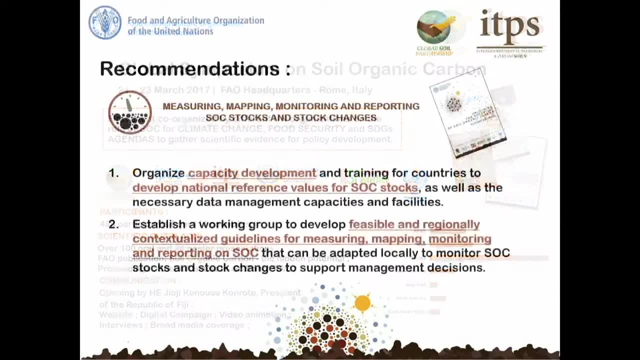 You can download the outcome document as well the related ancillary documentations, presentations and all what you are interested in. Just a few highlights to you of the recommendations. The recommendations, first of all, put the accent on the need to invest in capacity building in those countries that still don't have that much of activities in this area. 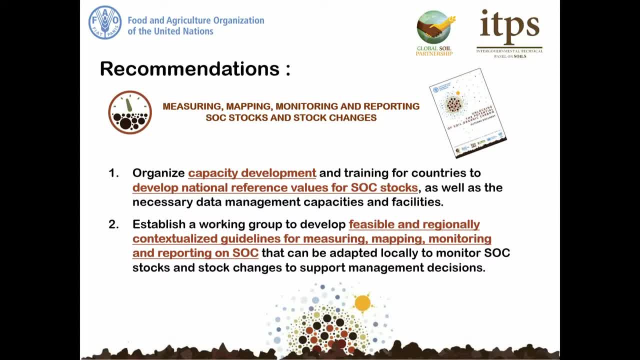 So the capacity development at national level in order to have at national level the necessary data, the information to assess soil organic carbon levels, was particularly the first recommendation. I will come back to that later on during the presentation. Then there was expressed the need to have clear guidelines how to measure and how to verify the levels of soil organic carbon globally and nationally. 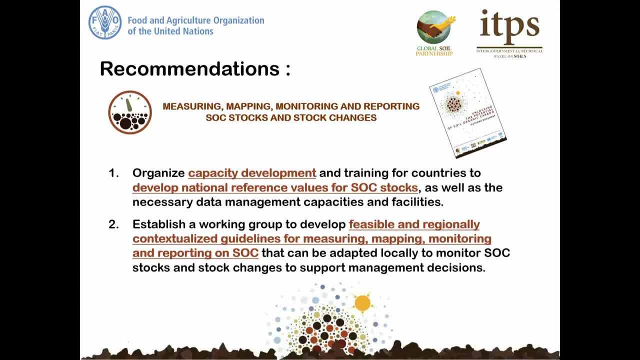 so that we can also report about changes. This is a crucial issue, particularly for this convention. If we are not able to report about changes in soil organic carbon, it will be very difficult to take it into account in any time Any type of climate change discussion. 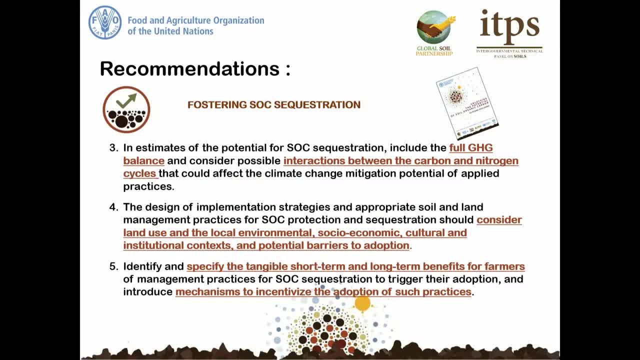 The other recommendations were related to the issue that we must consider carbon in soils also in relation to other issues, For example nitrogen balance. You cannot deal with carbon without dealing with the nitrogen in soils And, as you know, N2O emissions are, on the other side, quite important greenhouse gas factor. 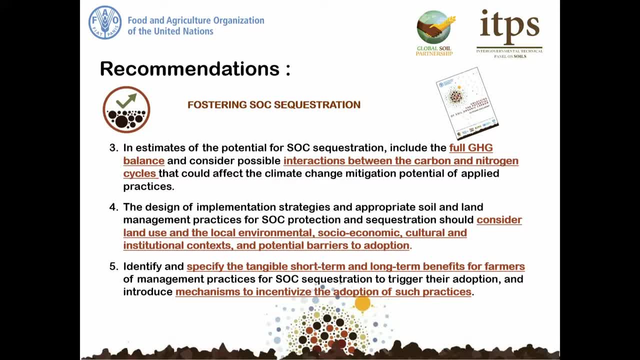 And so you need to consider the carbon management in a more holistic way, in a more interdisciplinary way, And, of course, you must also try to highlight the short-term economic benefits in applying soil organic carbon management practices which are positive in the sense of accumulating and sequestering more carbon in the soils. 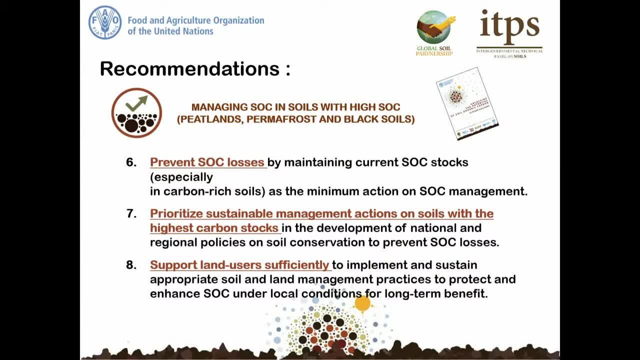 Final set of recommendations was about the need to pay particular attention to the areas which have very high organic carbon levels. You may know that four countries on this planet hold more than 50% of the total soil organic carbon: The Russian Federation, Canada, United States and Brazil. 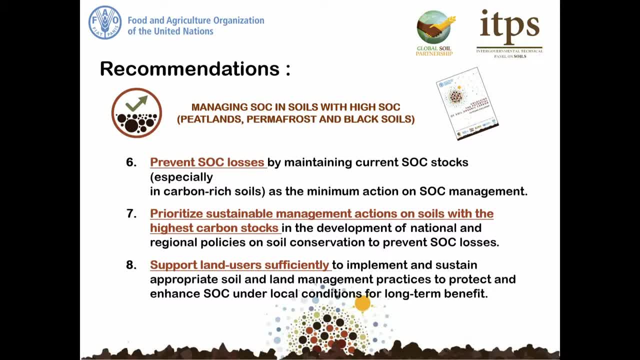 This soil organic carbon pool is very important and it's mostly concentrated on what we call organic soils, So soils which have more than 30% of organic matter, typically peatlands, typically highly organic soils in the boreal areas. So these soils are particularly delicate and should be protected because emissions from these soils could be massive if there is a massive land use change happening there. 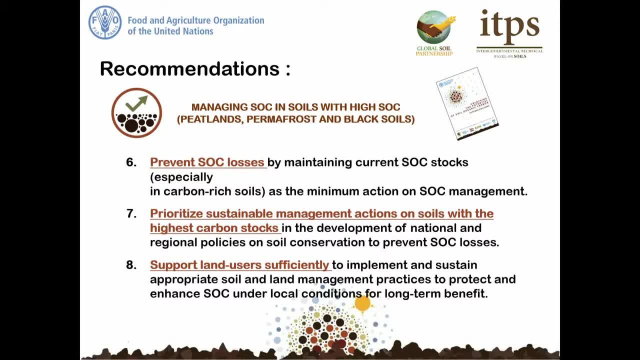 So we should protect these soils, We should prioritize those areas, but also prioritize sustainable management actions there where we can have the biggest benefit on the short term And particularly, of course, always taking into account that the land is mostly in private hands. 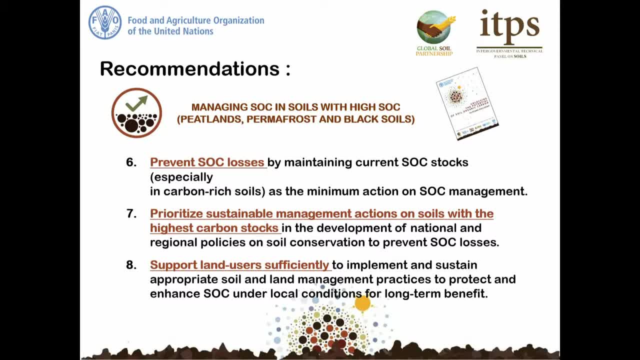 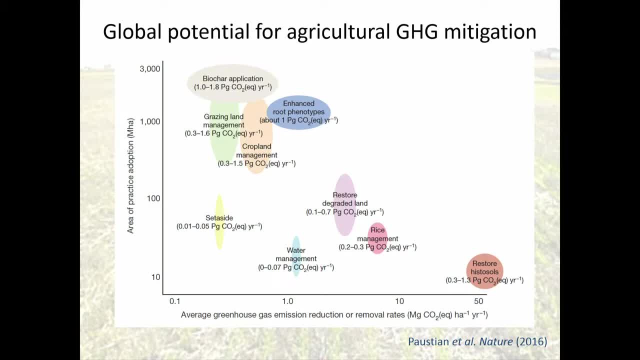 so you need to involve from the onset the local land users and land owners. So just to close to say that there is plenty of literature, also very recent literature, about the fact that there are very effective possibilities to use greenhouse gas mitigation in the agricultural sector, particularly in soil management. 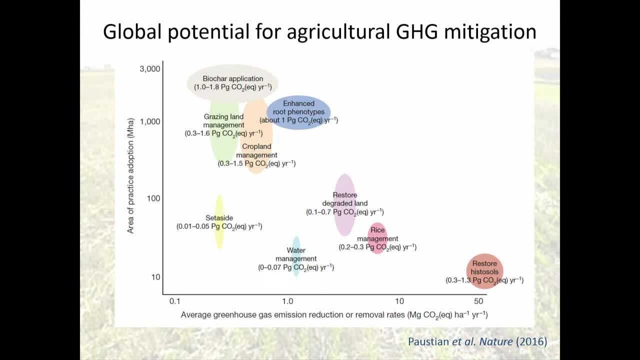 You will find here a graph giving you the potential of greenhouse gas mitigation for different in relation to the area that is affected, As you see, particularly restoring histosol, so organic soils. The far end to the right hand here is having a very high potential in very small areas. 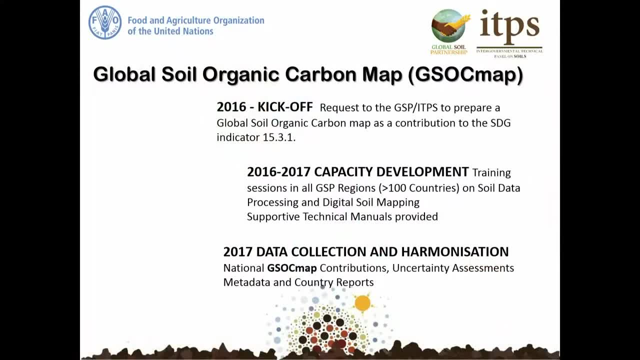 But this, of course, maybe for later discussion. Finally, I would like to close saying that one of the major products that you will see by end of this year will be the new Global Soil Organic Carbon Map, which is a flagship product of the Intergovernmental Panel. 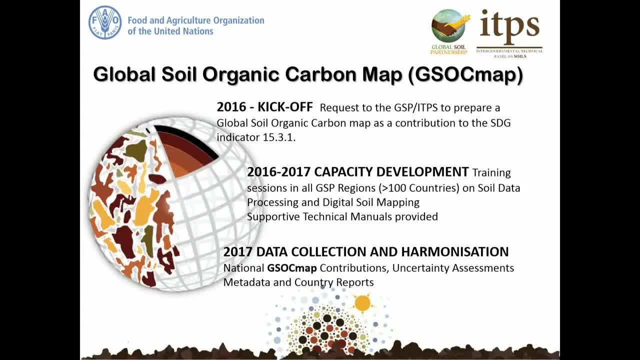 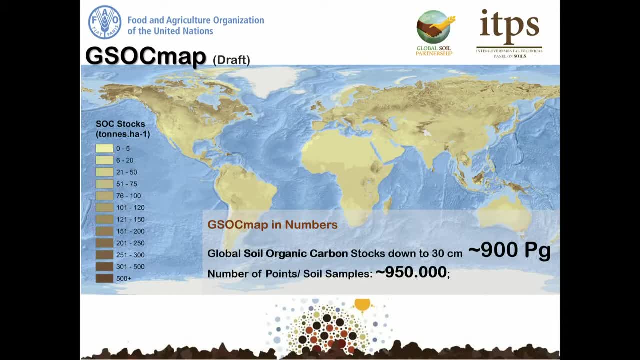 that is currently in its process of being finalized and is a collaborative effort, collecting from national authorities and from national soil surveys soil organic carbon data that are the most updated and most detailed ones, and putting them all together into a global system that is currently under development and will be released officially on the World Soil Day. 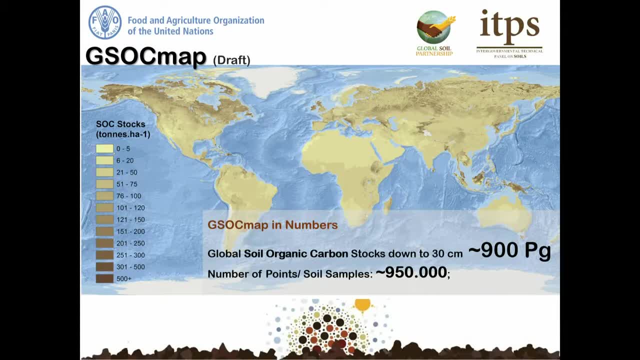 As you may know, it's on the 5th of December. So this 5th of December 2017, we will release the new Global Soil Organic Carbon Map, and you're invited, of course, to consult this data then on the online system that I suppose FAO will be hosting. 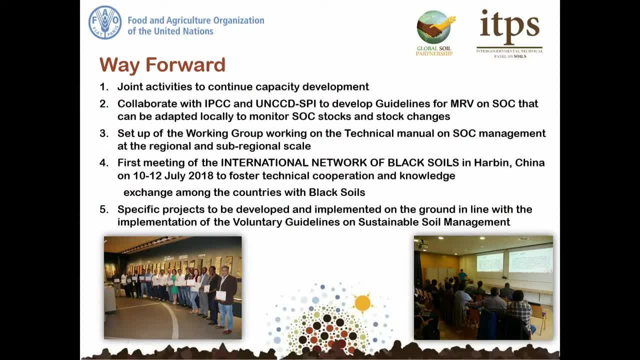 So the way forward for all of us is to work together and to continue developing this field, which is particularly important for greenhouse gas mitigation, And this will be done through various initiatives that are ongoing. The working group that will now work on the methodologies. 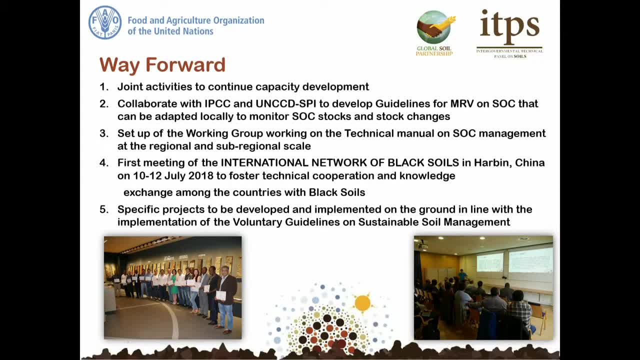 and guidelines for management, but also in the technical manual that will be provided in order to do implementation on the ground Networks that are getting established, particularly on the soils, as I mentioned, that have very high organic level, the so-called black soils. 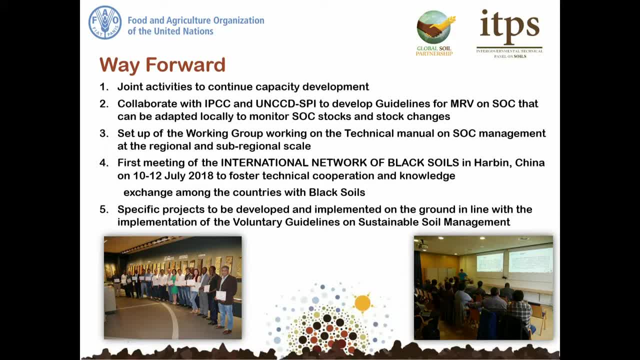 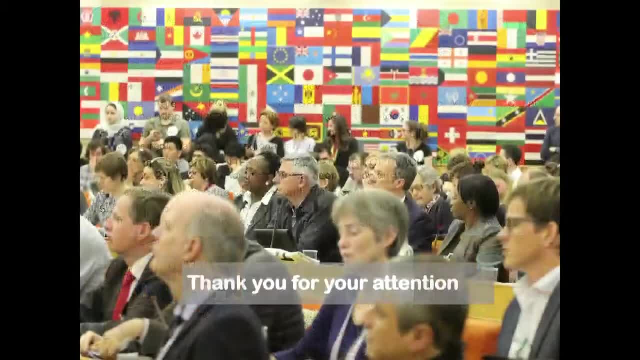 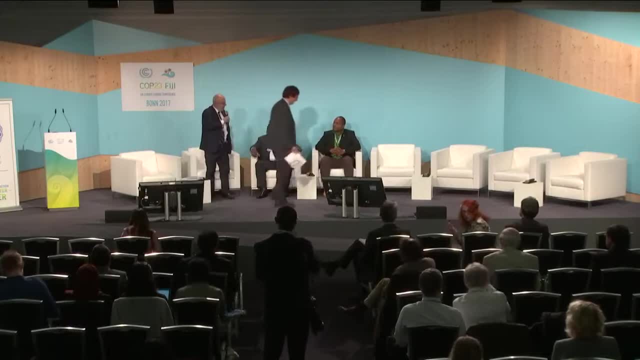 And then, of course, special projects that are ongoing in implementing this issue within the voluntary guidelines for sustainable soil management. Thank you for your attention. Thank you very much, Luca. Please don't go anywhere. Join us here. I would like to invite now Tekini. 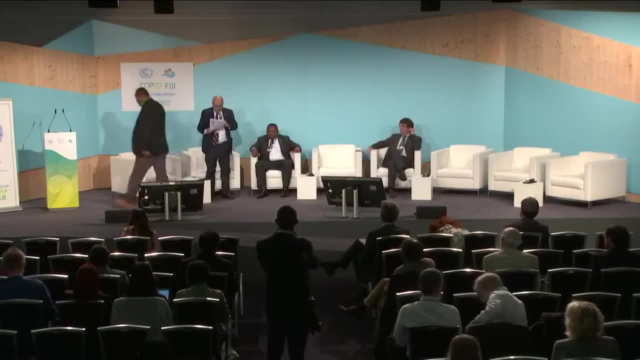 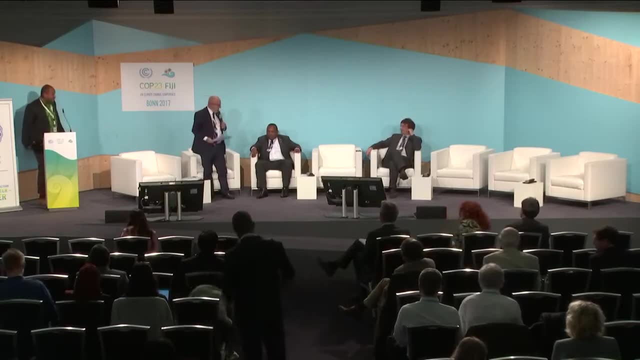 Mr Tekini Nakidakida works at the Ministry of Agriculture of Fiji. Your boss is here. I know it's a bit complicated when we have the boss present, but when we have a boss like Minister Enia, I think that thing is much easier. 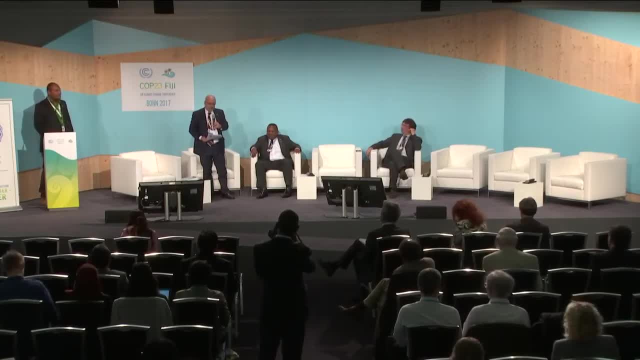 Tekini is from the research program of that And he's going to tell us about soil, organic carbon in the Pacific Islands. That would be a nice link with the global picture that Luca just presented. The floor is yours. Yeah, Thank you very much, colleagues. 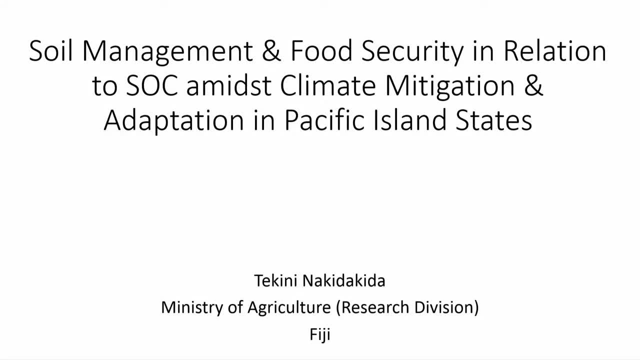 Honorable Minister and members of the agriculture family, As mentioned by our Minister this morning, that Fiji is in the forefront of climate change and mitigation and adaptation And for agriculture is very important. So I'm going to very briefly just say about some of the practices or way forward. 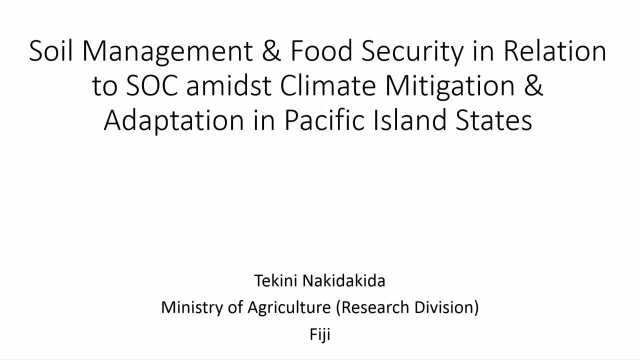 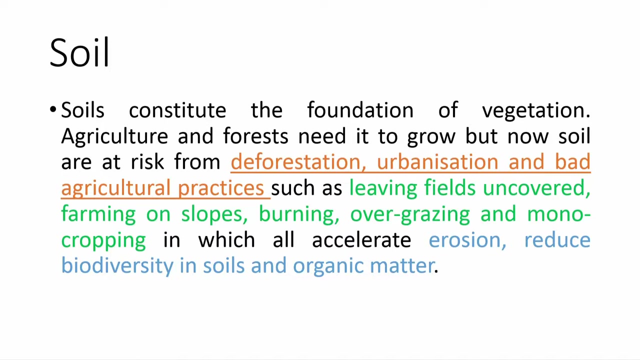 that we've been practicing in Fiji and also in some of the small island states in the Pacific. So sorry, I'm going to turn it over to Luca. Yeah, So all this while we've been trying to upskill our farmers, the members of our states, on why soil. 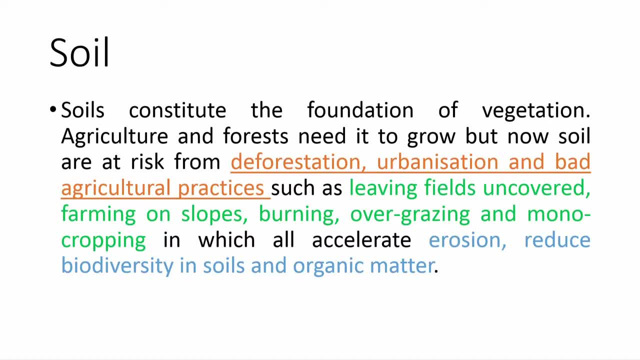 Because soil is the foundation of vegetation. Yeah, Deforestation, urbanization and most of the other practices- All of these accelerate erosion And altogether including the climate change effects of saline water intrusion. these are some of the factors that affect crop production and harm food security. 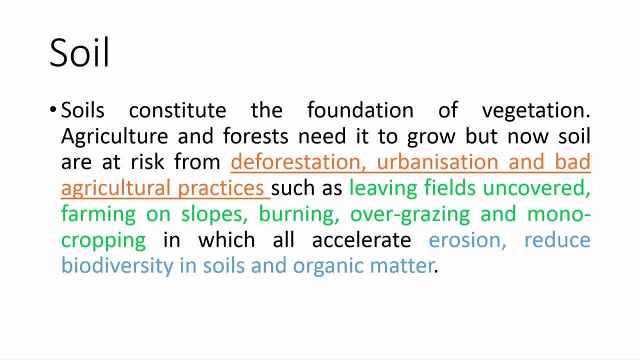 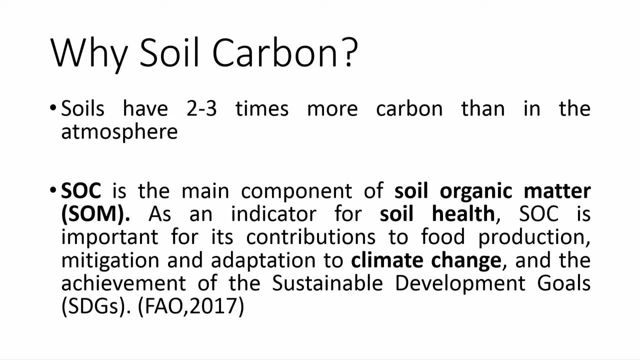 And all of these reduce the organic matter components in the soil. So why soil carbon is, as said by Ms Luca, is that soil has two to three times more carbon than that is in the atmosphere, And it is the main component of soil: organic matter. 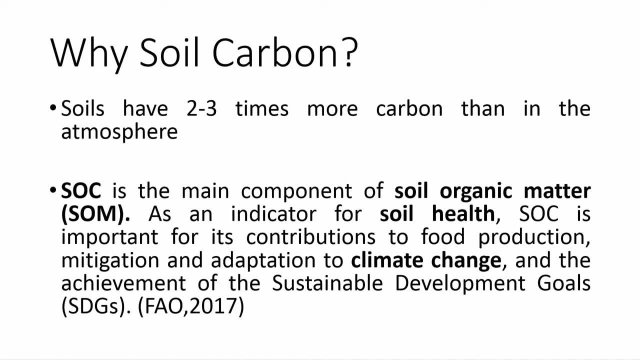 It indicates soil health, The color of the soil. that is what soil carbon does, And it contributes to food production, And in the Pacific we are mostly trying to adapt to the effects of carbon. That is some of the things that we are doing in order to achieve some of our sustainable development goals. 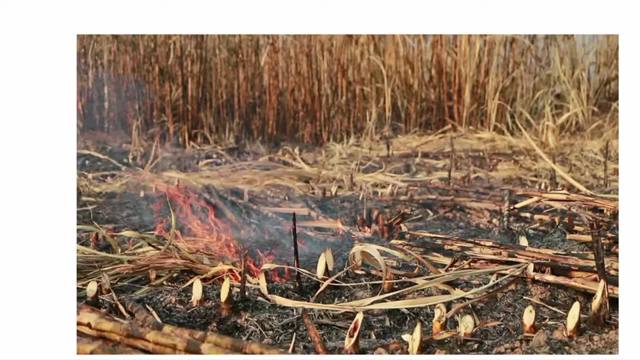 And some of the practices that we are trying to advise our farmers or our citizens of the Pacific Island states is to come away from previous management practices and try to change the way in order to improve soil carbon content in the soil, So burning off crop residue. 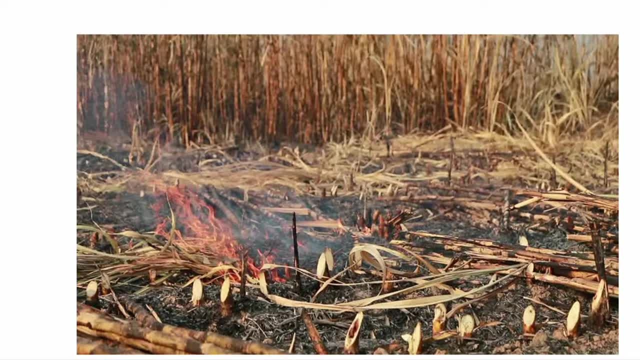 this has been the practice in sugarcane belts of Fiji And that is what we are trying to move away from in order to incorporate all those carbon into the soil. It is hard to change, But change should happen if we expect better results. 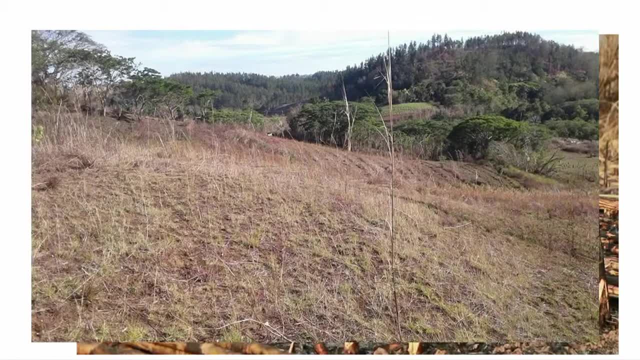 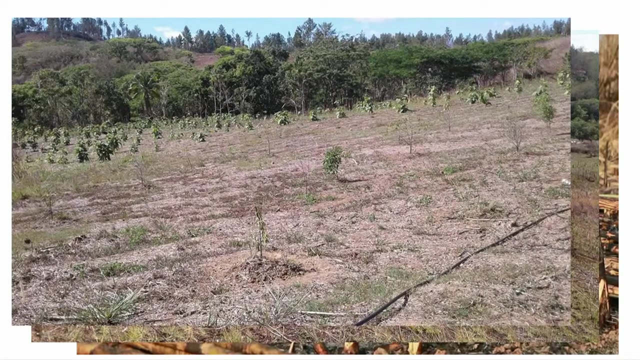 And these are some of the marginal lands or the dry zones that our minister has mentioned- has been experiencing months of dry spell. There is a group working on some afforestation in Fiji. Is that trying to adapt in these marginal or dry zones? they make heavy mulching on the trees. 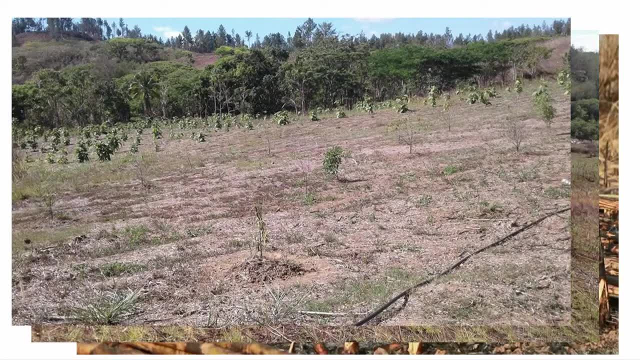 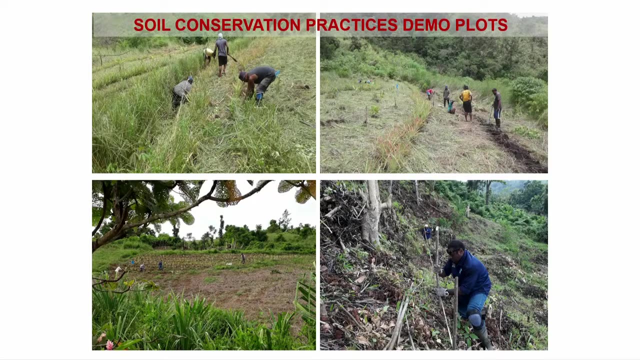 First is to reforest those marginal lands, and then agroforestry techniques will come in in order to ensure our food security for our local and smallholder farmers. So soil conservation methods has been practiced and taught to all our farmers, Irrespective of scale of farming. 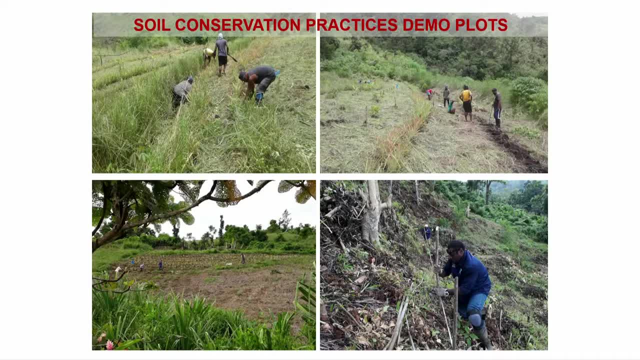 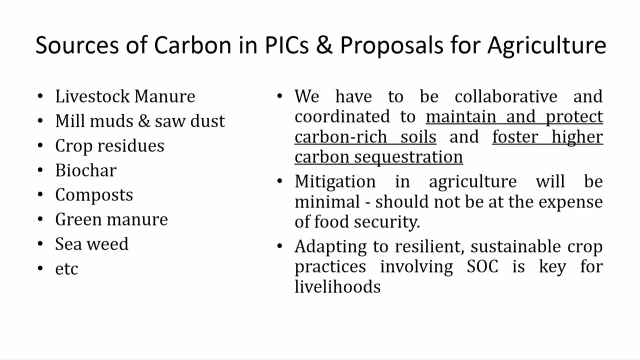 we always try to advise on how to incorporate carbon or sustainable methods of farming to the farmers in Fiji and the island states. So sources of carbon in our Pacific Island countries are mostly livestock, manure and compost and bio-car, etc. So we think that we have to be collaborative. 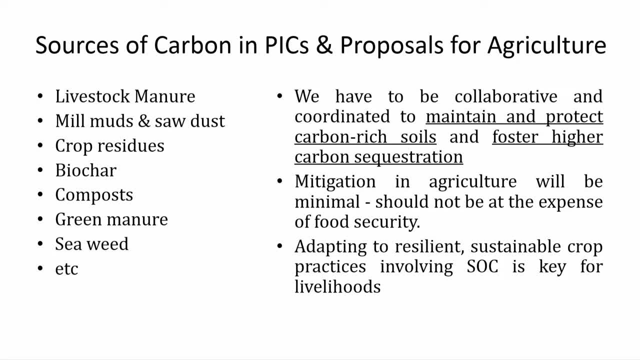 in order to have a maintained and carbon-rich soils foster the carbon sequestration. So, moving away from burning and slashing and try to incorporate all of those organic matters back into the soil. All of this we think it's imperative because it has to change the soil structure. 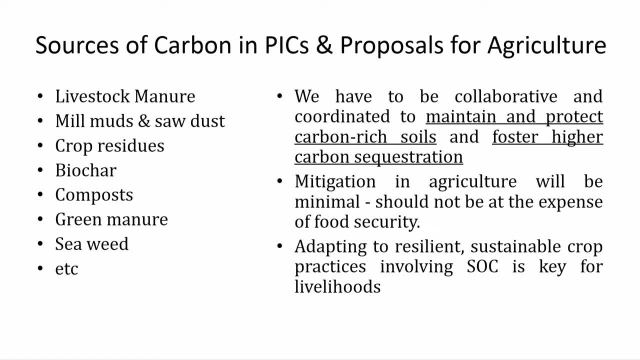 and improve root conditions. So adapting mitigation in agriculture will be minimal in our Pacific Islands because we are trying to focus more on adaptation, which is very, very important because mitigation will be for developed countries who have higher carbon emissions For the Pacific Islands. 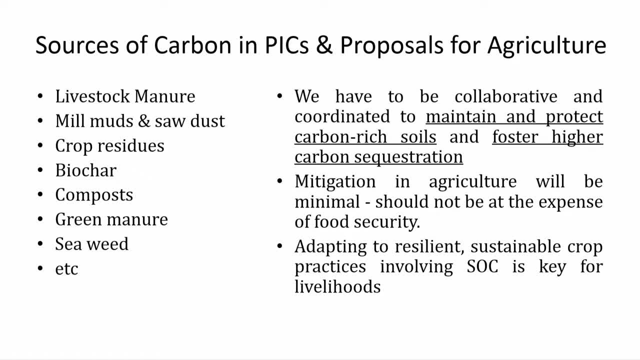 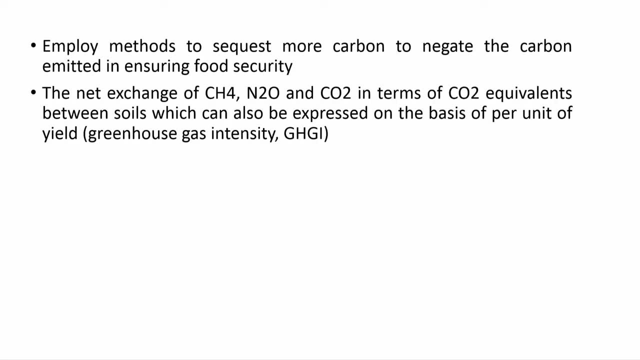 we try to adapt more and have a sustainable crop practice, which involves soil organic carbon, and incorporate more organic matter into the soil, So employing methods to sequest more carbon, and we're hoping that it will negate the carbon that is emitted when we try to ensure food security. 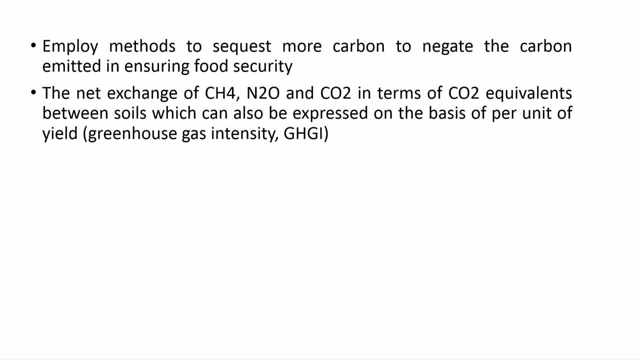 through the use of machineries and fertilizers. So the net exchange of all this methane, carbon dioxide, nitrous oxide, all this carbon exchange happening in the soils, it can be also expressed in terms of greenhouse gas intensity. So I think our colleagues from IPCC 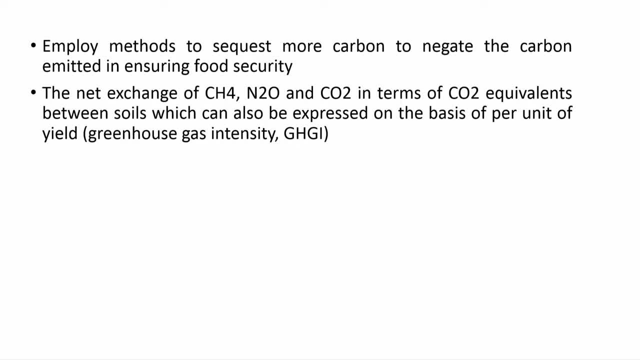 or scientists in the family. we can know that greenhouse gas intensity shows the intensity of the practice that we will employ. So greenhouse gas intensity, greenhouse gas emission, Basic mathematics will tell us that to reduce the intensity we have to increase the denominator. 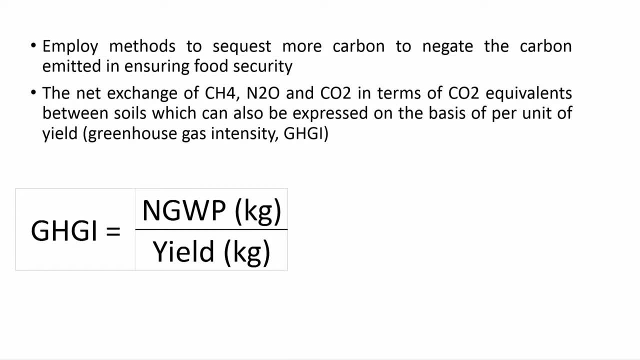 which is the yield. So that is why improving productivity in the Pacific Island countries in crops and animal production. this is key to reduce the intensity of greenhouse gas. So employing all methods of agricultural practice- sustainable, resilient and hoping that improving all this productivity. 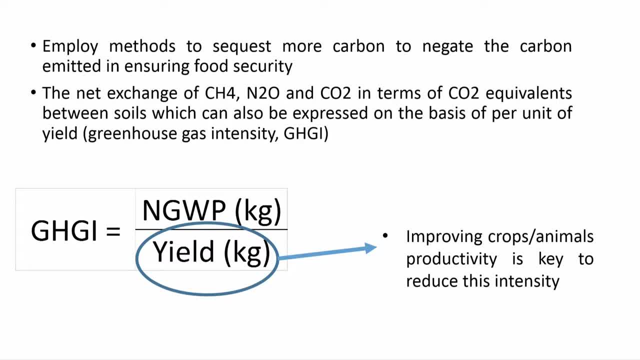 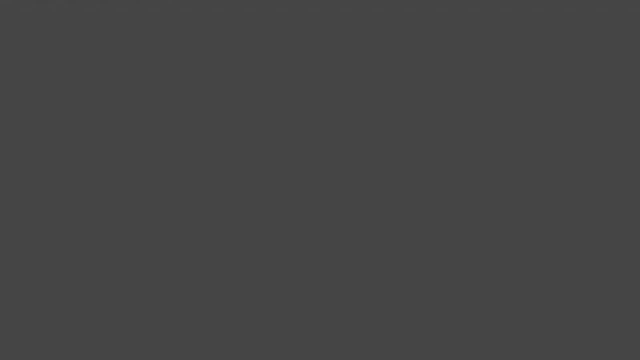 gradually or fast in these coming years. we hope that we will already be negating this carbon that we emit from our small island countries in the Pacific. Thank you very much. Thank you so much, Tekini. It's so interesting, really interesting, to see solutions coming up. 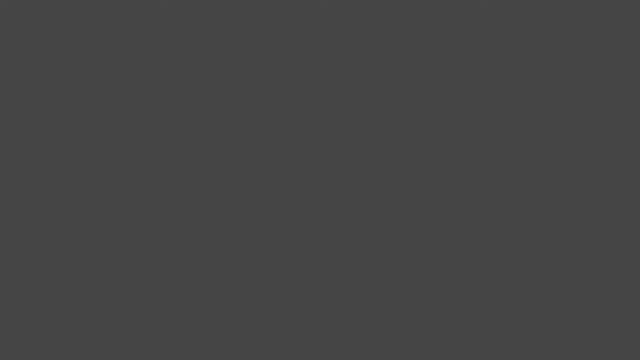 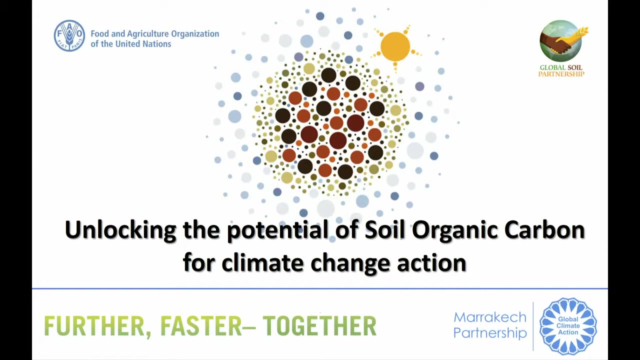 and to see that increasing productivity contributes to reducing emissions. And in agriculture, this is fundamental because we need to produce more with less. We need to produce more food with less water, with no deforestation. FAO, my director general, normally insists on the issue. 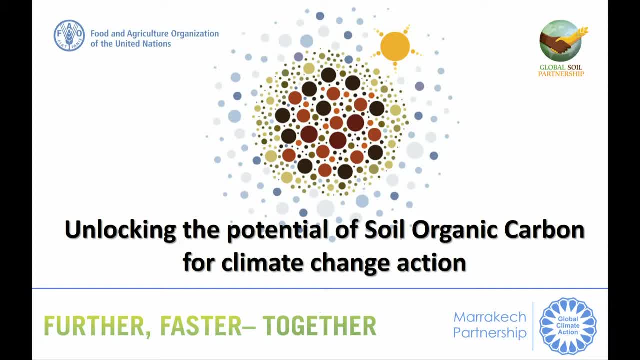 that we have to produce more food. We have to produce maybe 50, 60% more food by 2050, and we don't the year 2050, to cope with the increasing population. but we don't have to cut one more tree. 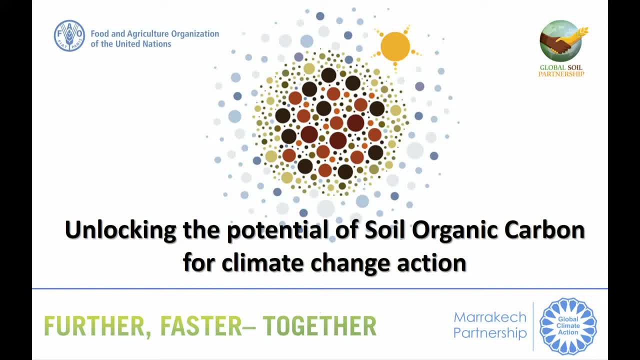 to produce this food And in the livestock session that just preceded us, we have about 30% reduction on emissions from the livestock area, which would be a lot related to increasing productivity. So thank you very much for us to see the solutions from these areas. 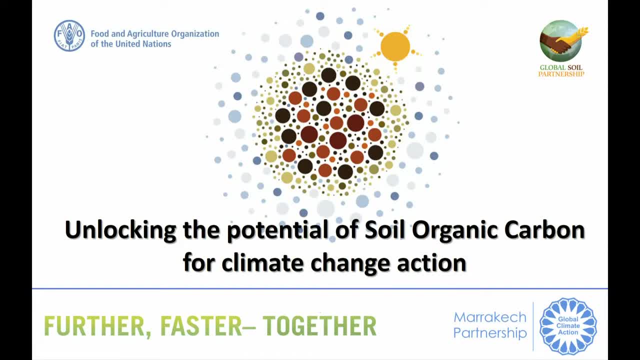 And now we would like to have a bit more of dynamism and have a panel, And I would like to invite the panelists to join us here. They would be Madame Jo House, from the Intergovernmental Panel on Climate Change, the IPCC. 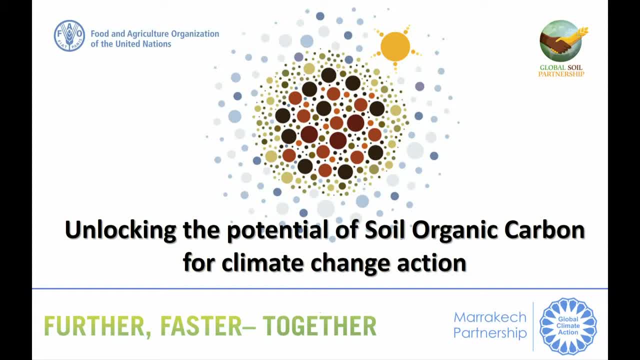 Jo, you are most welcome And maybe you want to escort Mr Minister here. Thank you very much, And I have my colleague from the World Meteorological Organization, the director of the research department, Dion Terblanche. Dion, you are most welcome. 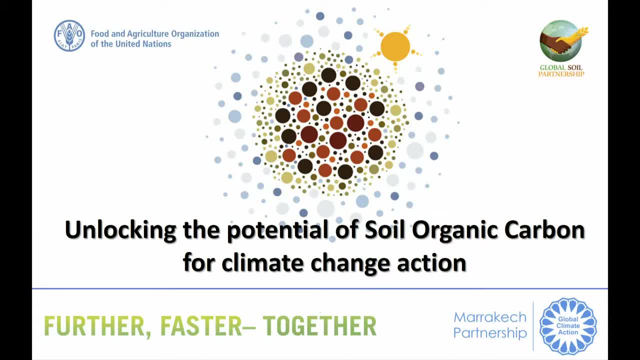 Yes, you may want to sit there. I would also like to invite Jean-Luc, Dr. Jean-Luc Chotté. Am I pronouncing Chotté Chotté? okay, A good friend from the. he's really representing the scientific body. 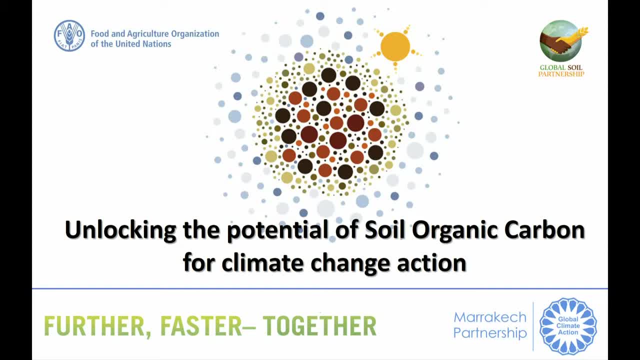 of the United Nations Convention on Combat and Desertification And I cannot recognize Josiane. She's not coming right, Luca. Luca is a good representative of the European Commission with us. Josiane was invited. Unfortunately she couldn't make for today here in Bonn. 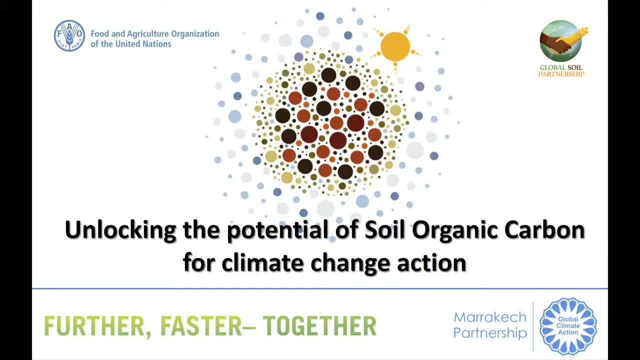 I think we have an excellent panel to move ahead with us with some interesting questions, And I think I will first ask each panelist to introduce yourself more properly Why you're interested in soil, organic carbon and especially the three colleagues. that joins us here. 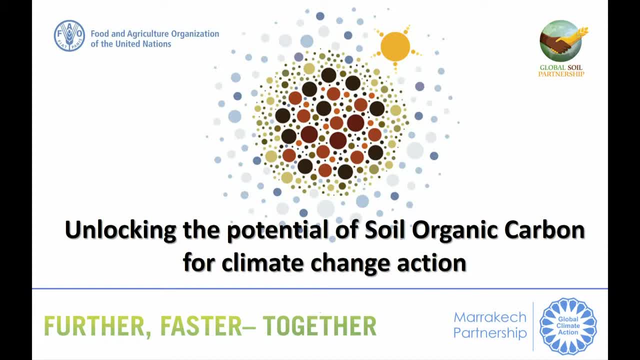 And who are you and how long have you been working on this? But do it in one minute for us to gain the time while I get the questions that my colleagues in Rome sent to you, and they are tough, So I have to make them properly. 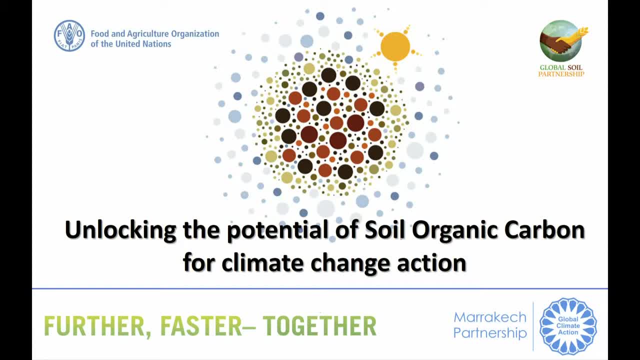 Hi everyone, Thanks for coming today. My name is Jo House and thanks for the really good talks. already I work at the University of Bristol on land and climate interactions. I'm also IPCC lead author since the third assessment report through to the fifth one on working groups one, two and three. 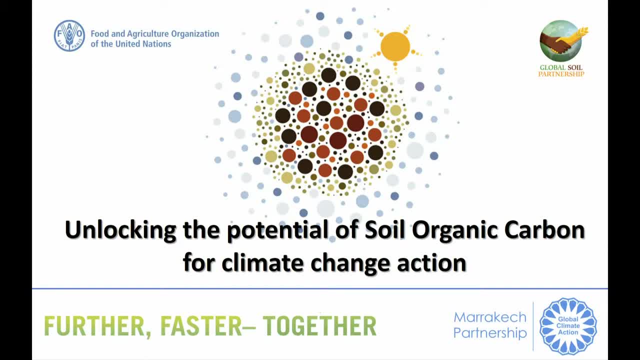 And I work on the methods report side And I'm currently lead author on the 2019 update to the 2006 guidelines on greenhouse gas inventory methods and on the special report on climate change and land, And I've also worked in government for a while in the UK. 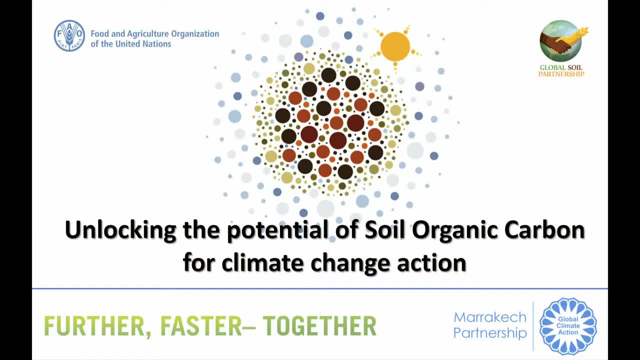 Do you want me to just say something briefly about that? Yeah, So IPCC update. So that would be a bit informative. Everybody we share, every two of us share, one mic We have. most of us are informed, very well informed, about IPCC. 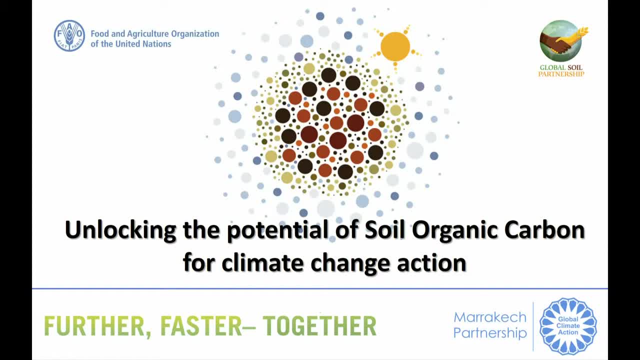 but not everyone. It's so interesting to know why the scientific body is interested in what you're doing, So it would be nice to know about IPCC and its process, please. So soils are really central to a lot of what we do in IPCC. 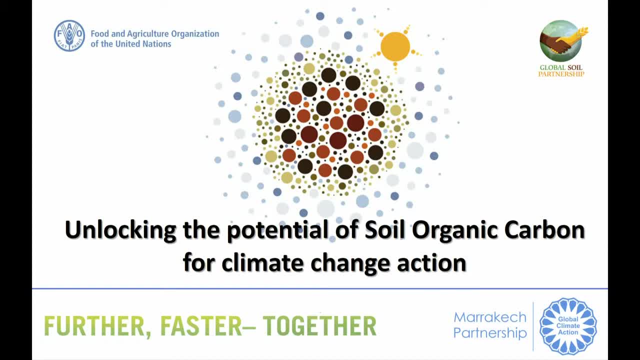 In the assessment reports we're obviously assessing the science and that includes information on emissions from the soil and impact of climate change on soils. I mentioned about the inventory work. There's a whole methodology on doing your greenhouse gas inventories. that includes very specific methods on both organic soils and mineral soils. 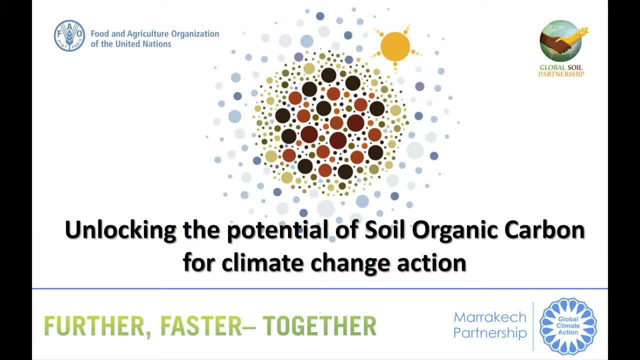 And we're currently updating the 2006 guidelines to include things like the new information on carbon stocks, new guidance on methodologies and some more elaborations of the more complex methodologies that come in three tiers, And that update will be published in 2019,. 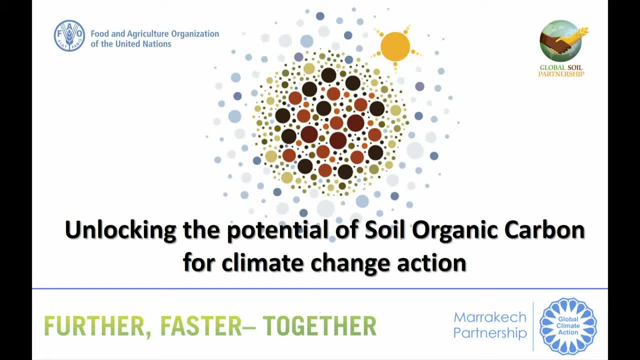 or the refinement, will be published in May 2019.. We're also doing three special reports at the moment in response to government requests: one on 1.5 degrees, one on oceans and cryosphere and one on the land. And the one on the land. we have chapters on desertification. 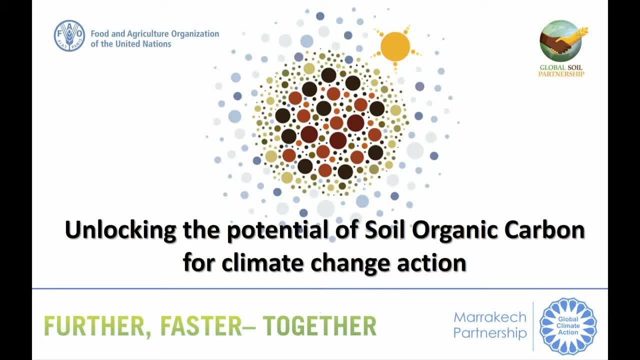 degradation, greenhouse gas flux, and they'll all include a large element of soils- both impacts on soils and mitigation- And there's also a chapter on synergies and trade-offs which will touch on some of the co-benefits of soil-based mitigation. 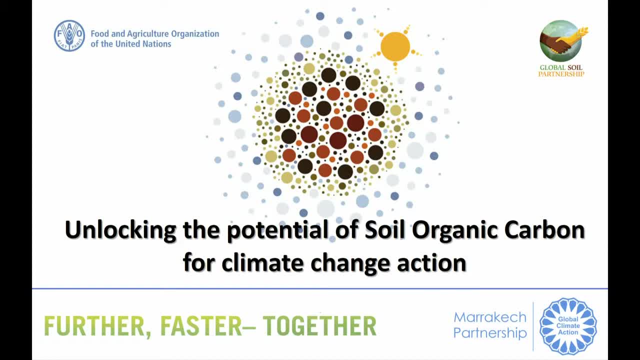 And that's due to come out in September 2019.. Thank you, Dion. would you like to introduce yourself Now? I think we know more of the process and we are so happy to contribute to the IPCC process. Dion from the World Meteorological Organization. 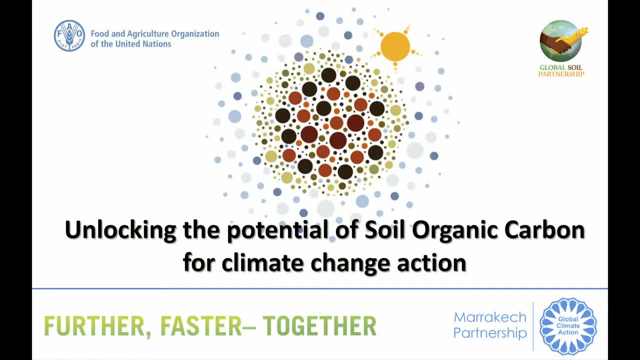 and the Research Department. we have a little bit that you lead. Can you tell us Sure? The World Meteorological Organization is one of the specialized agencies of the United Nations. Just a little bit closer to your mouth, Can you hear me Sure? 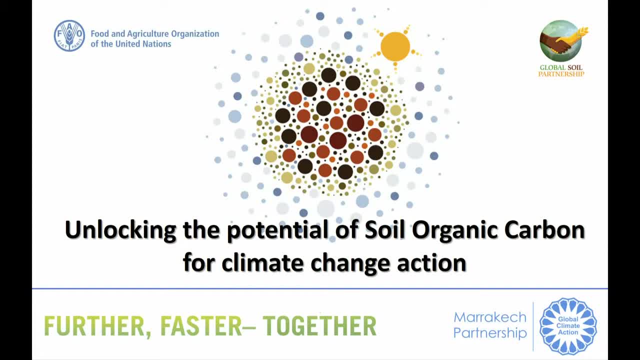 Okay, so the World Meteorological Organization is one of the specialized agencies of the United Nations, and its mandate covers the elements of weather, climate, water and related environmental issues, including the composition of the atmosphere. I head the research department, and so I oversee the work of the World Climate Research Program. 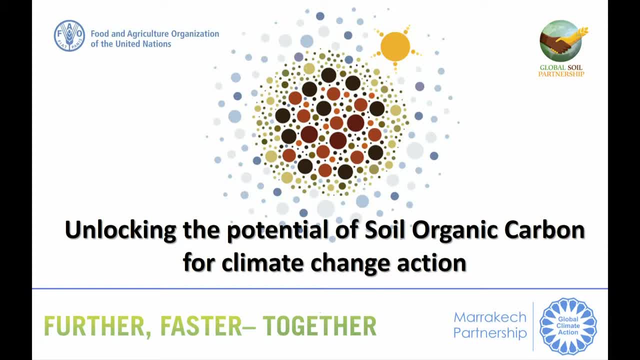 that feeds directly into the IPCC, but also the Global Atmosphere Watch, which is the program that does harmonized measurements of atmospheric composition, including greenhouse gases, around the world, and the World Weather Research Program. So the interest in this topic, of course. 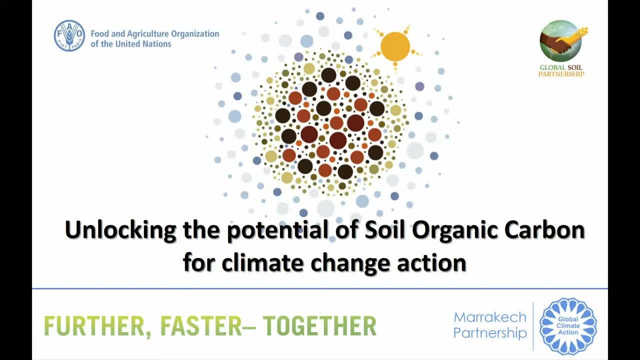 is that this is one of the uncertainties in the modeling efforts, including the issues related to permafrost, and that is why WMO has decided to properly engage in this matter, so that we can refine the models, improve the observations and do a better job at covering this very important aspect. 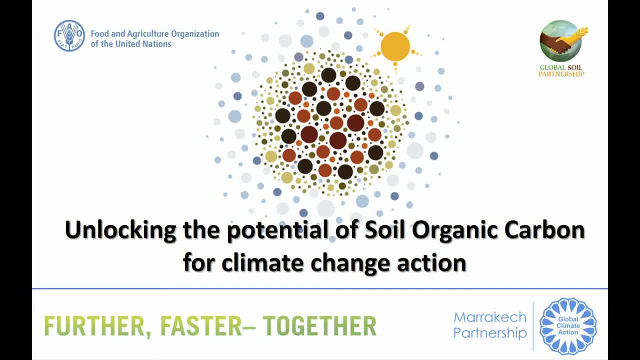 Yes, thank you. First of all, I would like to thank FAO to have invited UNCCDSPI to be on the panel, And just a few words in my personal opinion. I did my PhD on carbon dynamics in French soil and after that I got a position through IRD. 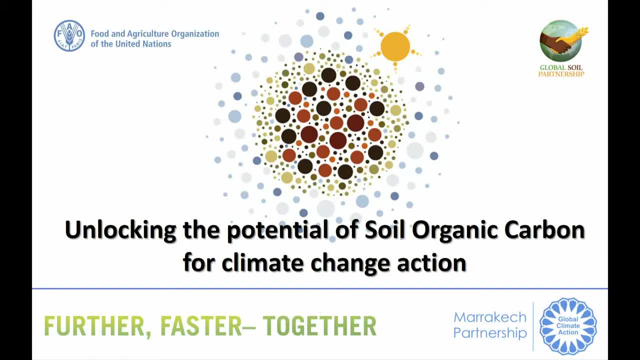 and I spent almost 20 years in West African countries- And when you go on the ground, when you see farmers looking for organic carbon and when you see the effect of organic carbon on maintaining soil fertility and improving productivity, that is why I have always been working on organic carbon. 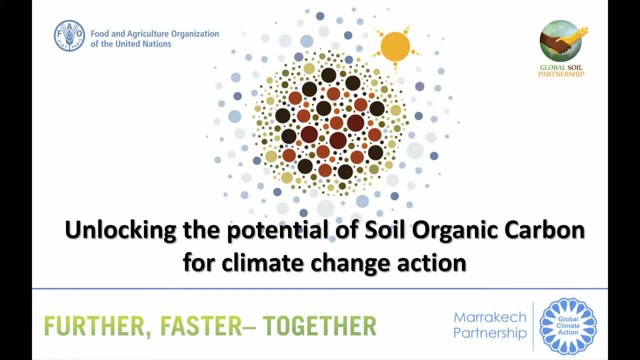 And it is why- because UNCCD is dealing with, you know, land degradation and desertification- I just joined the SPI group. SPI group is a group of 20 experts, 10 mandated by parties, 10,, you know, selected because of their scientific background. 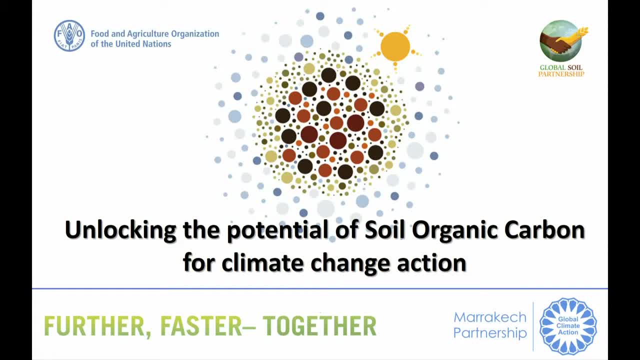 And the very innovative issue is that on the same group you have representative of parties and research and scientific, And there is also three seats for observer. And land degradation neutrality has been, you know, a huge project run by UNCCD SPI. 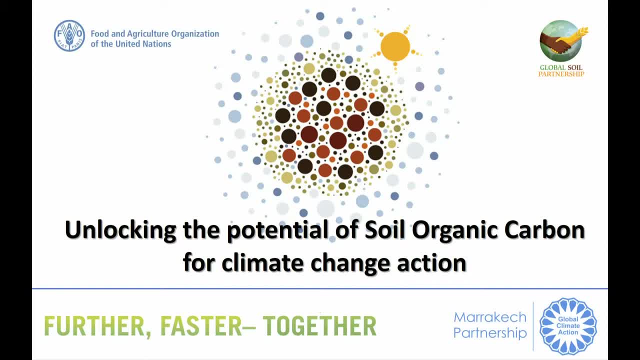 And it has been adopted during the COP 13 in Ordos, And one of the metrics of land degradation neutrality is soil carbon stock. So here we are. Thank you very much. Thank you. So you are now informed about the level we have here. 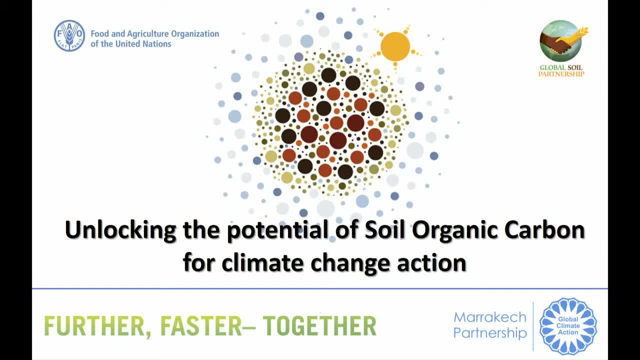 And it is very high. I am very happy. Before I start putting the questions, we have about 54 minutes to go. The watch there are very helpful to tell us to go if we use the time that has been allocated to us for this session. 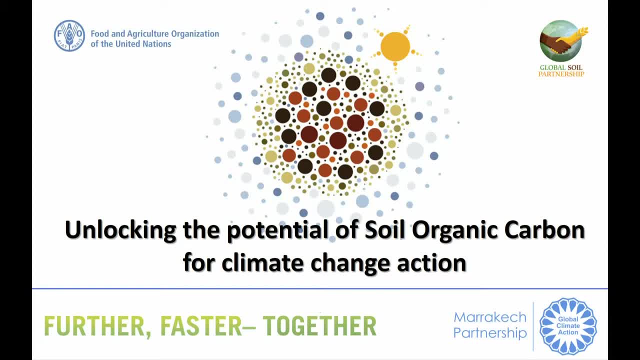 I would like to say that the evolution of the science behind this is very important, but we have to put it in a language that non-scientists can understand, So I will have a surprise. in the end. I will ask for someone that is not a scientist. 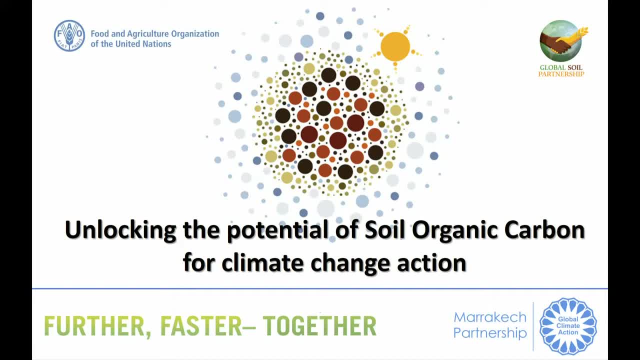 to talk to us and see what he or she has learned about this session, And I am talking about a colleague that we invited today to join us, Terran Giacomini. She is from the. I have to have the right name, Terran. you may want to introduce yourself too. 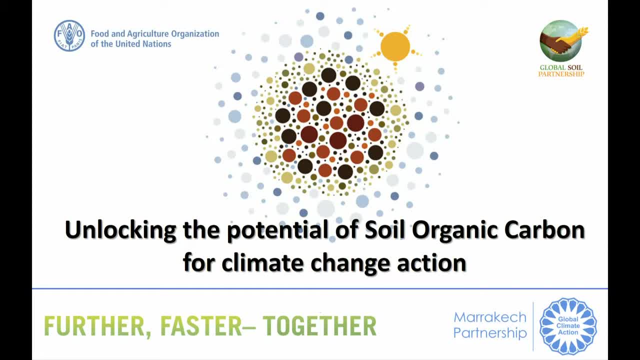 Hi, Where do you want me to sit Over there? But I need the mic. Oh, you need that one. It is one for two. There is a mic there. Okay, Terran will introduce herself and tell us. We catch her here to try to translate the language. 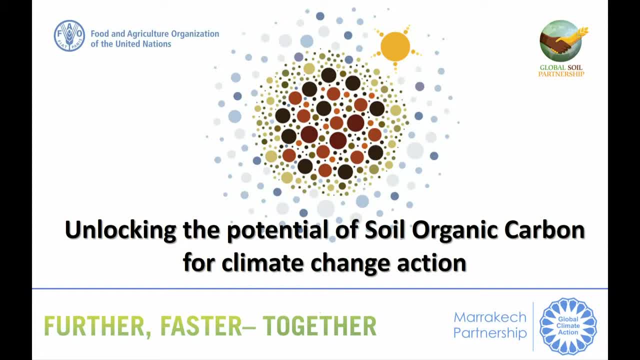 that we are discussing into how we understand this. You gave me exactly your affiliation, but maybe you want to repeat. I can clarify that. Yes, So my name is Terran Giacomini. I am from the National Farmers Union in Canada. 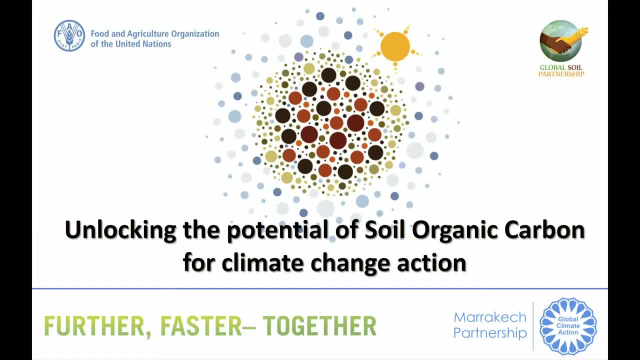 which is an organization of farmers from across commodity sectors and of different scales, And we are a member of the global peasant movement, La Via Campesina, which many of you have probably heard about. So you want me to provide some reflections on what we have heard so far. 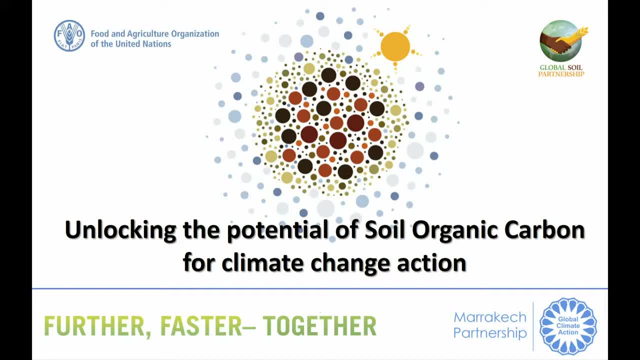 Yes, At the end. I want you to help me take notes and look from your perspective, from the Farmers Association in Canada and Via Campesina in general, how soil, organic carbon and climate reflect or what you think that we can contribute to this. 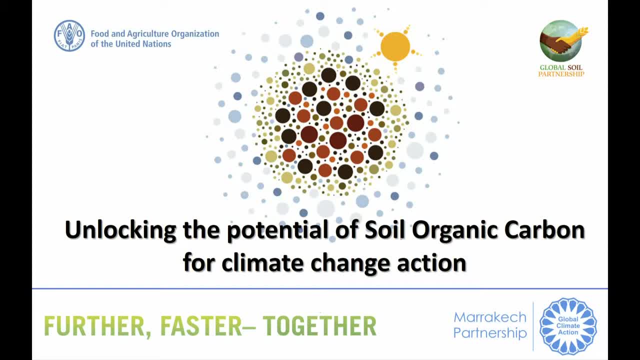 So if you help me with that, it would be at the end of the session. I can help you with that. Thank you very much. So I would start with you, Jo, And that also improves a bit the gender balance in this panel, which was pretty bad, I have to say. 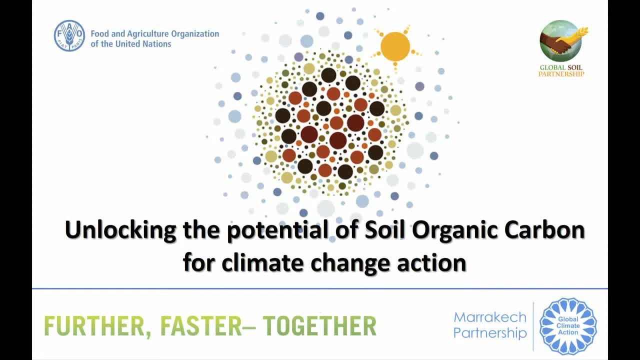 although very well represented by the two ladies that are joining us now here. IPCC: I will put two questions. My colleagues asked me to put two questions to you. IPCC started a new cycle. you explained to us. you have the assessment report coming up in 2019.. 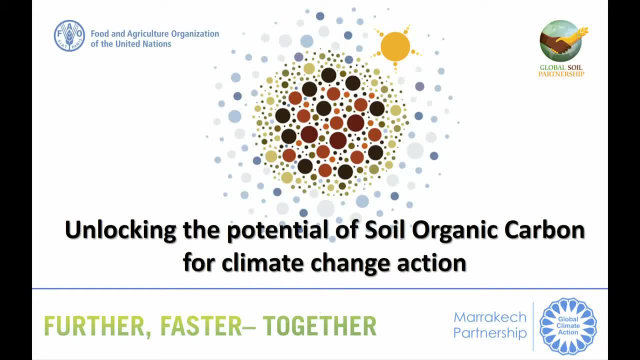 Why is an updated IPCC guidelines on monitoring soil organic carbon stocks and soil organic carbon changes necessary? What's the relationship of this and the recommendations that came on the global symposium that we organized earlier this year? we run together with IPCC, SPI and the World Meteorological Organization. 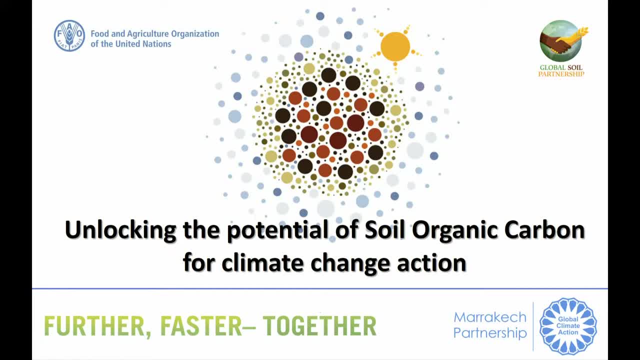 And also in that symposium the chair of IPCC, the secretary, Mr Moksit. he raised the issue that one of the main gaps identified in the fifth assessment report was missing globally harmonized and standardized data on soils. So how can the link to the efforts achieved 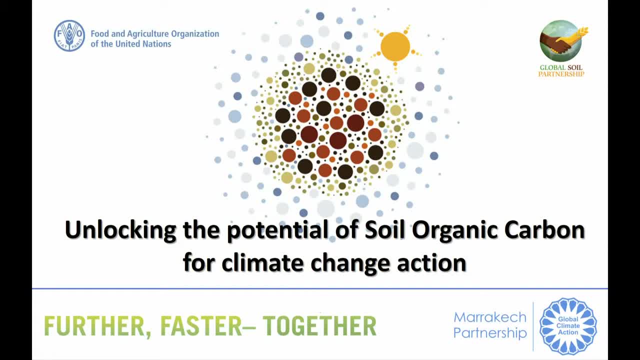 and to be further developed within this network- international network of national soil information institutions, the Global Soil Partnership and the Global Soil Organic Carbon that Luca just referred to us would contribute to this general effort of improving soil organic carbon data. Thank you, Eduardo. 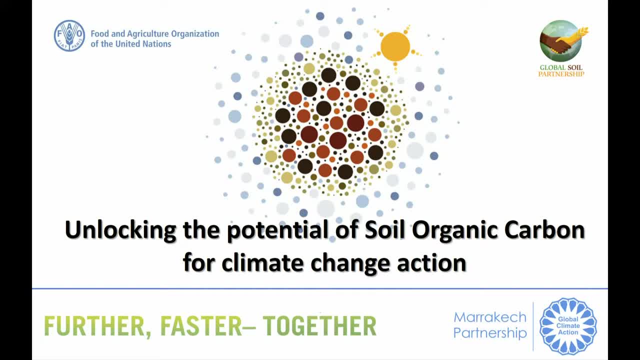 and to whoever asked the questions. So first just to clarify: the assessment report, which will be the sixth assessment report, is different from the methods update and the special reports. So the sixth assessment report cycle is just beginning and that won't be done until 2019.. 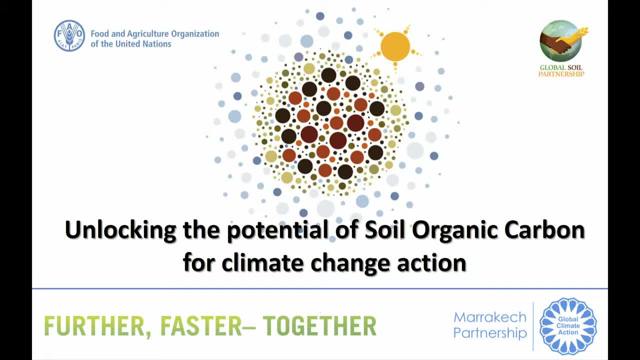 It will be done until 2022.. The methods report, which I think is what the questioner really wants to know about, is to update the 2006 guidelines, because 2006 was quite a while ago and since then there's been lots of new information. 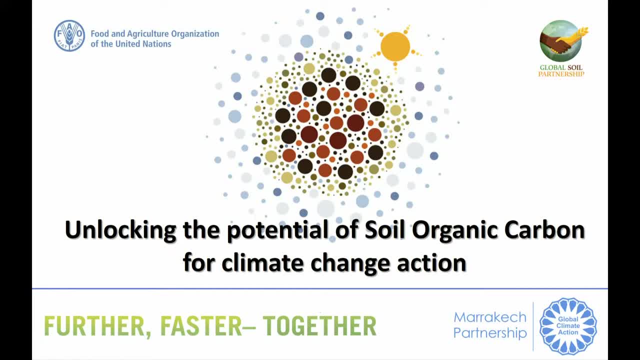 And so the particular needs were identified, scoped with governments and with scientists, So particularly things like information on soil carbon stocks and on changes in soil carbon stocks to provide updates to the emissions factors database that countries use, and then some new guidelines on the methodologies. 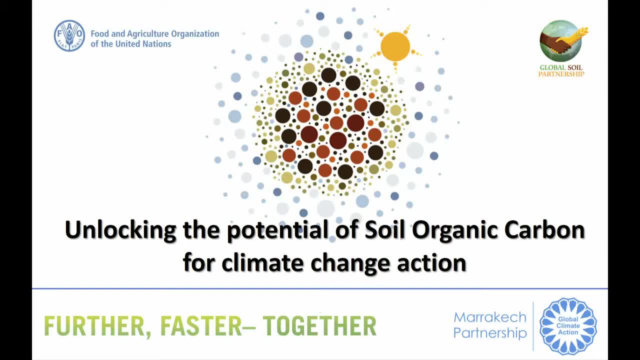 that countries might use for modelling or incorporating newer soil models and more country-specific data, And so there's a need for this update, really because they're the good practice guidance and good practice guidelines and good practice that countries are using the best available scientific knowledge. 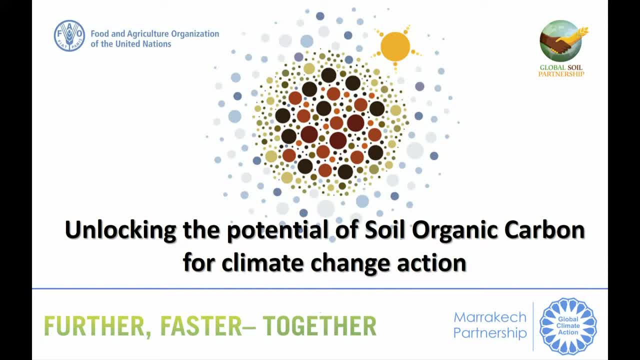 And in relation to things like the soil map that was being developed that Luca talked about, and also the ISRIC soil product. So there's conversations going on between IPCC and ITP and ISRIC and others to see how useful those products might be to us. 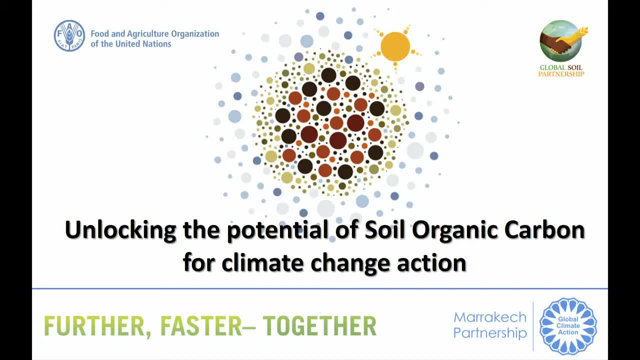 and if there's a need to develop new products. IPCC doesn't do science, but we assess the availability of available science and we assess what's helpful in the methods And definitely where there are available maps like this and for countries that lack country-specific data. 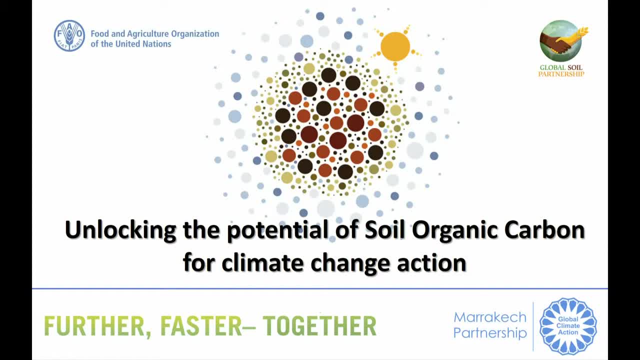 these kind of products can be extremely useful. Thank you, Thank you so much. Thank you for bringing light on this, Your Excellency. My pleasure It's not only. we are very honored to have the presence of the Minister of Agriculture of Fiji. 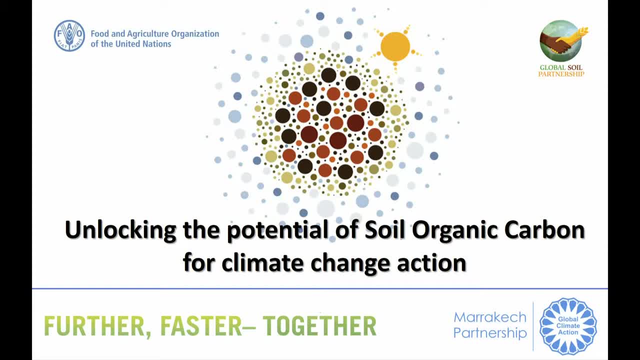 but it's not only because we have the space here. I would like to make sure that we have the other panelists who are waiting. Mr Nazir Fuad, are you in the room? Can I see you? Yes, Nazir, would you be able to join us in the panel? 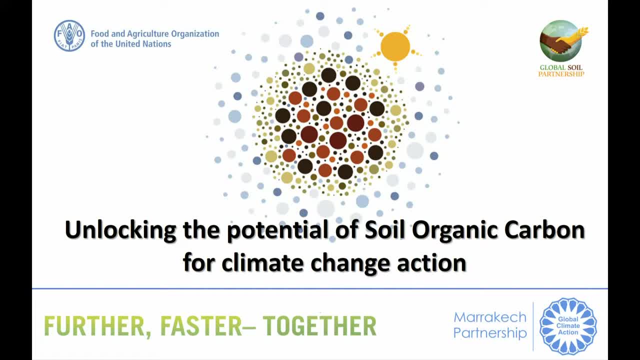 Nazir is from the Pitland Restoration Agents of Indonesia and we all know how important it is to have the Pitland perspectives on this. So if you could take the seat, please- and maybe Yes- in the middle And maybe you can introduce yourself as 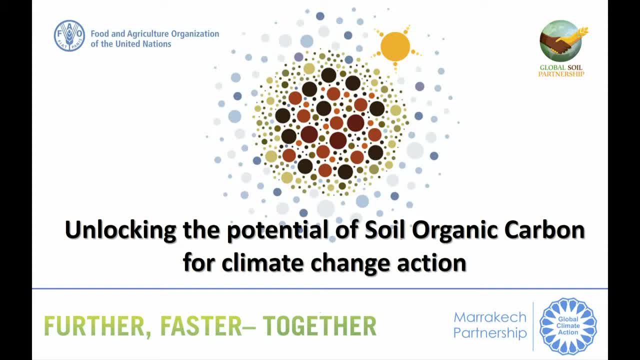 Sorry that I jumped immediately on you, but as the others have already introduced themselves, can you please do so? And why the interest on this? I mean, Pitland says everything, but you may want to say exactly about the work of the Pitland Restoration Agents of Indonesia. 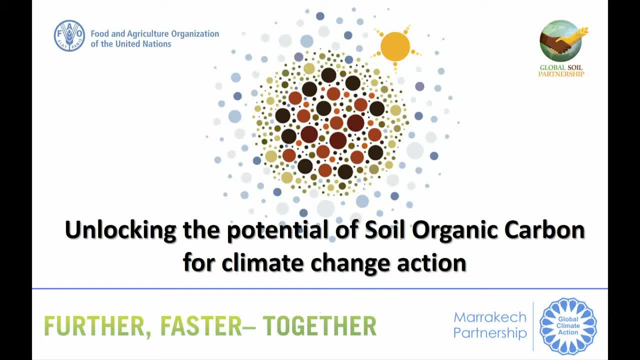 Yeah, hello. Thank you for the invitation. I am Nazir Fuad, head of the Pitland Restoration Agency. This is a new agency set up by the President of Indonesia. report directly to the President, As Indonesia has the largest tropical pitland in the world. 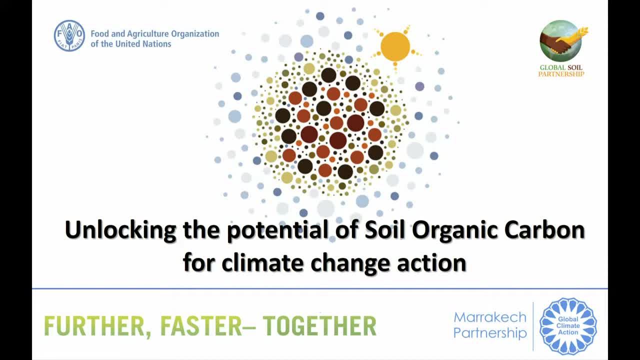 but also about half of our pitland is degraded and some are badly drained and causing a lot of problems, including fires. the President instruct us that Indonesian pitland has to be protected and restore part of the area. restore part of the area can be used. 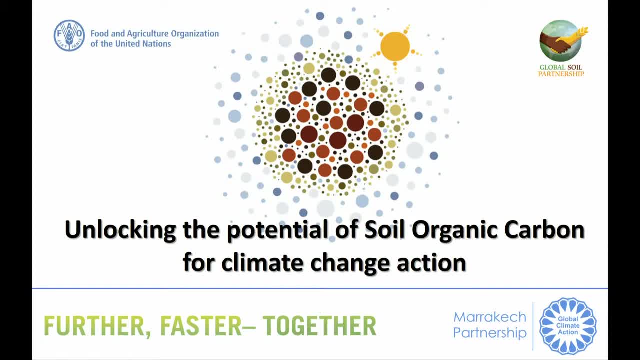 for agriculture or other purposes. Thank you, Thank you very much. I'll come back to questions to you in the end. because it's such a specific aspect, I would like to go broader to my colleague at the World Meteorological Organization, Dion. 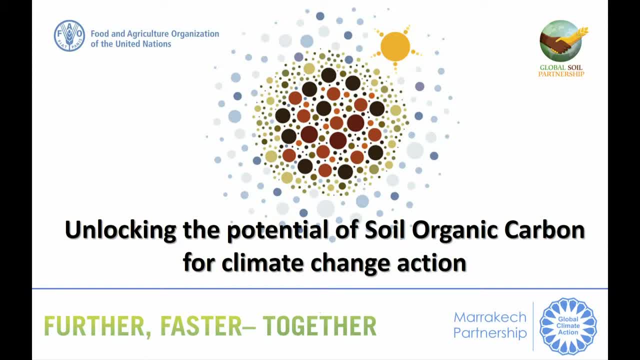 How is the soil organic carbon preservation and sequestration and its interaction with climate predictions addressed at the work that you are doing in the research department at the WMO? Is the preservation of the largest soil organic carbon stocks, such as under permafrost, realistic and feasible? 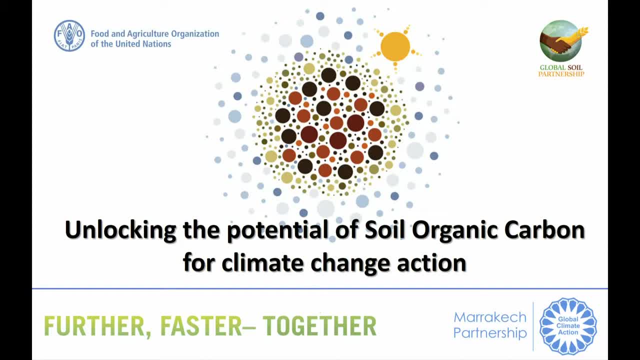 under the climate change scenarios. Would you like to come up with those ones? Sure, thank you. Those are very good questions and very relevant ones. Before we get into answering them, I just want to remind everybody again that the World Meteorological Organization 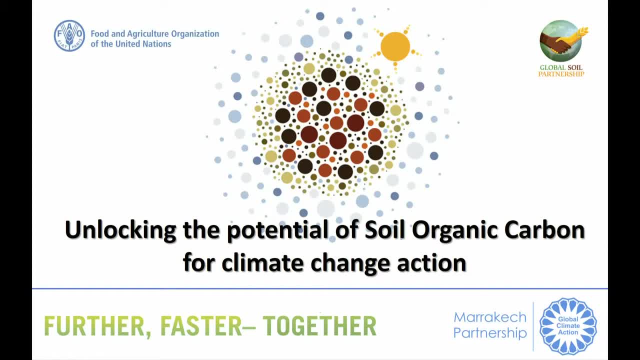 every year issues the greenhouse gas bulletin, and the greenhouse gas bulletin every year is launched by WMO and that was done just more than a week ago, And we saw for 2016 an increase of 3.3 parts per million in the global greenhouse gas concentrations related to CO2,. 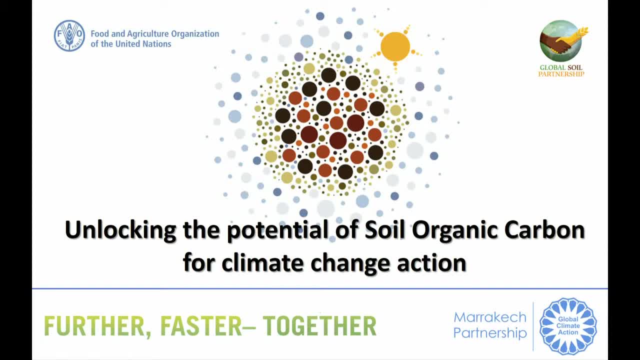 which is the largest increase on record. So we are actually lucky that the environment and nature is good, because the oceans and the terrestrial biosphere absorbs about half of the emissions that we put into the atmosphere, but it's what stays behind in the atmosphere that really drives climate. 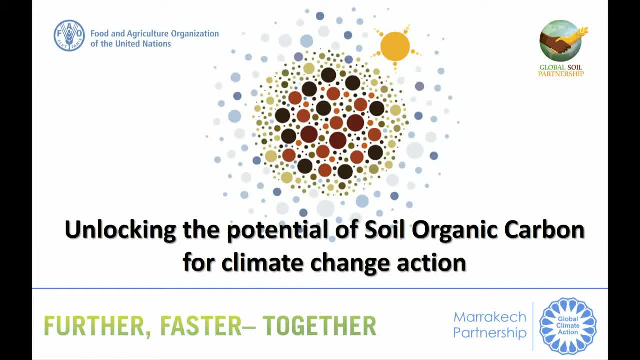 and impacts on the oceans and the environment in general. So, with this as background, it is quite important that we understand the carbon cycle much better And, as we have heard, the soils of the world plays a very important role in this and contains very large stocks of this. 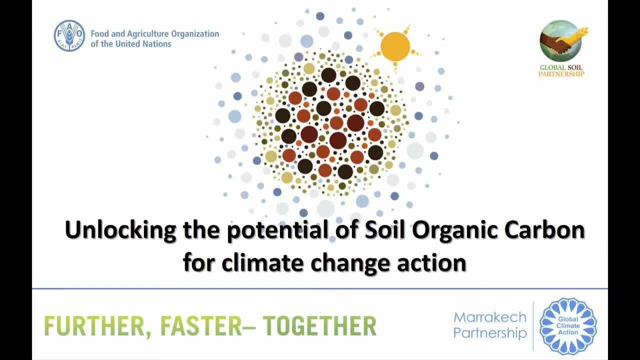 So, if you just think about, the first meter of soil in the world stores about twice as much carbon than we have in the atmosphere. So any changes there will have dramatic impacts on the world, as we know. So this is the baseline. So WMO engaged in this whole issue. 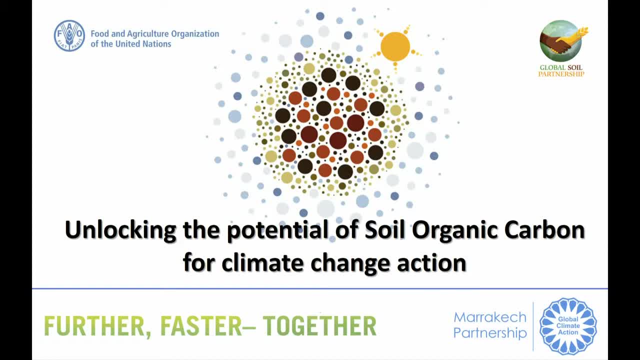 by being a co-sponsor of the Global Symposium on Soil Organic Carbon that was mentioned already earlier, And from the recommendations that we saw, we thought that the two that we would really engage in is on recommendation two and three. Two is on the issue of the guidelines for measuring. 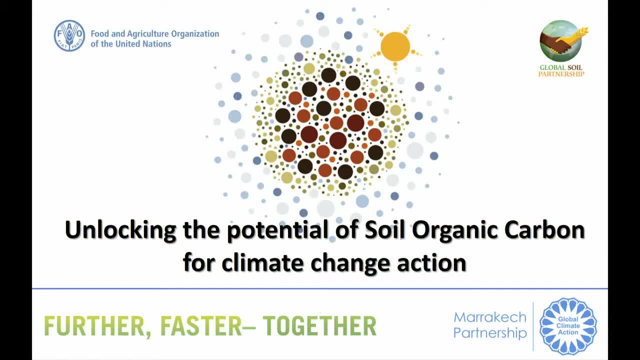 mapping, monitoring and related to the global soil organic carbon map, which is also, then, a very important input into the modeling work that will be done by WCRP and then eventually being assessed by IPCC. So we complete the cycle in such a way. 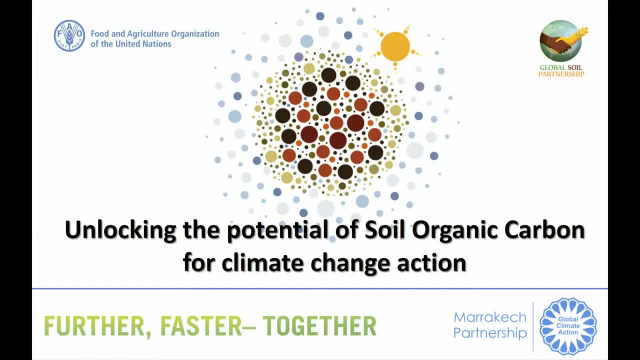 But also in terms of recommendation three, which regards, which is related to the interactions between carbon and nitrogen, because in the Global Atmosphere Watch, we have the global standards of how you go about to measure the gaseous phases of these compounds, And so we can also bring something to the table. 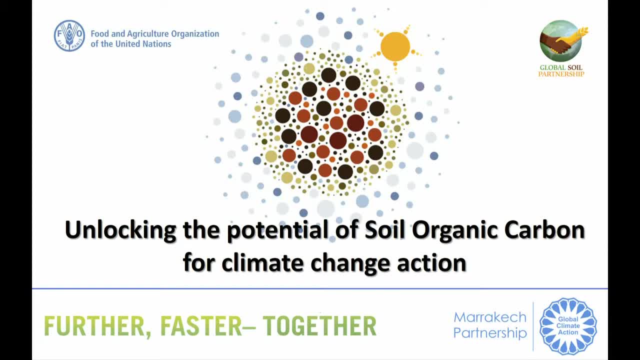 in terms of best practices on measurement techniques. The Global Atmosphere Watch is also launching a system that is being discussed in COP as well and that is called the Integrated Global Greenhouse Gas Information System, because we have now moved beyond the state of just using observations to understand better. 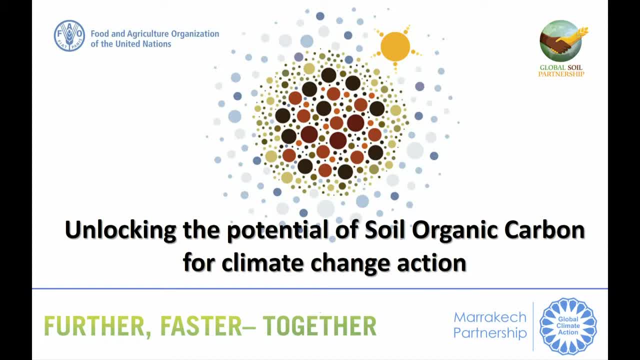 If we combine observations and modeling, as we do in reanalysis, to get a better idea of what the high-resolution past looked like, we can also do the same when it comes to the greenhouse gases, And this integrated global greenhouse gas information combines high-accuracy measurements in the atmosphere. 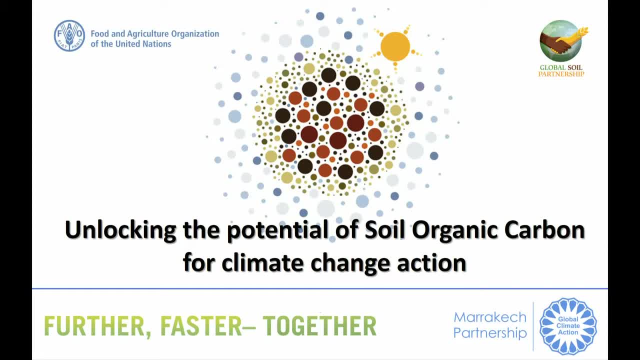 with inverse modeling, so that you can have an additional source of information And it's scalable. You can take it down to small areas and you can actually don't want to use the word verify, but you can add value and reduce the uncertainty on the emissions. 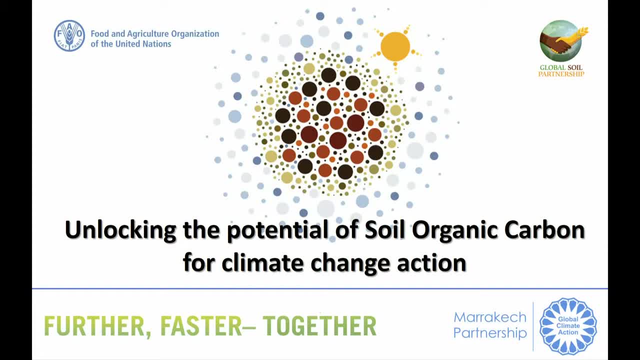 Because I think it's extremely important that our actions be measured where it matters- And to me it really matters- in the atmosphere and it's quite clear where it matters there, because that's where the radiator forcing for the climate system happens And that is where the whole chain reaction is set off. 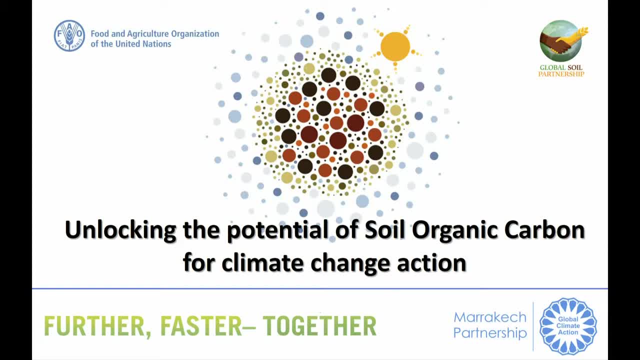 So if we do something on the terrestrial biosphere, on the way we treat our soils, we must be able to follow that through in measurements of the impact on the atmosphere, And with this system, which is scalable, you can then verify some of these issues. 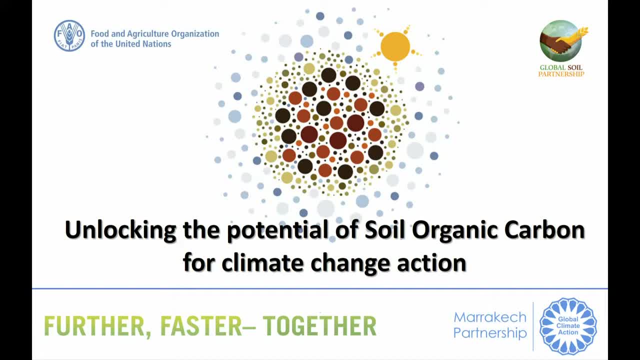 But of course, WMO is also a co-sponsor of the World Climate Research Program, as I mentioned, And there are several initiatives in the world like the World Climate Research Program that addresses soil, organic carbon and its interaction with the Earth system In terms of CLIC. 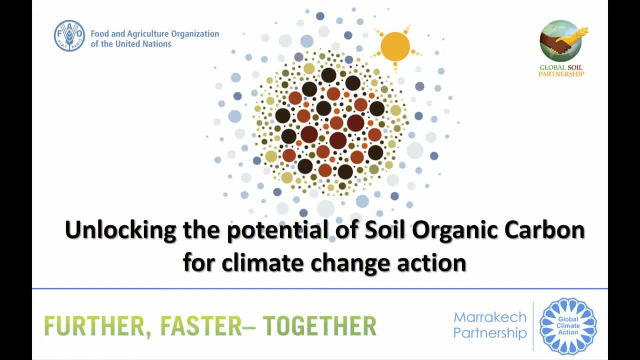 it's one of the core projects of WCRP. It deals with the icy parts of the world and, of course, it is also a partner of the International Permafrost Association. So in terms of permafrost, we store about four times as much carbon. 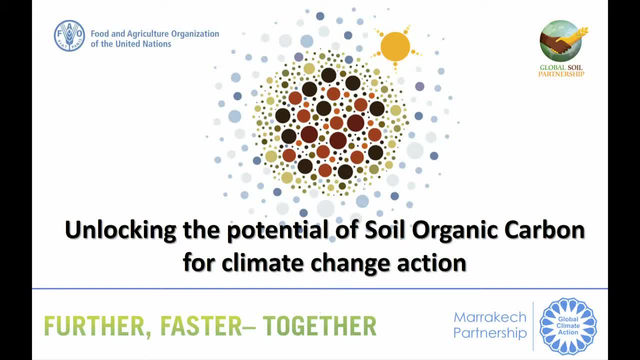 as mankind has ever released into the atmosphere in the permafrost. So it is extremely important and there's a lot of uncertainty still around that It needs to be better treated in the next cycle of the IPCC, and WCRP is working towards dealing with that in a much better way. 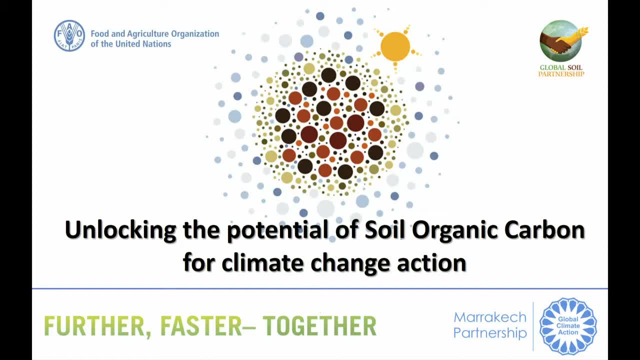 So if you just think about four times as much as we have already released in the atmosphere, any instabilities in the permafrost of the world can really have positive feedback and tremendous chain reactions that will put us in real danger. So this understanding of the carbon cycle, 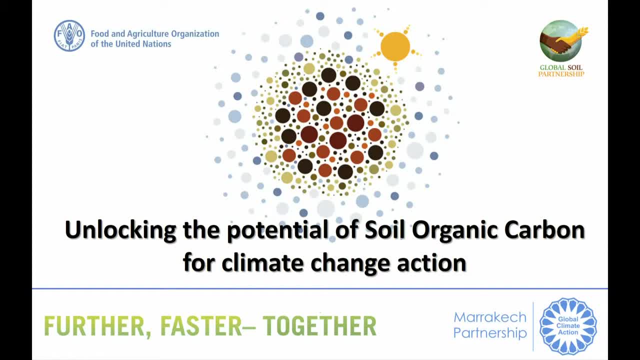 is, of course, extremely important, Also through the WCRP C-MIP. that's the model intercomparison project that feeds directly into IPCC. there's a specific initiative that deals with the coupled climate carbon cycle modeling efforts, But in WCRP 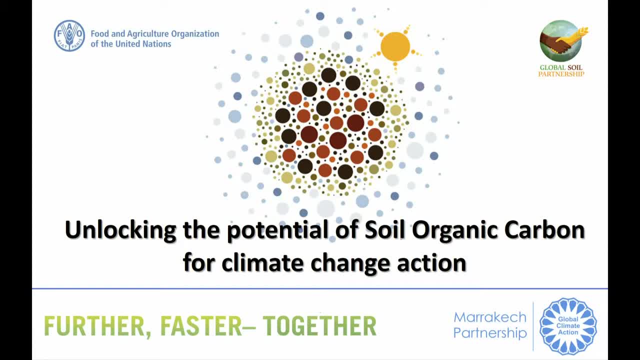 there's also one of these grand challenges that deals specifically with carbon in the climate system. So I think, from the WMO perspective, we really deal with this thing in a holistic way. but it's the detail, like the detail we discussed today. 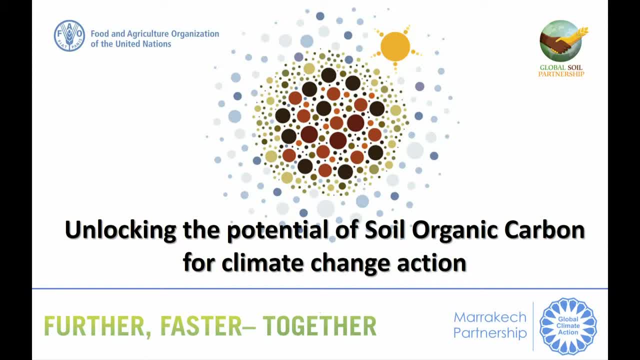 that needs to build up into getting a better picture of what is going on. I think I will stop there. Thank you very much. I think you provide a lot already: some very interesting and somehow scary information too, On the perspectives of managing soils. 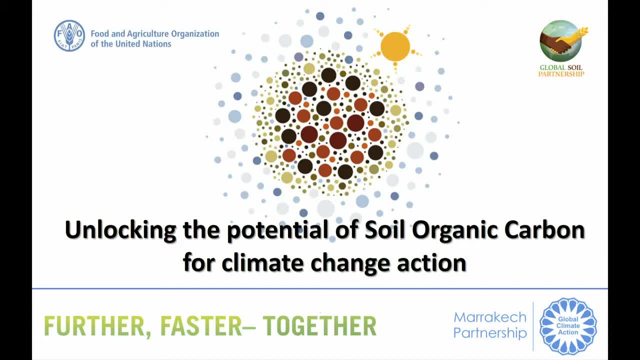 and the impacts on the climate change. I'm very glad to hear that the research is developing on this and we are learning more and more. Talking about this, Jean-Luc the UNCCD just finished its conference of the party in China. 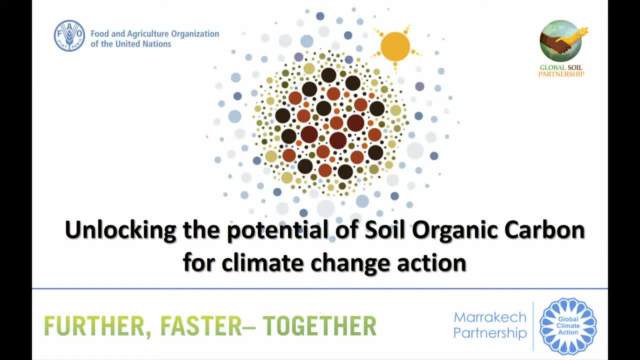 Land degradation neutrality target is now, I think, adopted by more than 100 countries and each country it's mentioned very clearly in the Sustainable Development Goal 15 on land in its target 15.3, having a land degradation neutral world, And we know that one of the metrics 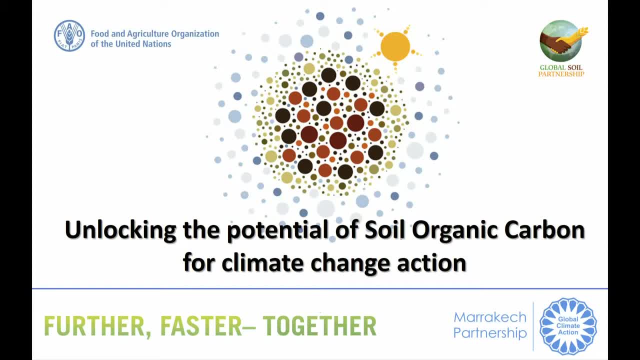 in this measurement for a land degradation neutral world is soil organic carbon. Can you tell us about the benefits of achieving a land degradation neutrality and how are we moving towards getting the countries prepared to measure and to report on the land degradation neutrality? What impact on their economies? 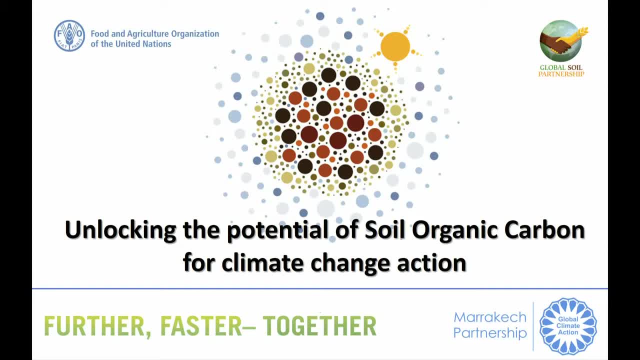 Why they should engage on this And if you think that this is soil, organic carbon sequestration is feasible everywhere. is it a recipe for all countries? Thank you, Just before asking you this, your last question. land degradation neutrality is built on three main metrics. 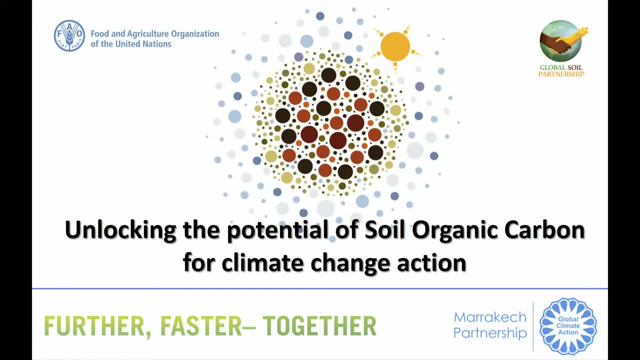 soil, carbon stock and land cover and land productivity. And what say the LDN framework that we need to bring on the ground, action plan for action that will fit all these three main indicators. These three main indicators are, I would say, one out all out. 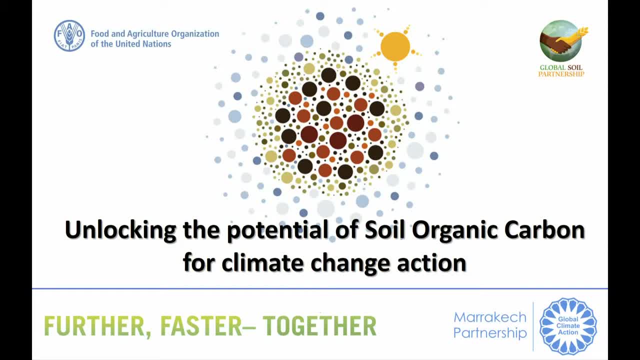 That's the main key message: If you provide a sustainable land management, this sustainable land management should fit in these two indicators. And, by the way, I take the opportunity that, at the same time that designing the LDN framework, SPI just did a data analysis. 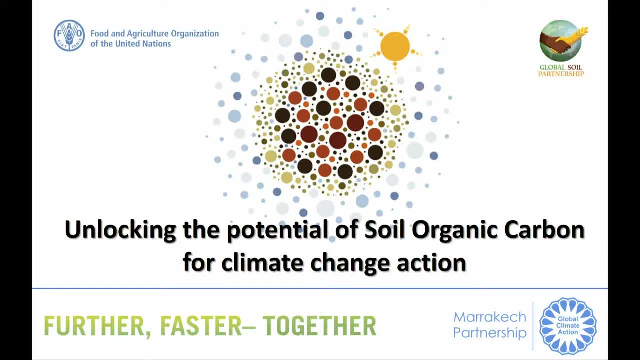 on sustainable land management to address drought, land degradation and desertification. And you will find in this technical report a meta-analysis telling that if you do agroforestry, if you deal with cattle or if you integrated fertilizer management, you will have impact of carbon stock. 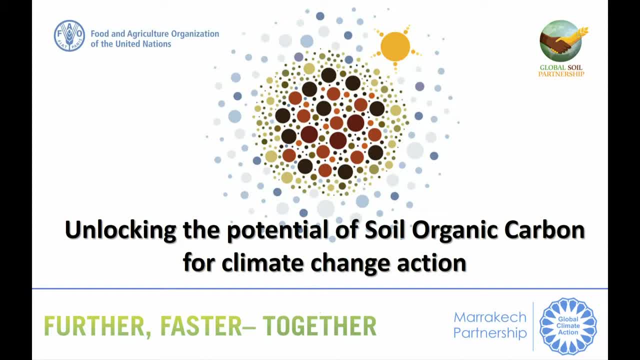 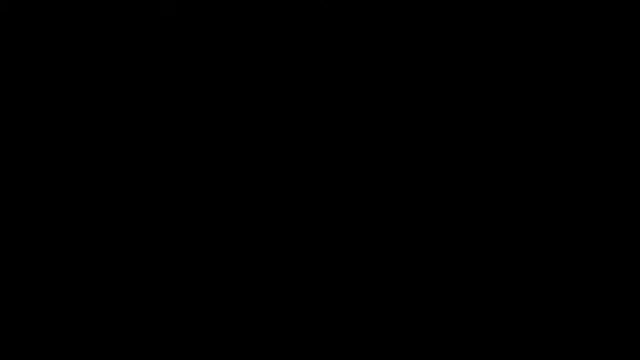 but also on biodiversity and so on. So it is why one, if this type of sustainable land management are brought to the farmers, they will be able to improve their income, because as far as you increase soil organic carbon, you will increase soil fertility. 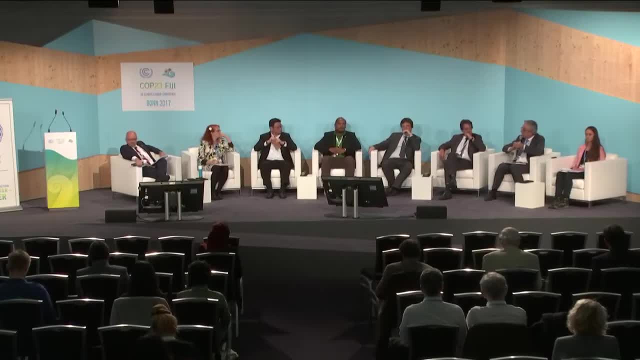 and we are expecting to increase yield. That's the first point. That's a local And at the national level, if we look at, FAO did a very nice analysis on NDCs and we all know now that NDCs are on the agenda. 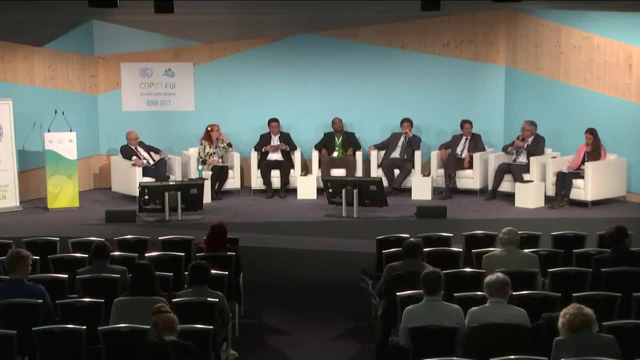 agriculture is on the agenda of NDCs of most countries, and particularly in developing countries, to mitigation, but also to adaptation. That means that by providing or by, you know, supporting sustainable land management, addressing degradation, desertification and drought, parties will be able to fit in the NDCs. 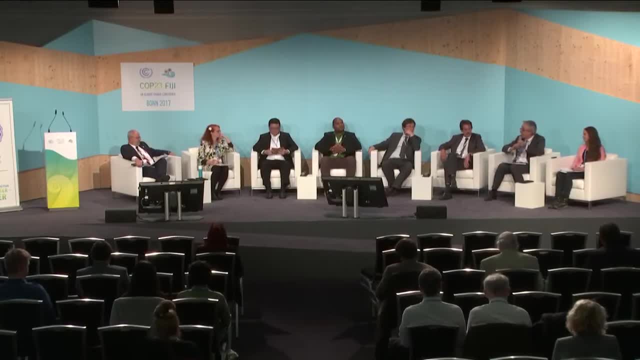 and to contribute at the global scale to the mitigation of climate change. So that means that there is benefit for local farmers, for countries, but also at the global scale for all the community. And the last question: Yes, The first thing on land degradation neutrality. 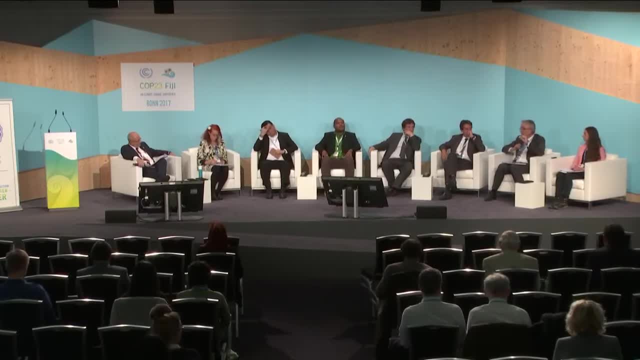 is to prevent degradation, to prevent soil organic carbon stock, to decrease, to avoid that and to try to increase. Of course, if you see the carbon map, the carbon stock is not the same everywhere because it will depend on land management practices, but also on soil texture. 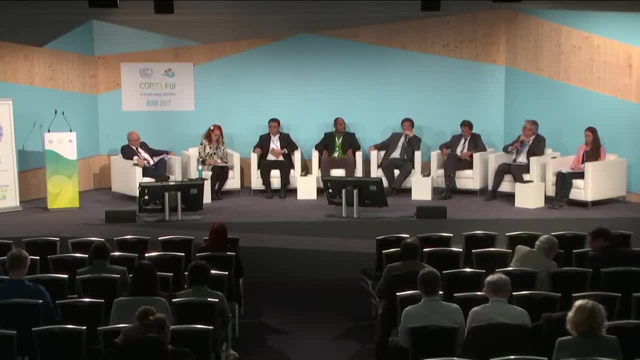 So we can increase, but accordingly to local condition, but also socio-economic condition. It is why, in one country or in one place, we should provide farmers with incentive to be able to transform their way to produce, to be able to, of course, meet their need for food. 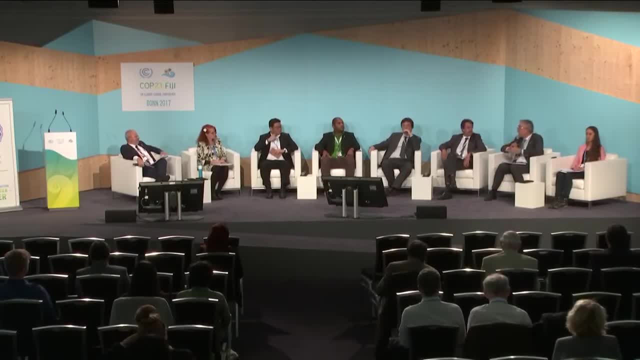 that food security, but also to make them part of the solution combating climate change. So we can achieve. we can increase soil organic carbon, but not at the same level everywhere And science, research is trying to figure out where are the best location. 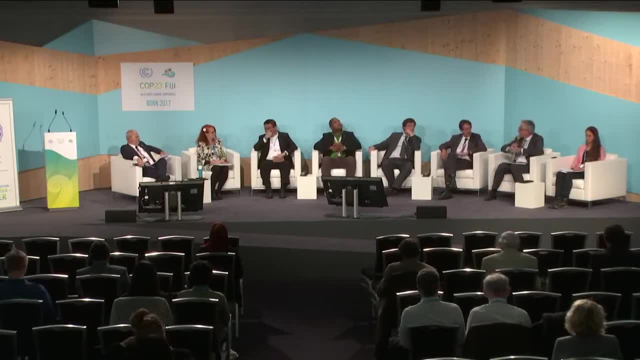 the best means to increase soil organic carbon stock. Thank you very much. Looking from my perspective, looking from agriculture perspective- I'm from FAO- I'm very happy to hear what you said: that sustainable production and avoiding degradation is the first step. 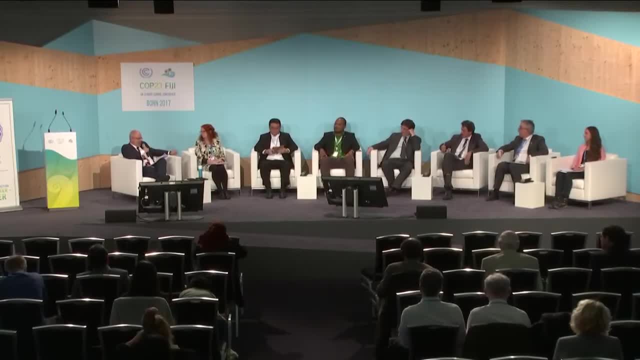 And we have here with us Nazir Fouad, who is the head of the recently established peatland restoration agents in Indonesia, And we would like to hear from you the challenge regarding conservation and restoration of peatland in a situation where livelihoods of smallholders 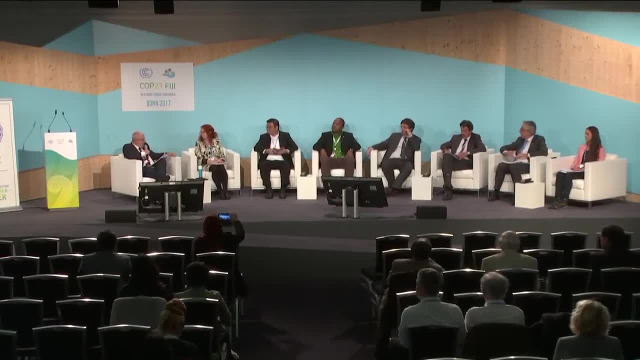 are dependent on the use of peatland. You have to look at it in the aspects of conservation, restoration and livelihoods is a big challenge that you have in your country and we would like to learn from you how you are approaching this. Thank you, 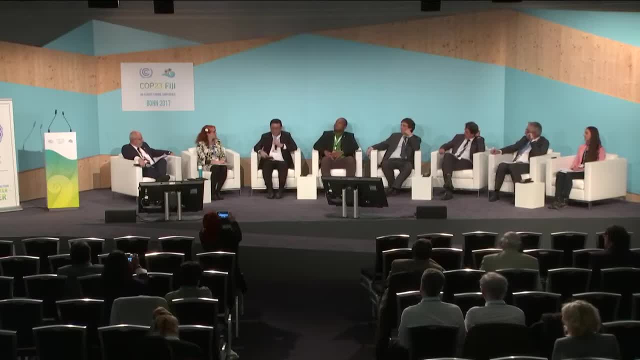 Yes, indeed very tough situations. Let me describe this first. Indonesia have about 15 million hectares of peatland. If we are in Germany now, I guess that is double than the largest state in Germany, which is Bavaria. So it's about double than Bavaria. 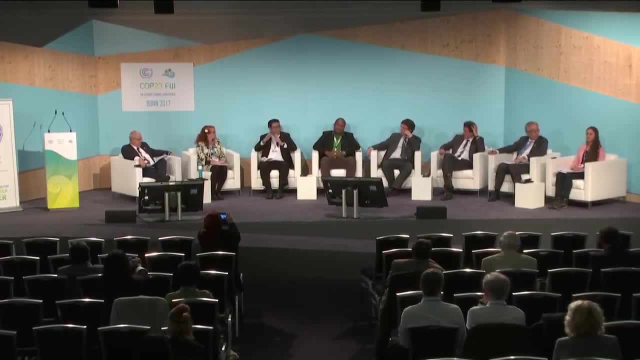 And out of that, 15 million hectares of peatland spread in several provinces. There are one province, for example, which more than half of the land is in peatland. That province size is even bigger than Bavaria and half of it is in peatland. 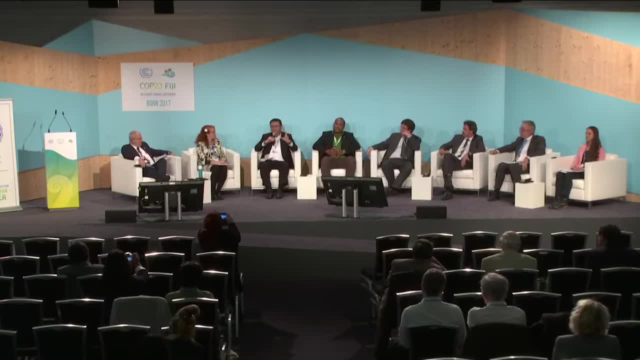 And in that province there is a district which size is also quite huge- It's like five times than Luxembourg- And 96%- 96% of that district is in peatland. So there are people, of course, living there Traditionally, some of our farmers. 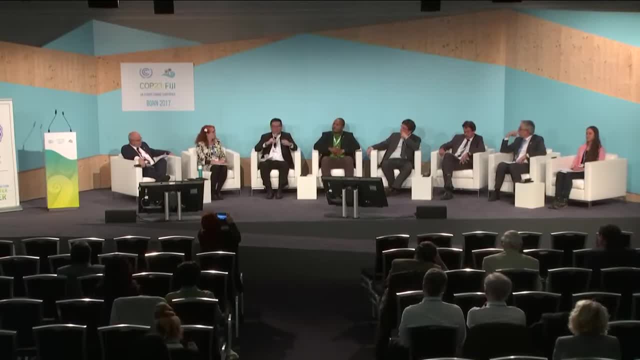 have been cultivating crops that are suitable for wetland in the peatland traditionally, But we face a much bigger problems in the last 20 years or so when a huge track of peatland being drained and converted for commercial large size plantation. That is the problem we're facing. 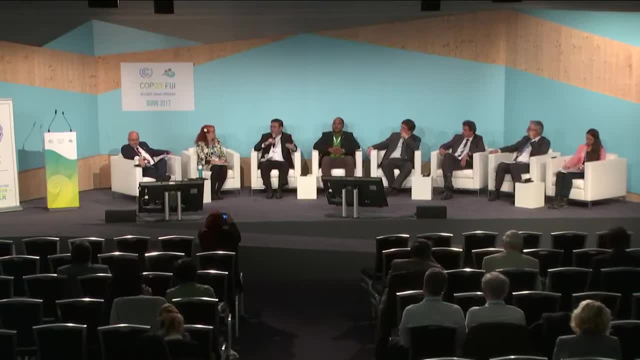 It get drained too much. It started a huge forest fire in 2015, when we have strong El Niño. I think some of you must have read some articles published by scientists or in the CNN and Reuters that saying that in the worst week of the forest fire in Indonesia. 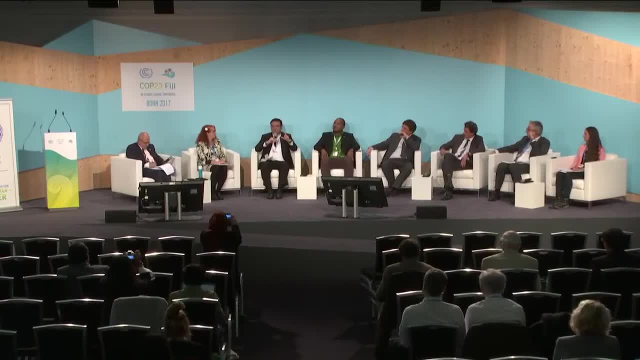 the daily emission. carbon emission of Indonesia exceed daily US for daily for two weeks. So it was very bad because of the fire in peatland. That's why in 2016, early in January, the president set up this agency to overcome the situation, preventing 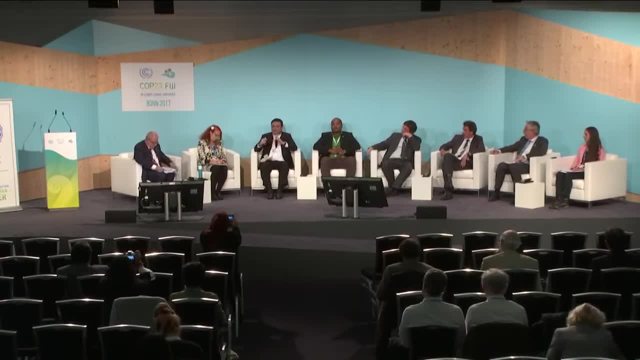 this kind of problems anymore. So what we need to do is, of course, first protecting all the remaining peatland which have not been opened. Keep it intact. Second, we need to restore this already degraded and drained peatland, But we have to also recognize peoples. 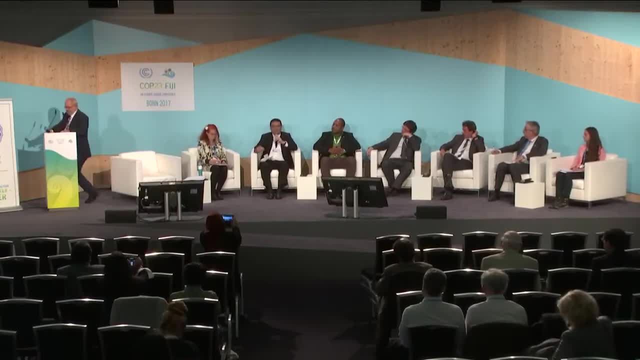 using those peatlands, including some companies which have already got license, legitimate license from previous previous governments that we have to also respect. So what we're doing now is we're developing methodology in doing the hydrological restoration. So in the dry months we try to keep the peatland. 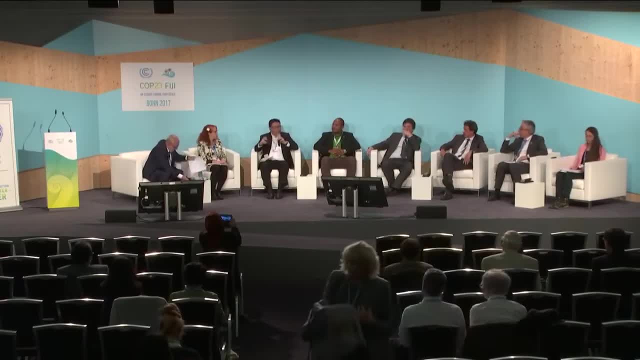 still moist and wet so it's not easily caught fire. At the same time, we're experimenting agriculture techniques with communities, with farmers, so their livelihood can improve. We have very good examples in certain areas in Kalimantan, in the islands, That some farmers 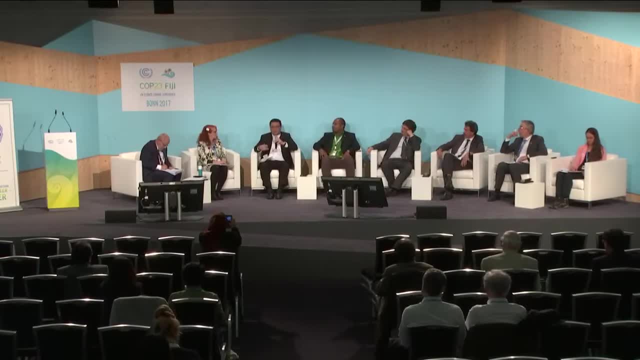 indigenous people have using peatland for rice farming, But they're doing it once a year only, And that's why in the dry months they let it dried by under the sun and then they burn it before planting it. So we try to keep the production. twice a year. So at least there are no times for leaving it and then burning it And we can get to a point that the productivity per hectare increased at least double. So if they're not planting twice a year, they got four times bigger yield annually. 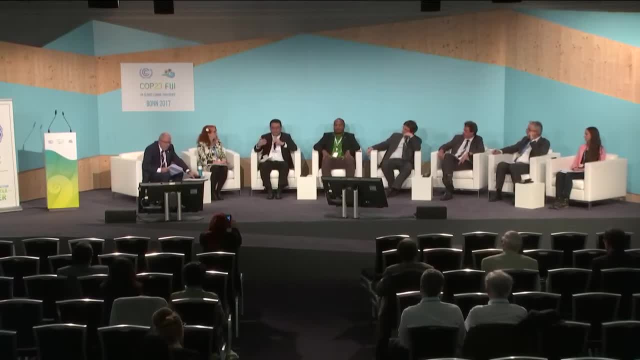 But of course that needs a lot of not only agriculture but also more like social and cultural changing. Farmer behavior is not easy, I'm sure. I mean all farmers around the world are the same, And then in the meantime we engage with a lot of scientists. 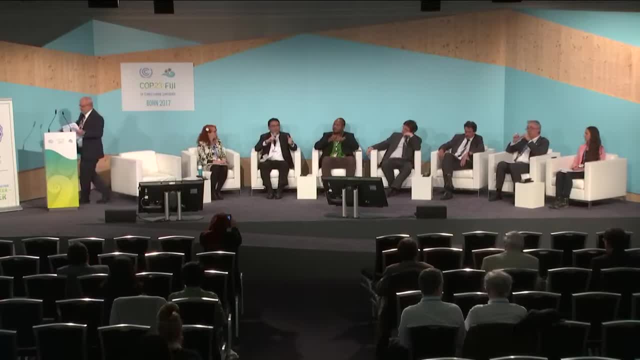 To do several things. First, in doing the hydrological restoration, we need to have a quite accurate estimation or a measurement on how well, on how high, the water table increased Daily, weekly, monthly, covering the whole peatland. We put out a sensor right on the field. 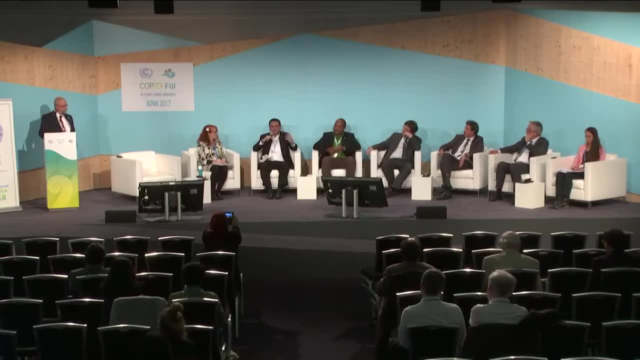 But if we're talking about peatland size of 15 million hectares and spread all over the country- Indonesia is quite large, It's like Portugal to Moscow- The width of the country- Then it's a lot of work and very expensive. 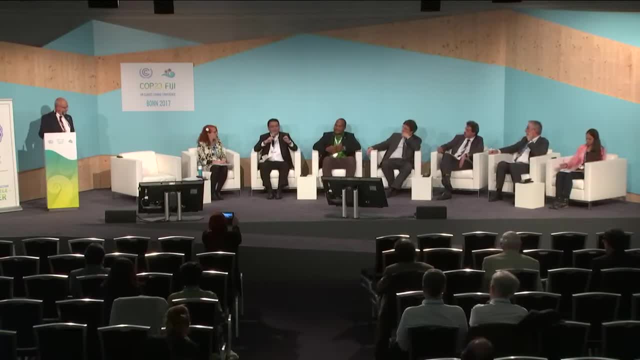 So putting that sensors, also coupled with help by some scientists. We're still developing the technique in estimating the soil moisture from satellite images. So it's combining the real measurement as well as satellite, And some scientists show us that they can estimate more or less the carbon emission. 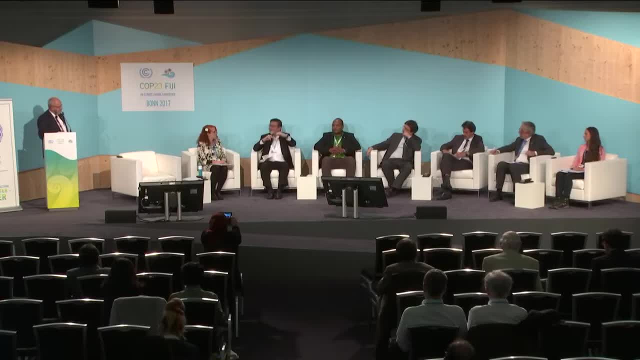 reduction if the peat is getting wetter and wetter. What does it mean? if this kind of peat have two centimeters water higher? It will mean less decomposition of this carbon on the soil and meaning also less carbon being emitted. Some science of doing monitoring. 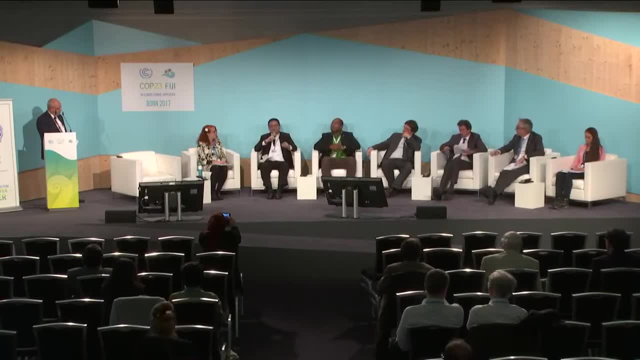 We need it a lot. Also science on how getting more productivity of crops that can grow well on peat. We're talking with FAO in Indonesia about paludi culture, for example. And also science dealing with big corporation, because the corporations also get huge already. 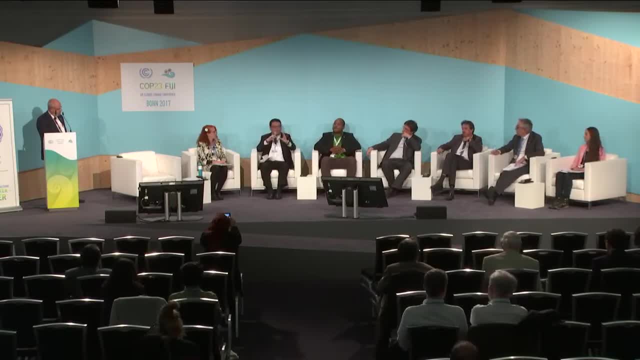 licenses and how the business model of the corporation can be justified, What kind of crops they can also modify. So if the license have to be still going on, how can they make a good business without getting the draining, continuing This kind of stuff? Thank you. 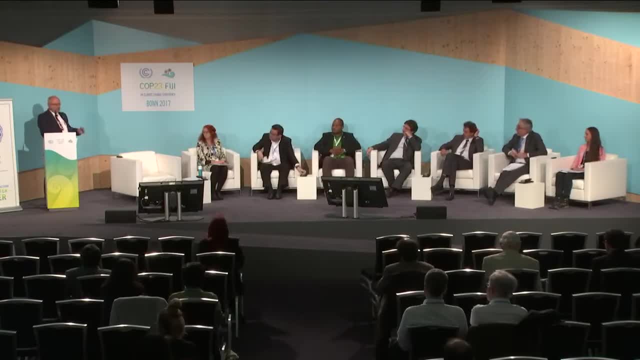 That's a lot. Thank you very much, Nazir. I think we heard the presentations of Luca and Takini. We heard the points, that key points that have been raised by our panelists and we don't have much more time, but I would like to hear from you. 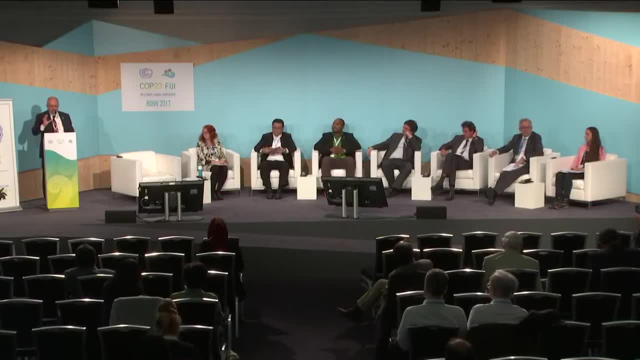 If you have any question, comment or a sharp point, Unfortunately you have to speak at the micro because we have interpretation. There are two micros in the middle of the room. or if you are sitting here in the front, I can just handle mine. 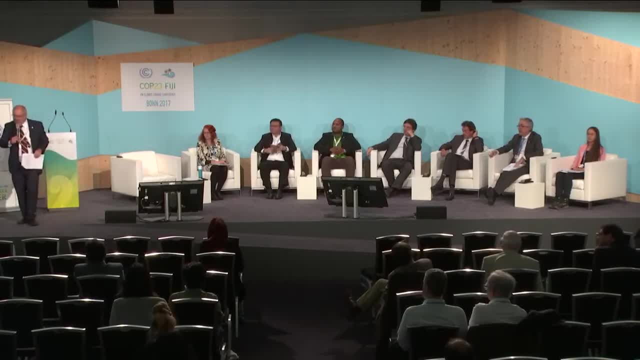 Identify yourself and then let's try to do a one minute question. Sorry, but we will have to be very time effective here, So just be sharp, identify yourself and put your point. Hello, My name is Judy Sol, from Mother Channel and from Cape Town Television. 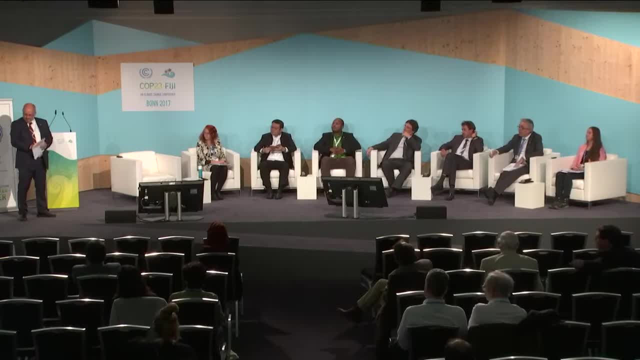 I have an important question because I have believed that the soil microbes may be coming to the rescue of the phytoplankton in the sea, who are dying with the increased heat that the sea is absorbing and with the increased acidity and chemicals that the sea is absorbing. 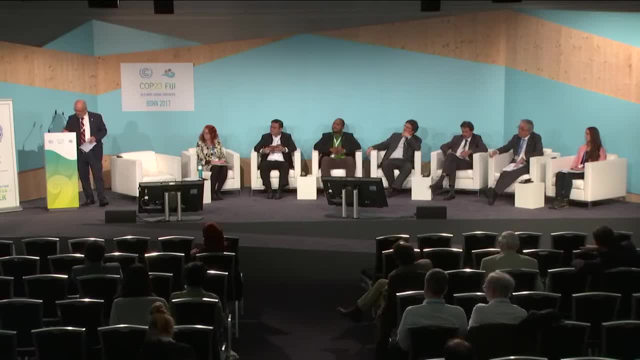 and I was wondering if you think there is any possibility of being able to scale up, not only for agriculture but people all over, to make nurturing microbes a prior responsibility to try, and because biomass under the soil is one of the fastest ways, I think, of getting carbon dioxide out of circulation. 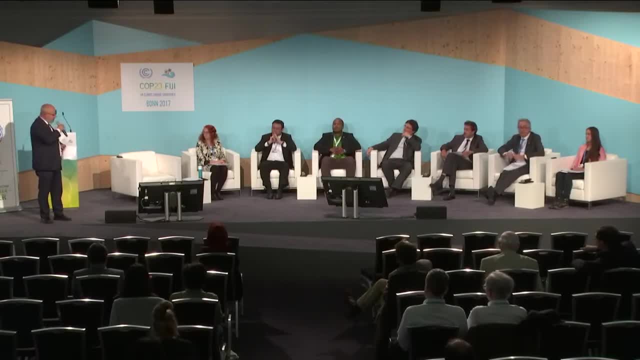 Thank you very much. The relationship of soil biodiversity in the carbon and the climate. I have two persons queuing. Would you like to put your question? Sure, Matthew Warnken from Corporate Carbon. We are carbon project developers and aggregators in Australia and recently. 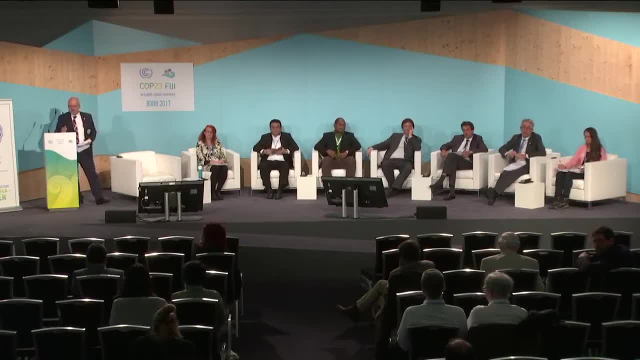 we convened a soil carbon practitioners industry working and we are very much invested and involved with on the ground soil carbon projects. My question to the panel would be twofold. One: firstly, what do you think the potential actually is worldwide for soil organic carbon? 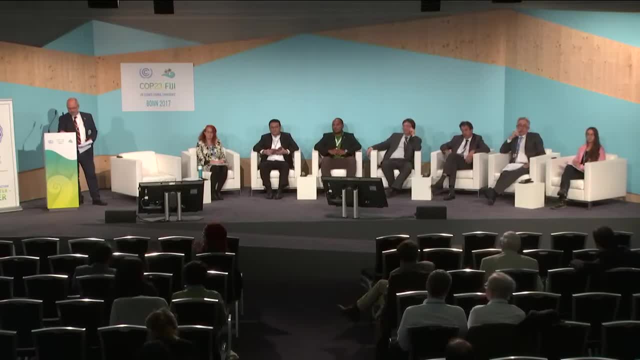 to deliver sequestration. So in terms of quantifying that potential, and then what is then that key to unlock us in terms of achieving that potential? So I guess twofold comments from the panel would be very much appreciated. Thank you, Thank you very. 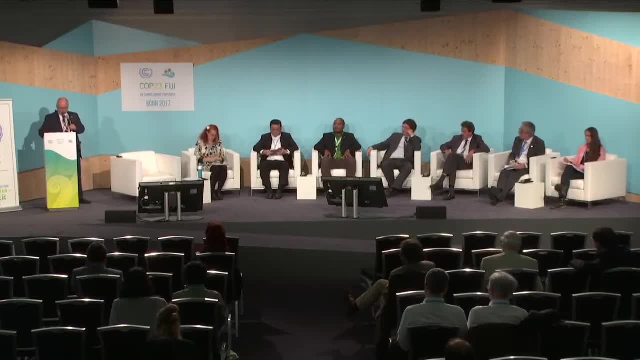 much, Very precise, The potential of the world to sequester carbon in the soils and the key elements to achieve it. Then I have a lady over there. Please identify and put your point. Yes, thank you. My name is Anne-Laure Sable from. 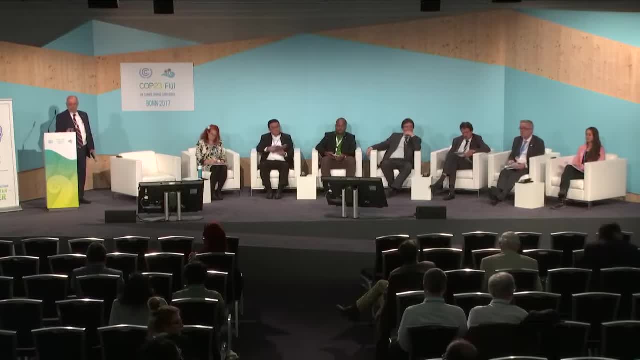 French NGO working on soil carbon sequestration. So I wanted to maybe to highlight two remarks. I really appreciate that Minister Fidji talked about food and nutrition security. I think this is very important and we tend to talk about a lot of food production but actually food security. 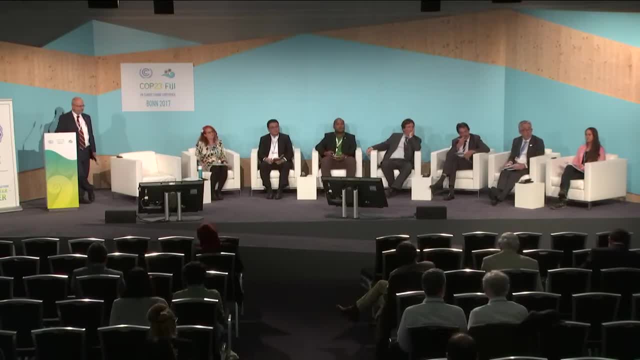 is also about access, quality and stability, and we produce enough to feed 12 billion people actually, but we have a lot of loss and waste and there are still 815 million people suffering from hunger and we also have 1 billion people with overweight. So I think 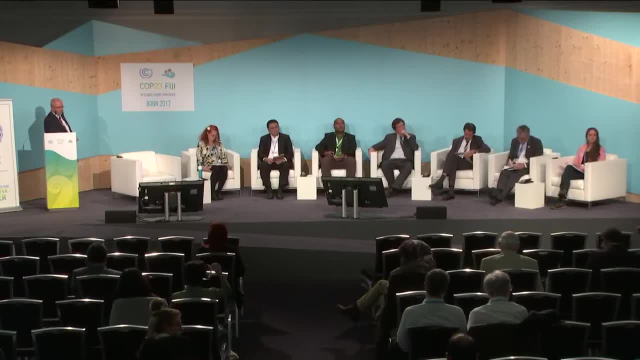 we need to really try to broaden a little bit the discussion about food security and not only focusing on food production and on soil carbon sequestration. Two things that I haven't heard from the panelists is about non-permanence, because soil carbon sequestration when you reach the equilibrium. 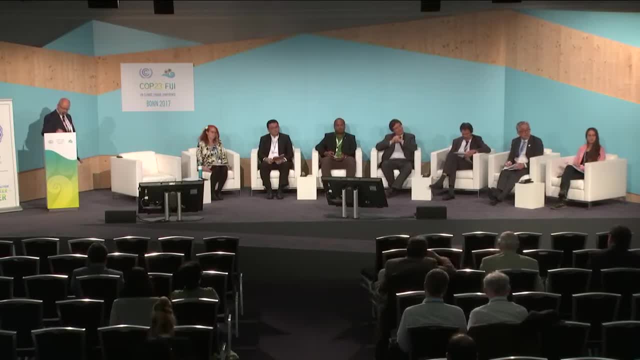 of the sequestration of your things. then you won't sequestrate anymore. So it will be just about maintaining and storing the carbon. so it won't offset forever agricultural emissions, and obviously agricultural emissions are about methane and nitrous oxide. If I'm 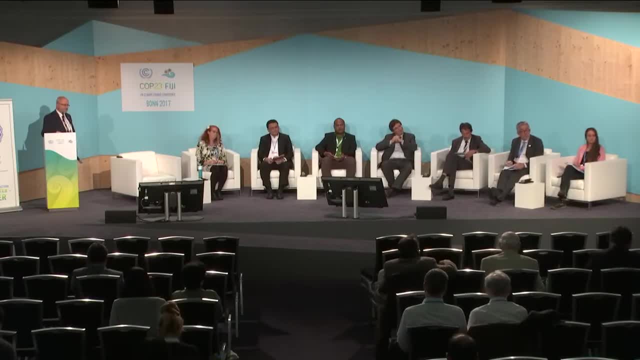 not wrong. the IPCC, AR4 or 5, you may correct me- is saying that actually the carbon cycle is neutral for agriculture and that mostly we are talking about methane and nitrous oxide. So I'm a little bit confused about this non-permanence not being 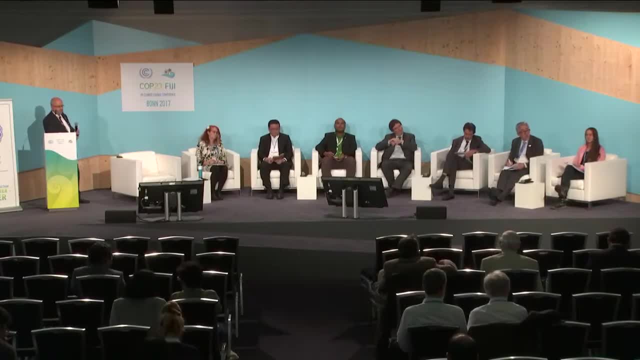 addressed during this conversation and uncertainties about publications. We have so many scientist publications saying now that we have a very wide range of results. Sometimes you can sequester carbon, sometimes you can't, And it's more about adaptation actually that we should talk. 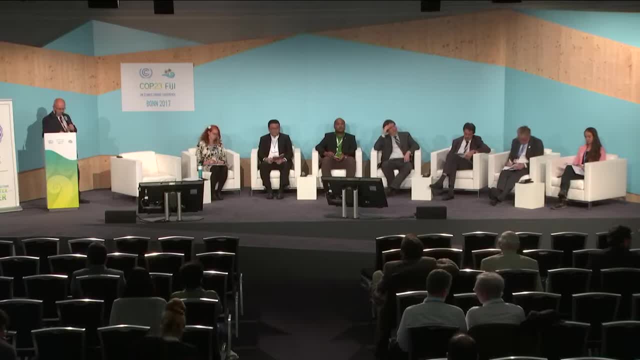 about soil carbon sequestration and we are talking a lot about mitigation, but I think mitigation should be about reducing non-CO2 emissions from agriculture, so it's permanent reduction and maybe we should focus on adaptation with, I would say, potential co-benefits. about: 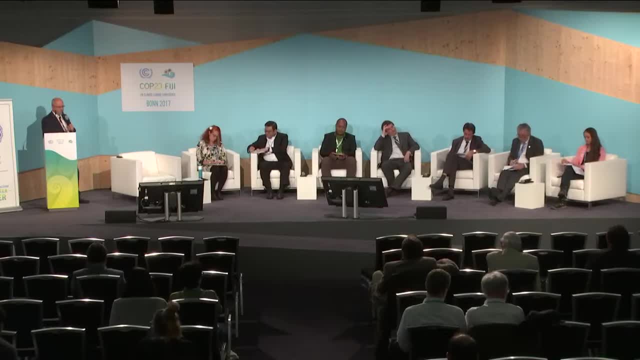 soil carbon sequestration, land degradation, neutrality, soil erosion, fertility- This is the main objective. I think about soil questions and soil organic carbon. I don't want people to think that we have like an Eldorado of carbon and that we should just go. 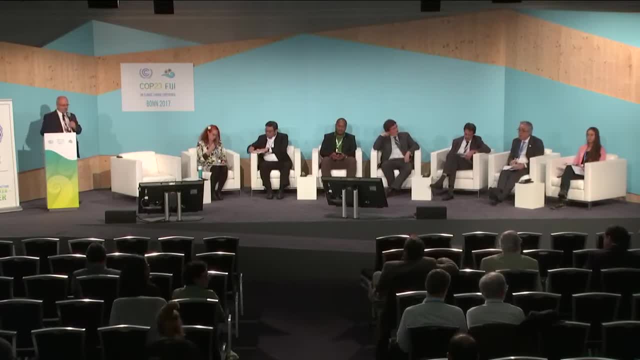 for this and not addressing other permanent reductions. so please be careful with that, and I would like to see how the panelists think about having an adaptation approach rather than a mitigation. and if people are interested, we have this statement made by an organization called Our Land Is. 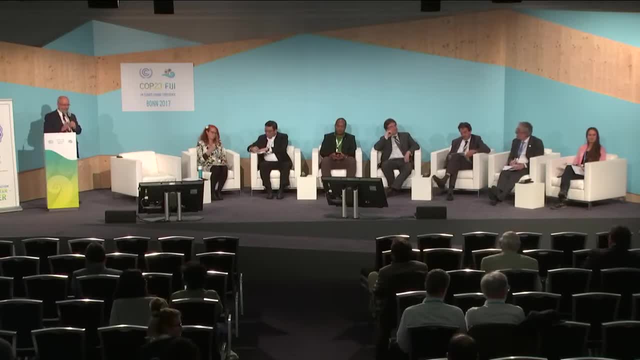 Worse More Than Carbon. just to try to have a broader picture, a holistic approach about soil, carbon sequestration. Thank you, Thank you very much. I think there are people willing to applaud. Thank you, You made your point and I think we took note. 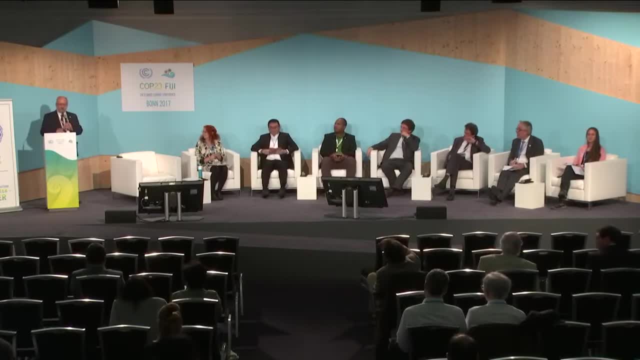 of the food relationship with soil, organic carbon, with the non-permanence and the issue of let's do mitigation, because that's it. There's a whole point on adaptation that has to be taken care. I would take the last question now and please identify. 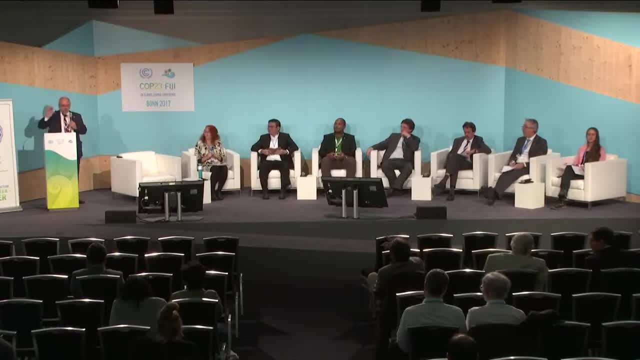 and go to the point: Oh, there are two more. That will be the two very sharp one. Identify and put your question, Then I will pass to the panel and I will give you two minutes for you to pinpoint. I'm very happy to see that the questions. 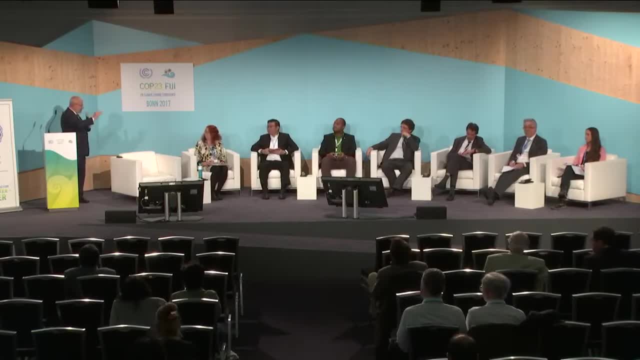 are very cross-cutting in general, so I think it will touch the heart of each one of you and you put your approach. And then I'm looking at Terran in the end, with the complexity of bringing this to the reality of the custodians. 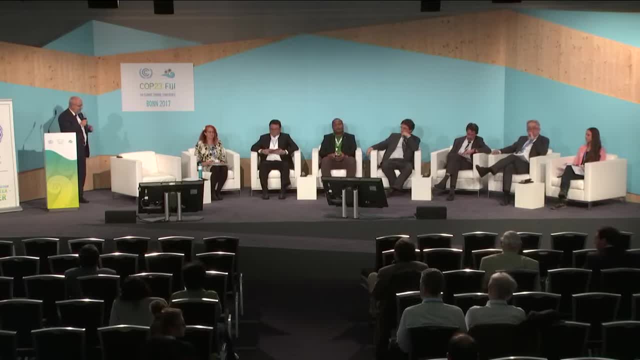 of this land that we are talking in the soil, the farmers. I have the gentleman there, Then I'll come to you and then you will be the last question. Please, Thank you very much. My name is Johannes Lehmann. I'm a soil scientist faculty. 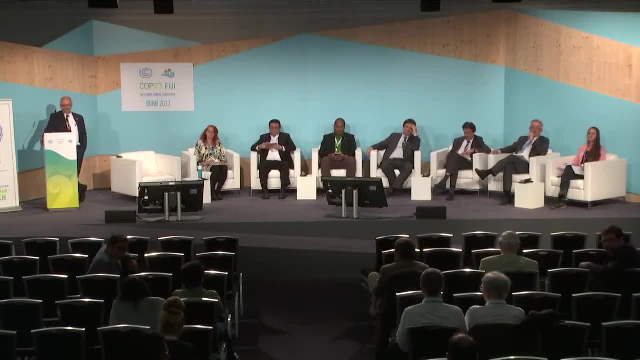 at Cornell University studying soil carbon. I commend the different organizations to produce the soil carbon maps. That's an essential resource. I was wondering how we can move from a static soil map to a more dynamic soil map that is changing, with practice-based modeling and 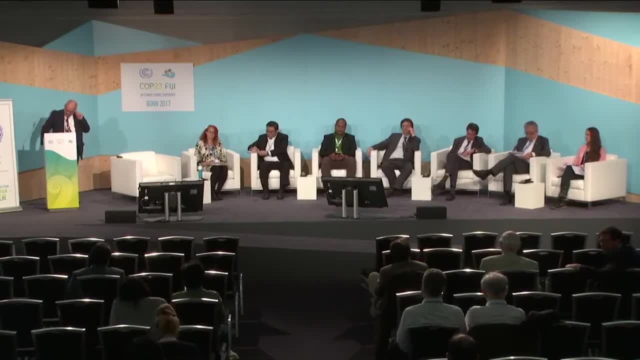 what kind of institution would volunteer to be the clearinghouse or the funded program leader for such an effort? Thank you, Thank you, Very precise, From static to a more dynamic soil map, and who would host this? Now I think you may use my microphone. 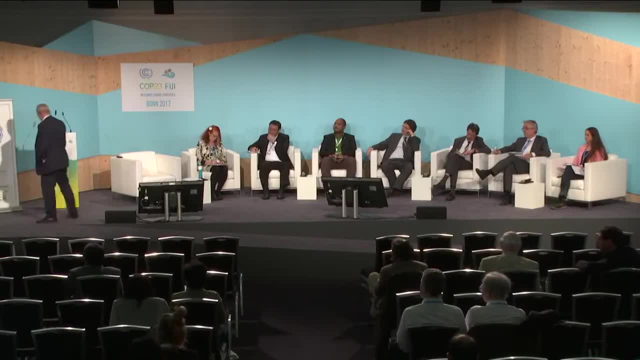 Thank you very much. I'm Arthur Reitacker from France, and we are a scientific and technical NGO for sustainable development. I used to work very much in Africa in the past. My question is: you have a whole range of solutions to decrease the emission of CO2. 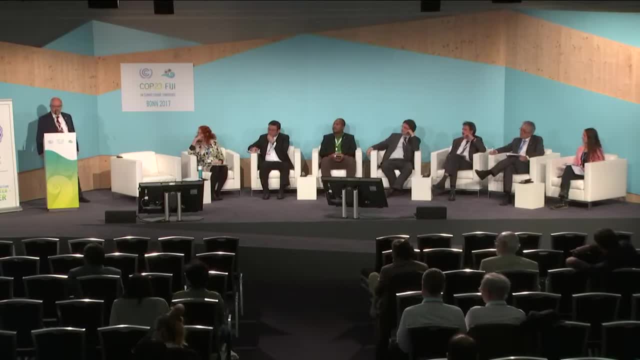 from the soil. Of course, when you go to Indonesia, in peatland it's a very serious issue and you have to deal with that first. But when you come to Africa, I think the first thing is to increase productivity of land. 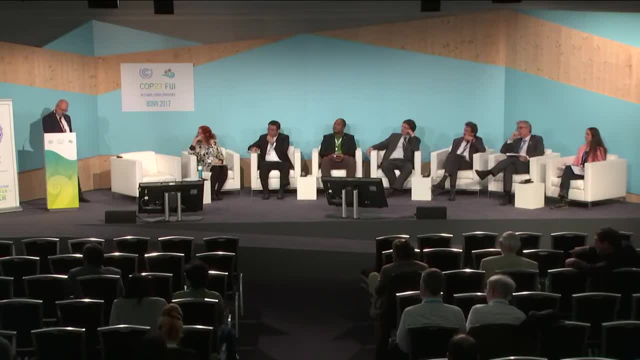 to avoid deforestation, because the population is going to double in the next 50 years or less. That means you can either double the area that means deforestation, and the deforestation will send in the atmosphere much more carbon than the amount that you can store. 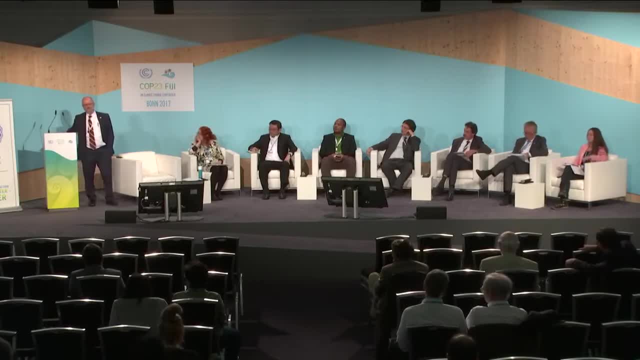 in the soil. This is really a main issue, and if you don't tackle with that, we are not going to tackle properly with the issue of food security either. Thank you very much. I see this more a statement in which we entirely concur that. 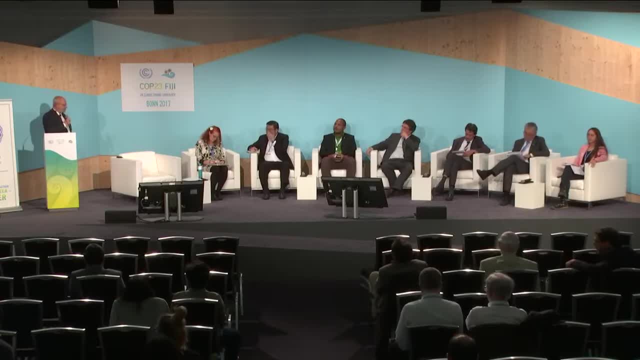 increasing productivity is the backbone of feeding the world. If we give two minutes to each panelist, we have 12 minutes. That's what you have, and then we still have a few minutes for Terran to wrap up and we will conclude, with some delay, but still. 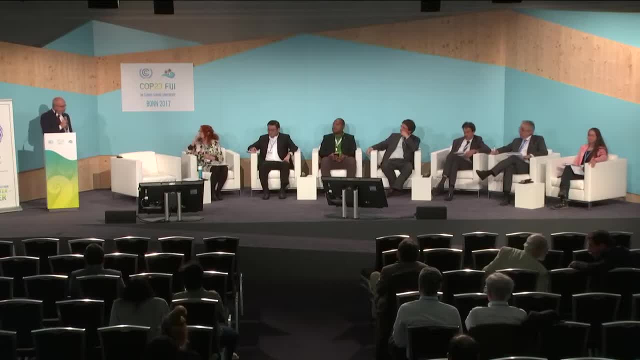 on time. We have five questions, or maybe four questions and one comment ahead of us and I think you took note: The relationship with sea soil, the potential on the sequestration, the relationship of food adaptation and non-permanence, the static versus a dynamic soil map. 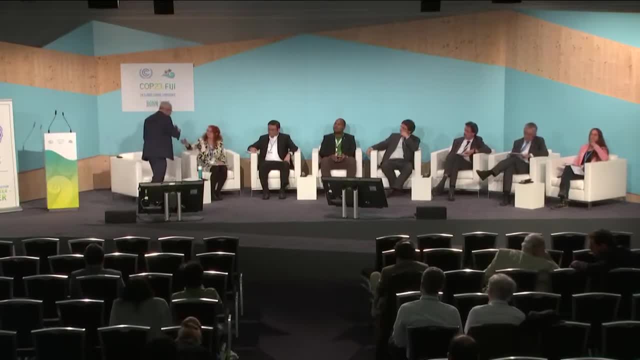 and the issue of productivity. Let me start with Jo. Thank you for some very interesting questions. Soil carbon and biodiversity. just to say that soil carbon biodiversity tends to increase with soil carbon, so anything we do to improve soil carbon also helps with biodiversity, potentially, but I'm afraid 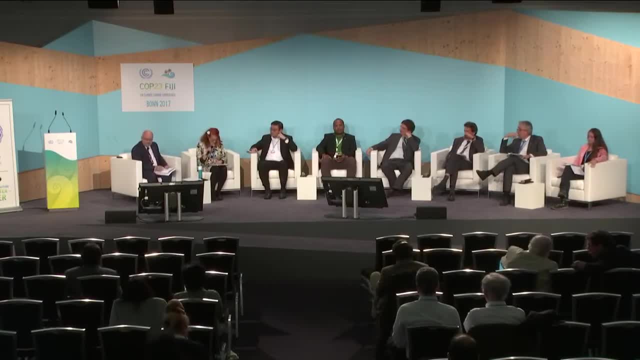 I can't talk about phytoplankton, I'm afraid I don't know too much about that. So the potential for soil sequestration. There's been a lot of recent papers. In addition to the one that Luca showed, there was a paper by Pete Smith that looked at 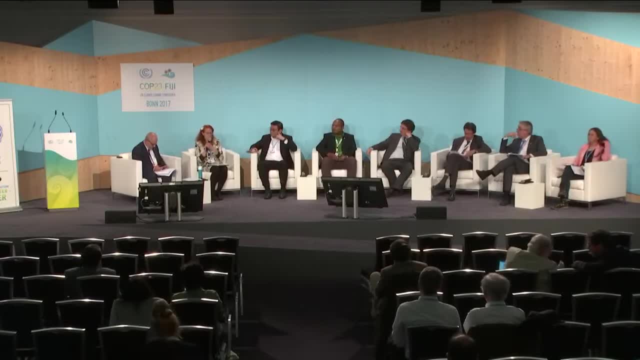 the potential for biochar and the potential for soil sequestration, both being about 0.7 petagrams of CO2 equivalent per year, and actually that touches on the other lady's question about permanence. Soil sequestration might reach a capacity that biochar. 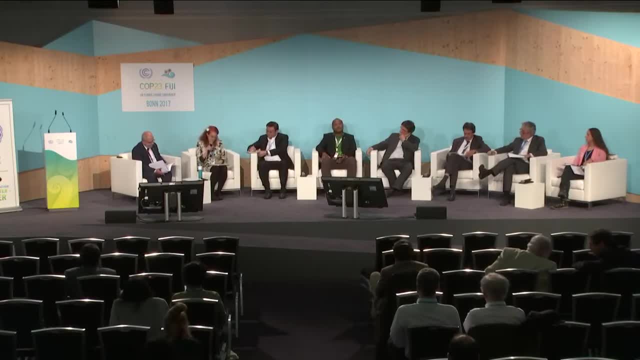 doesn't, You can continue to take CO2 out of the atmosphere That way. Then there was a very recent paper in. that paper was a 2016 one. Then there was a recent paper by Griscom just came out in the last. 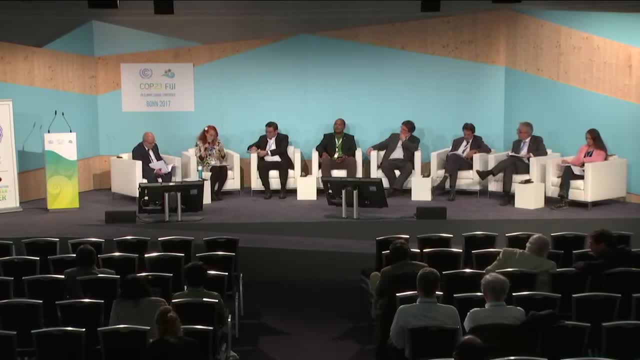 few weeks in PNAS That also looked at different natural solutions, and there they had peat restoration. coastal restoration, avoided peat destruction, all of those being about 1 gigaton of CO2 per year by 2030.. So, and that's something. 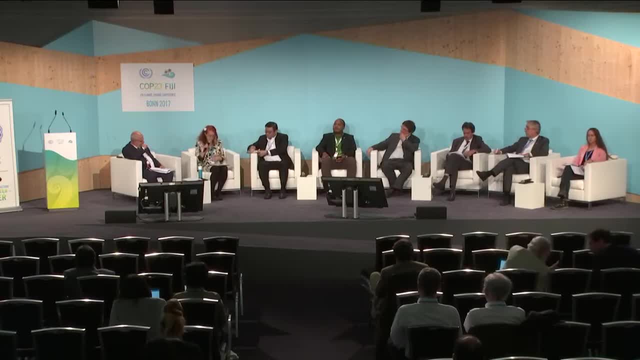 all of these sorts of papers will be reviewing in the IPCC special report on climate change and land And there was a comment on how you helped this to happen and actually having these things. if they're in the IPCC methods and countries have to report on them, then that helps to. 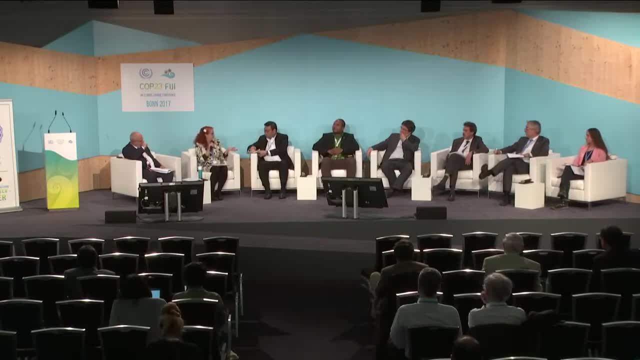 incentivise and there's a wetlands report that came out in 2013 that included a lot of new methods on wetland drainage and re-wetting. So if it's in there, then it helps to incentivise and that helps on the road to. 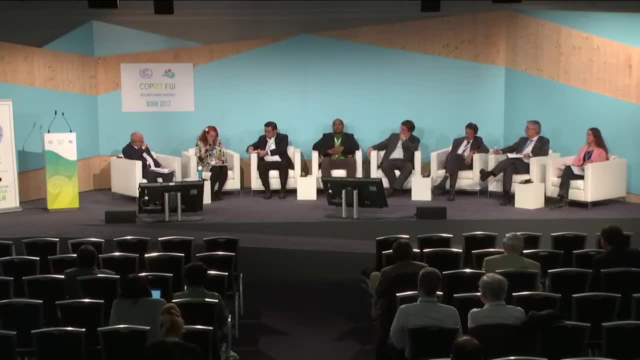 achievement, hopefully if they're incentivised with the governments. Again on a question about what's talked about, the permanence, but the non-CO2 emissions from soils are also considered important. There's a lot more information and, again, that's part of the IPCC. 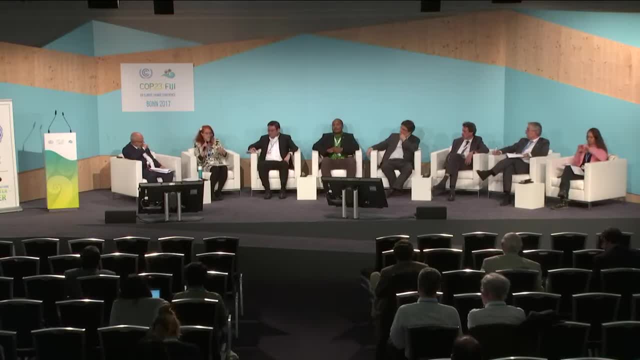 methods for countries to report on the non-greenhouse gas and again, it's part of something we assess in the assessment reports And totally agree about adaptation and mitigation co-benefits and there's a lot more talk now about mitigation and the co-benefits and there's been a lot 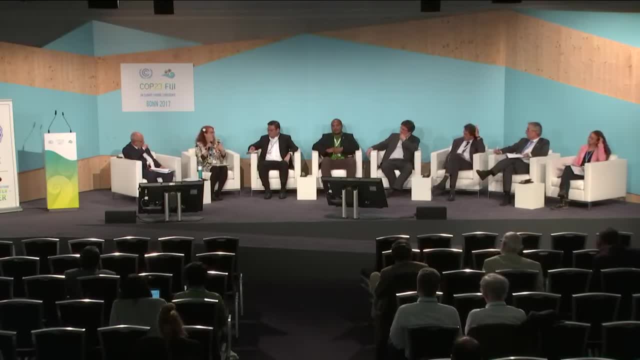 more information. Again, that's something we need to assess. There was another good paper by Pete Smith in Nature about that And mitigation- avoiding deforestation, I think was your point. I'm not quite sure and totally agree: Soil carbon options haven't particularly been in the integrated 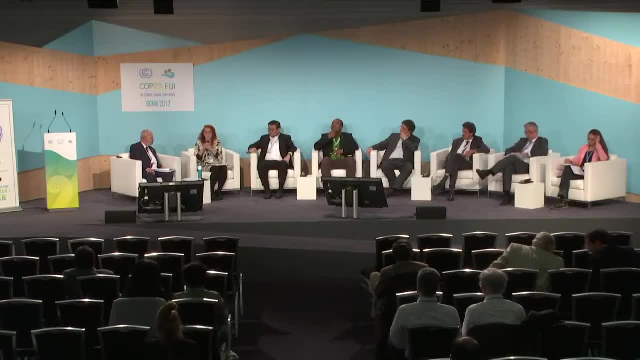 assessment model scenarios that the IPCC has available to assess and I think that's something we can do, moving forward to include that. But yeah, any mitigation options should really avoid deforestation completely. Thank you so much. Continuing on the science aspect, I think. 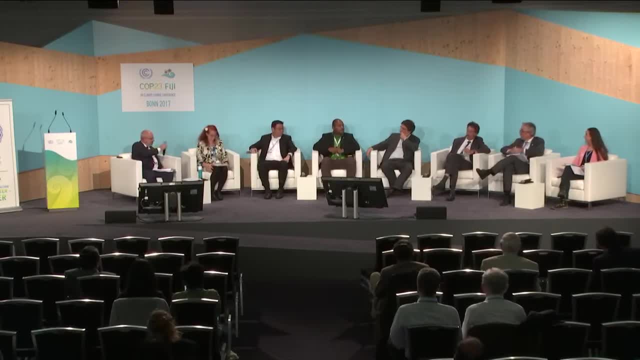 Jean-Luc, would you like to take your floor now, or you want me to go on the row? Maybe we can do this then. then we move to the colleagues from this side. I will be very quick and sharp. Yes, of course. 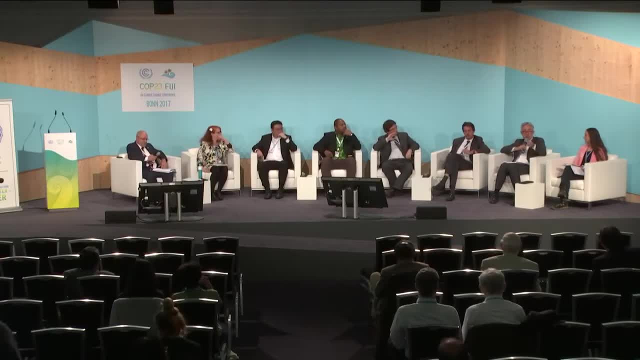 we are talking about permanent solution through building biomass production, because we have to keep in mind that to sequester carbon, we need to produce biomass. And, of course, this new technology with sustainable land management should not be implemented in one year. it should take almost 20 years. 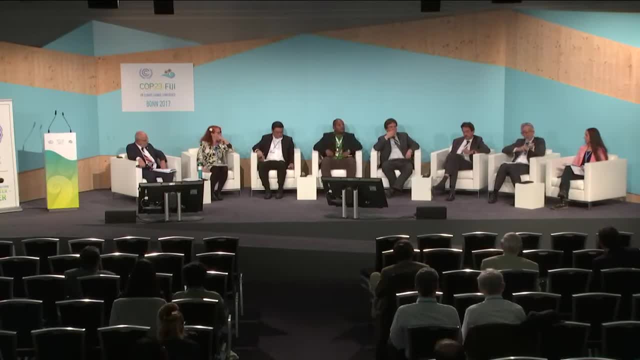 That's the way to do permanent option and to put agriculture on the permanent option for climate change And the good property. if you put more carbon in the soil, you need to have more biomass And by having more biomass you may have some more food. That means 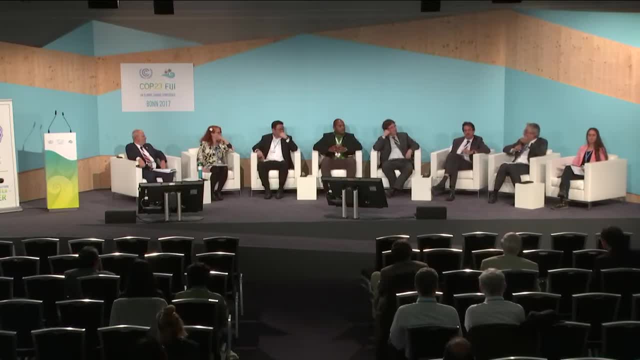 the loop is closed. Carbon, biomass, food security and adaptation. That's my main point. Thank you very much, Dion. would you like to contribute to the answers to these questions, please? Yeah, I'll also be short. I think that. 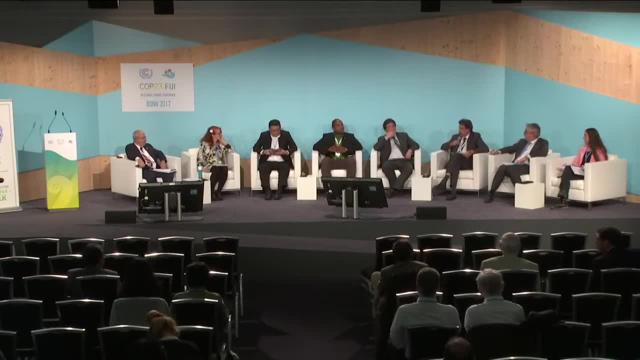 we are faced with really tough choices in life, especially as we move into this 21st century, And we've heard today that these tough choices require information and data and process understanding, And we have set up a system that works well And we 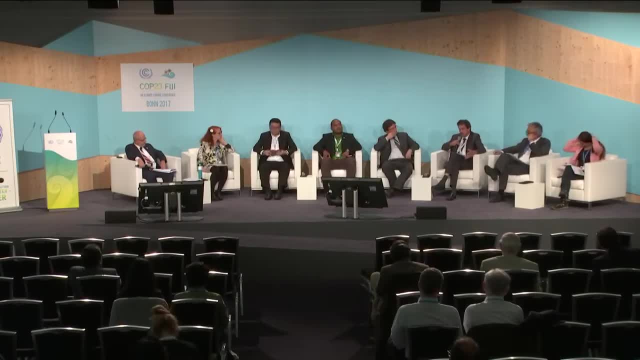 should use those systems- and I'll explain a little bit how I see it- but also invest in those systems that we have the information to make wise choices, And that system is the system of science being assessed by the IPC and then feeds into the UNFCCC. 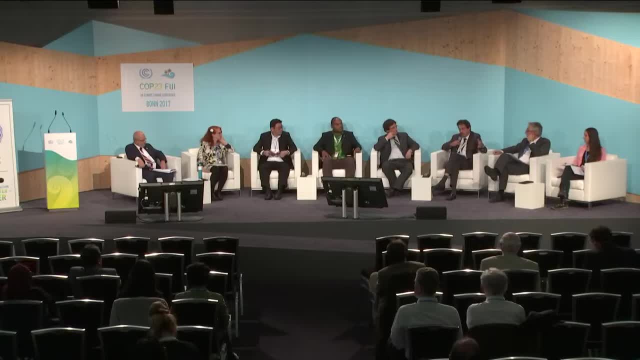 discussions And I'm fairly early in this food chain with the programs that I'm involved in- the World Climate Research Program and Global Atmosphere Watch. But I think this is the process, and at the beginning of this process is this detailed process: understanding of how the earth system works. 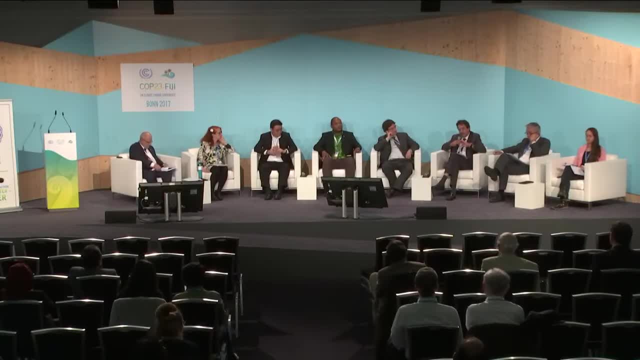 And this also applies to soil, organic carbon and the fluxes between the atmosphere, Because, as I mentioned in the beginning, we need not to lose our concentration on the atmosphere, because this is where the important processes happen, This is where the radiator forcing happens that drives. 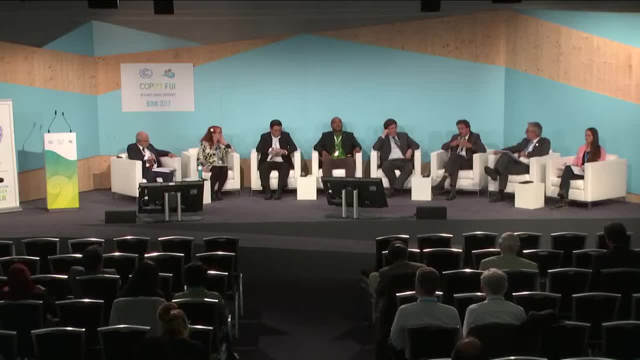 the temperature increase, and this is where the severe weather and the impacts eventually happen as well, And so we are intimately connected through our actions, through this complicated earth system, And only by understanding and measuring and modeling this better we will find the solutions. that makes a difference. 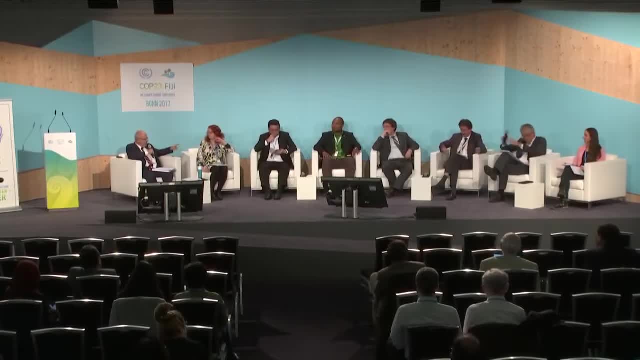 Maybe I'll go to the country perspectives before coming to you, Luca, because I'm looking at you with a double hat, With the ITPS, but also with the European Commission. So at the end we have to see how much does it cost? and 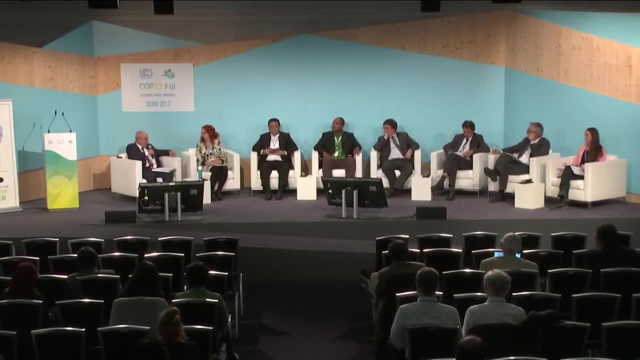 where we mobilize resources to put the science and the policy into practice. So I'll come to you on this, but I would like to hear from Nazir and from Takini from their perspectives on the peatlands and on the Pacific Islands and the questions that 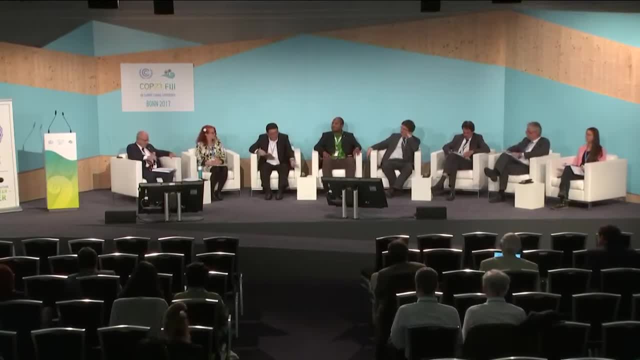 have been put. Would you come first, Nazir? Yes, What we learned in the last, let's say, 10 years or so? we believe that the weather extreme will happen more and more often. We've seen what happened in Europe and in the US. 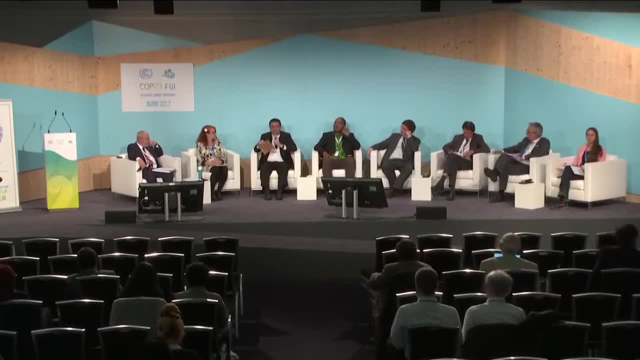 for extreme drought and fires happening And in Indonesia we believe that the peatlands which can hold water and a lot of Indonesian tropical peatlands, they are rain-fed peatlands, So if the water is not well kept and regulated during the rainy, 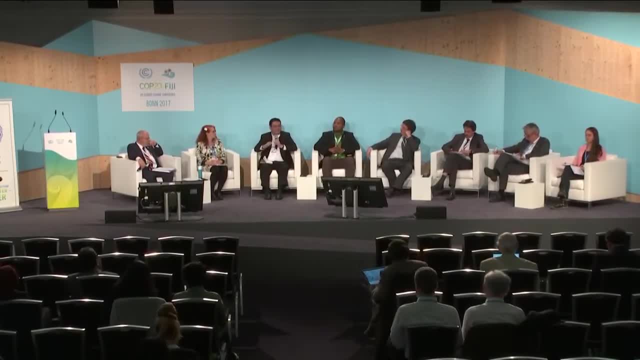 seasons. during the dry months it got not only dried but also the water that can be provided for lower areas will be no longer available. So if we can keep that water regulation well, it does not only avoid the fires in the peatlands but also. 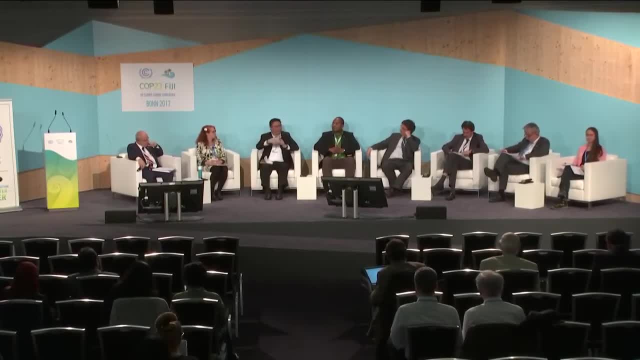 the water. can peatlands provide water for agriculture in surrounding areas? I think that's very important. Modeling on how the water should be regulated, modeling on how the rainfall continuing for the next month or the next week and when the rain stops and we're entering. 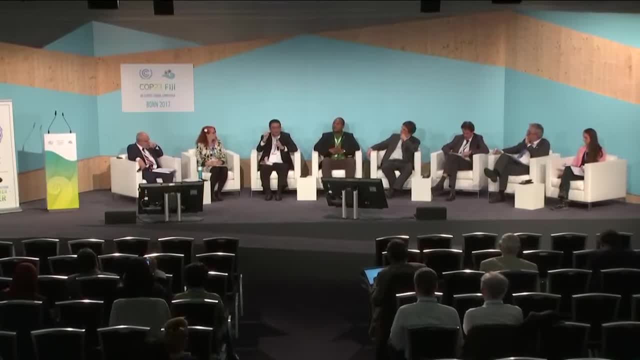 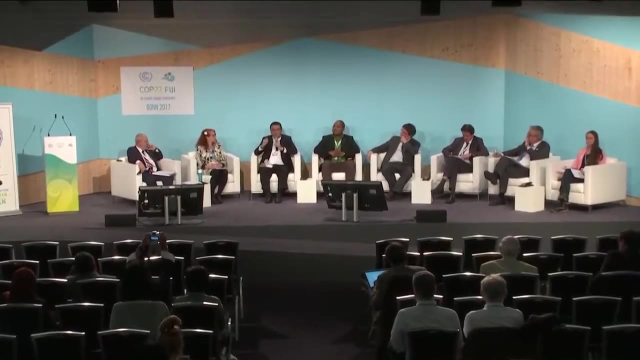 the dry season. all of that data is very useful for the management of the water regulations on the ground. I believe it costs much less than if we have the drought happen and so on. In our calculation, our Ministry of Economic Affairs believes that the cost 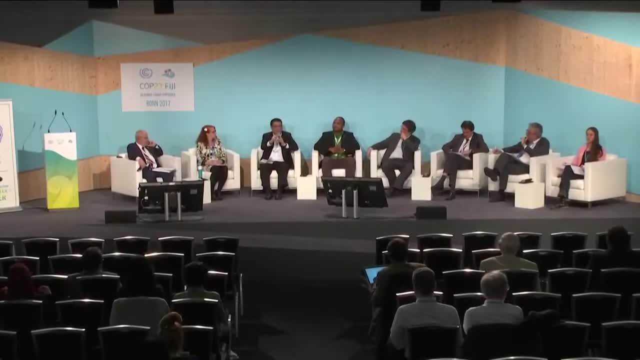 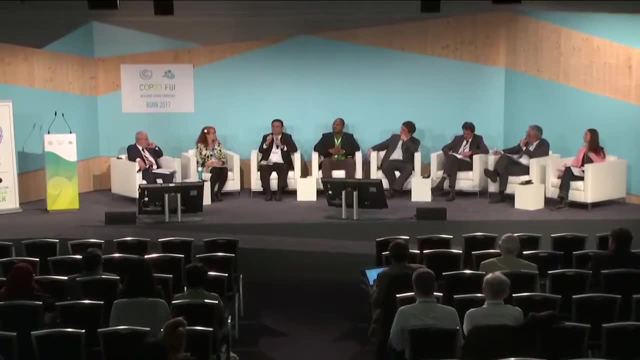 used to do this prevention type of disaster of drought is 25 times cheaper than if we faced with a disaster- 25 times cheaper. So of course, from policy perspective it sends a signal to the Ministry of Finance: you allocate this kind of 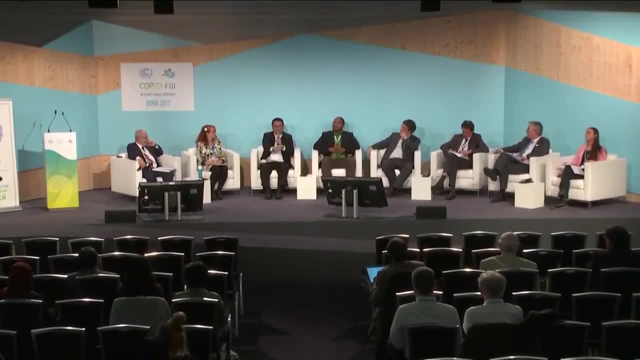 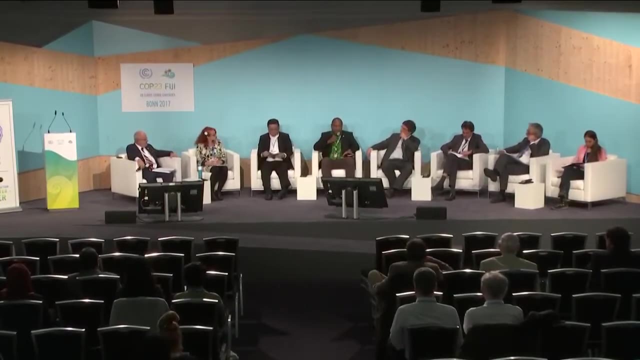 budget for this in comparison for the mitigations of the disaster, And science are very important in telling this modeling. Thank you very much. Thank you And Tekini, Thank you very much In the case for Pacific island states: sequestering carbon. 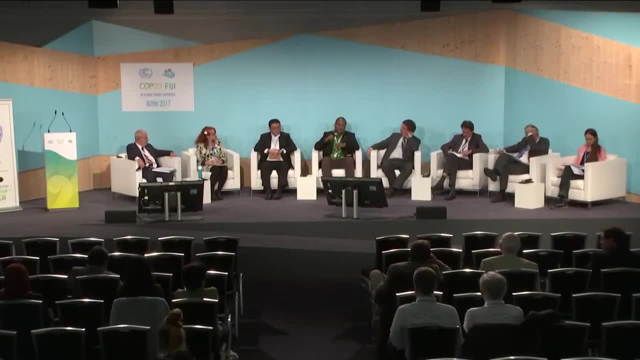 is a traditional agriculture practice for forefathers. Changing into conventional has brought about monocropping and all those. So trying to reverse the process is a bit hard, Trying to convince our farmers to take up all these new techniques that we are proposing. But to 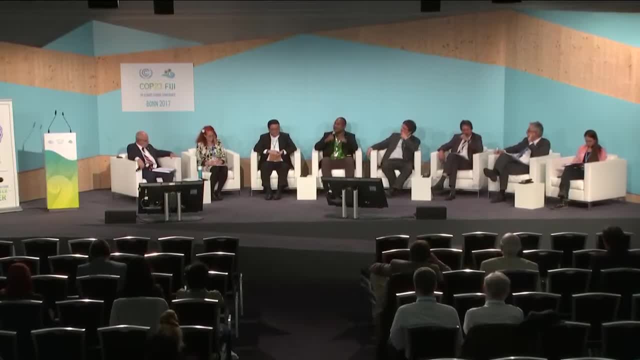 in order to negate all these small emissions that come out from our production, like my colleague said there, we have to increase productivity. Productivity alone will reduce the intensity of the methods of agriculture practice that we employ And also the closed cycle that has been mentioned by my colleague. 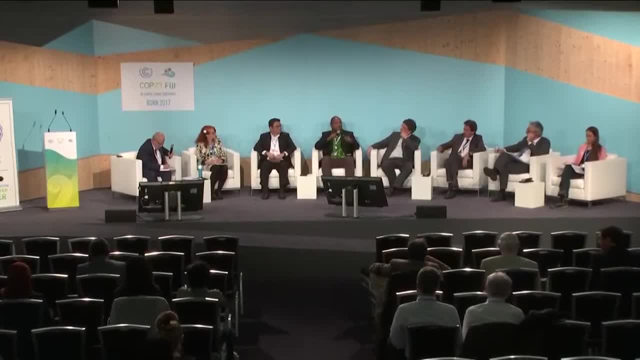 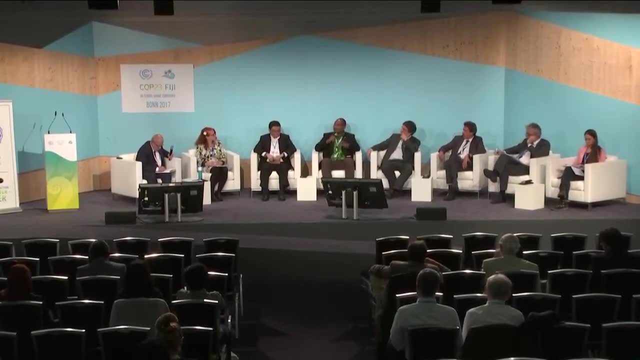 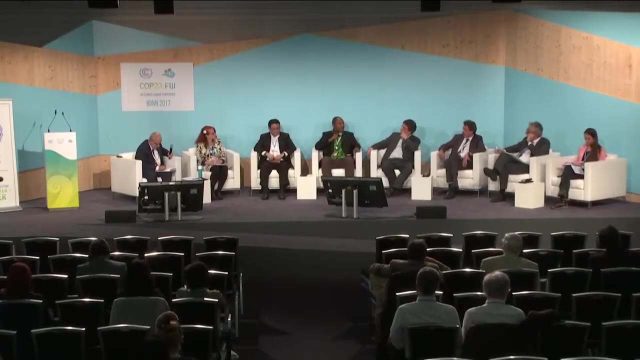 that it is true that carbon and food security and biomass, with that closed cycle we are able to maintain carbon levels in the soil and have that cycle closed for improved food security. Thank you, Thank you very much, Tekini, Luca. we have to. 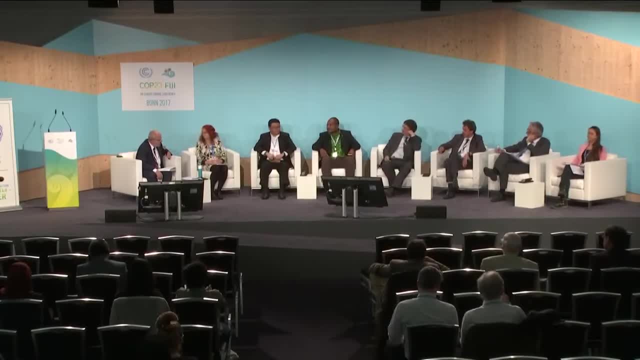 it's very nice to see soil As it is now in the climate agenda, the gaining momentum and the requirement of increasing productivity. that is also a fundamental question. We know that soil organic carbon increase will help us in this regard. We are very optimistic. 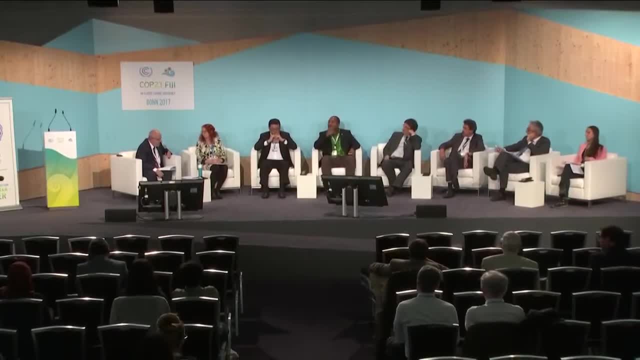 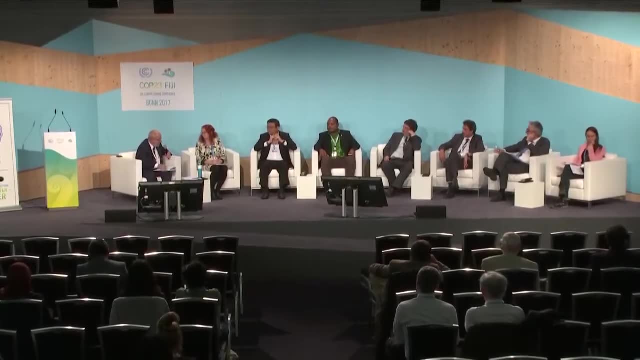 on this. This all have a cost, And science has its own path And we are running against time. How do you put these things together and try to focus on the questions that the colleagues put here to us today. Thank you, Eduardo. 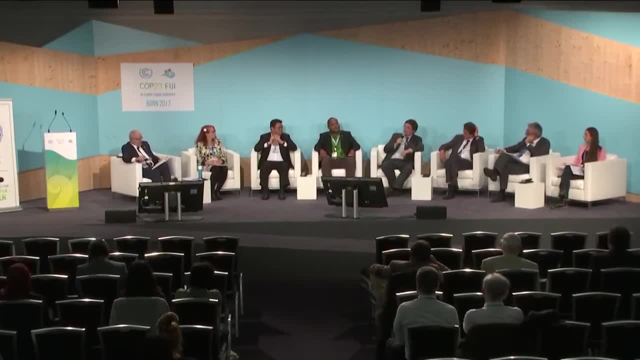 I mean, it's a difficult one, of course, And a complex one, But first of all let me say that really thanks again for organizing this, because it's not the first time that I come to the COP of this convention and we have a discussion. 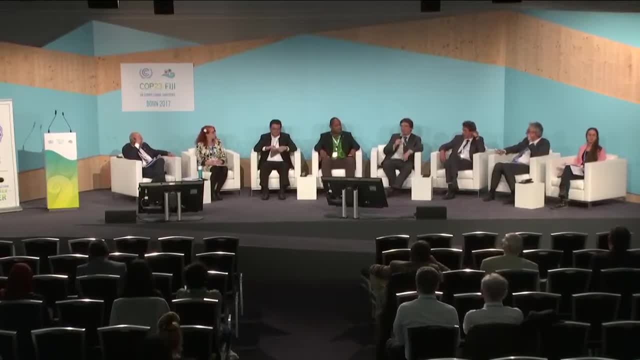 on soil- organic carbon. We had similar events also in previous COPs And I must say it's since COP21 that really we have here momentum, and I would like also to acknowledge the contribution from our colleagues from France in initiating a very strong process in promoting 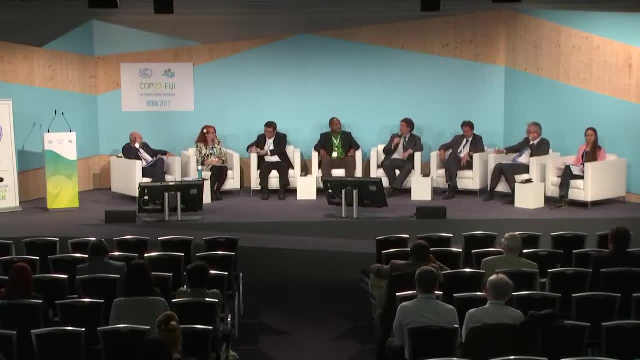 the benefits that we could have by increasing soil organic carbon levels globally. So I would really like to say that there is a big potential that is getting more and more recognized. Coming to the questions, I must say that I don't have the time to respond to all, but I was very impressed. 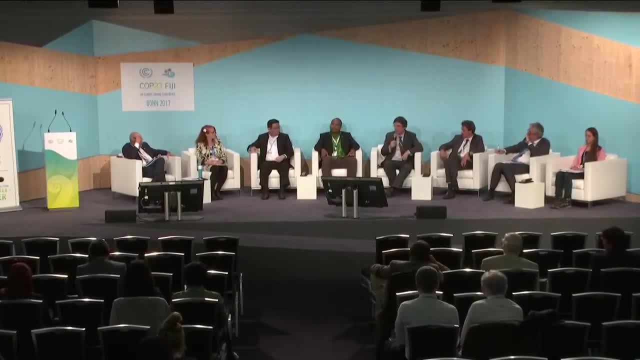 by your question, because you've put the finger on two things which are very important. First, the relation between the terrestrial environment and the marine environment, Which is always forgotten, that we should never consider all these issues in isolation, but there is a very close 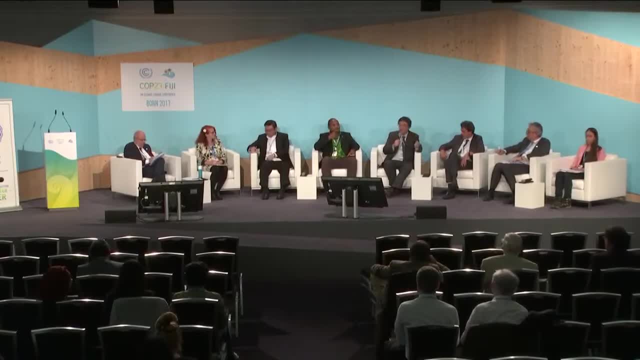 relation between what happens in the ocean and what we do on land And secondly, the issue of biodiversity in soils. This is a very neglected issue in the past. We as Commission have been investing a lot in the past years in raising the awareness that we must invest more. 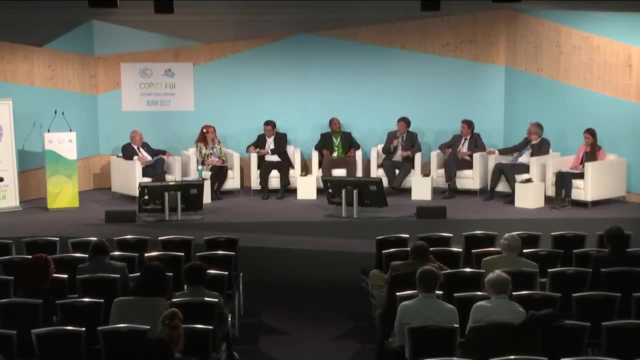 in understanding biodiversity below ground. By the way, we published last year a global soil biodiversity atlas that you may enjoy if you want, and you can download it freely from the European Commission websites. But particularly we are happy that there is now a momentum. We just had a few weeks ago, the global 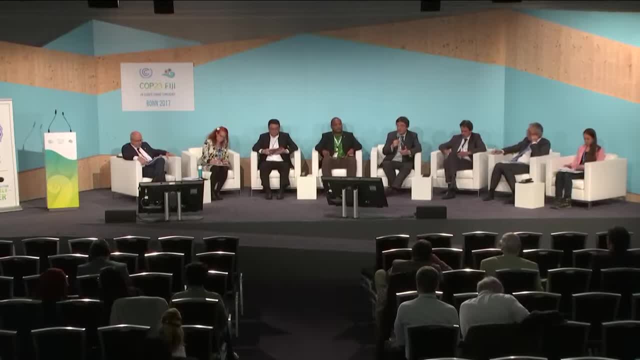 soil biodiversity conference, the second one. And also there is a call to do really something more, related also to what we do within more binding situations like conventions. We should recall that in 2006 we had a COP decision by CBD, by the Convention for Biodiversity. 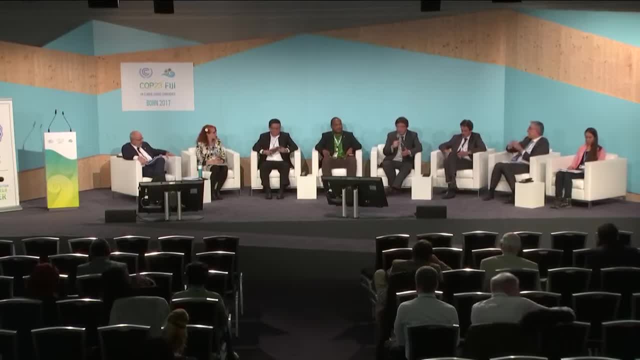 to establish a global soil biodiversity initiative With FAO in charge. So I think there is something there that still needs to be done on that issue that you're raising, and I'm very much supportive of what you're saying because it's something we, at least in Europe, consider. 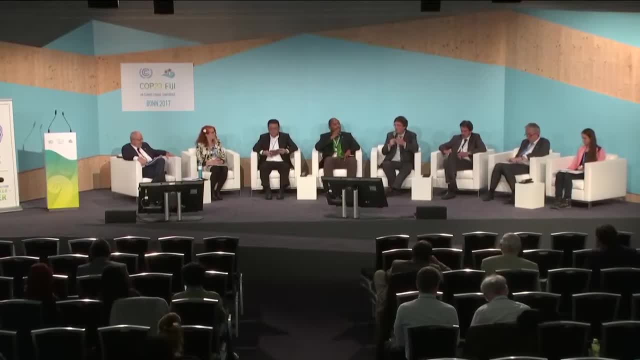 very important. The second question that I would like to spend a few words is the one of Johannes, because you're putting the finger on the problem of the global soil organic carbon maps or global soil organic carbon data that we have, And this is the finger on the fact that 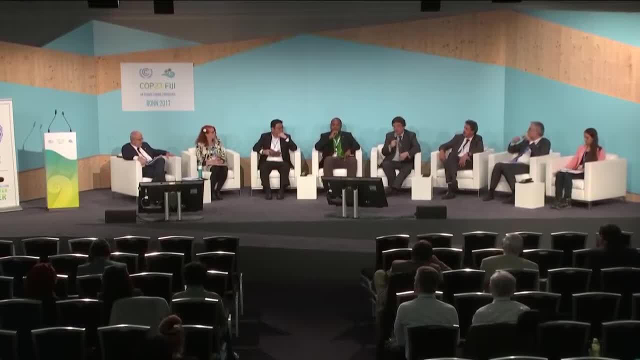 collecting soil data and soil information is very expensive. You need to go on the ground, you need to measure. So the global soil carbon map that we will present in December, which I just highlighted very briefly, is a collection of national contributions that come from very different times. 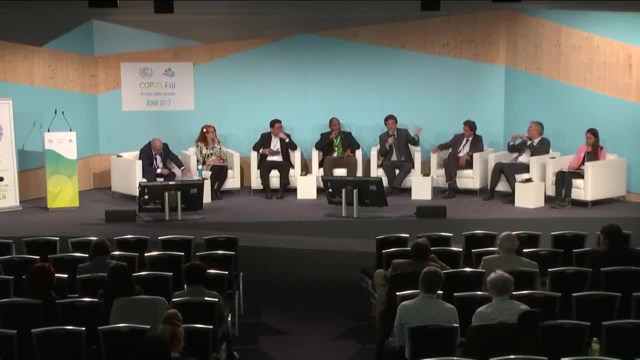 You will have a map made up of data coming on a range from 50 years. So it means some countries provide data of 20 years ago, some of 30 years ago, some have more update information And you are rightly mentioning we can't really. 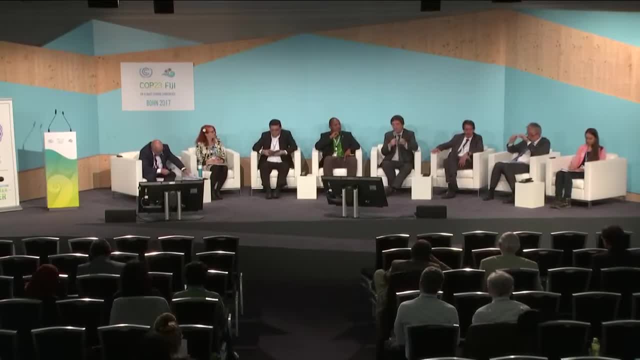 do anything if we don't have the tools to measure change over time of soil organic carbon levels, And this requires, of course, an investment. We in Europe, as the European Commission, have established a system which is called LUCAS, which is a system that measures. 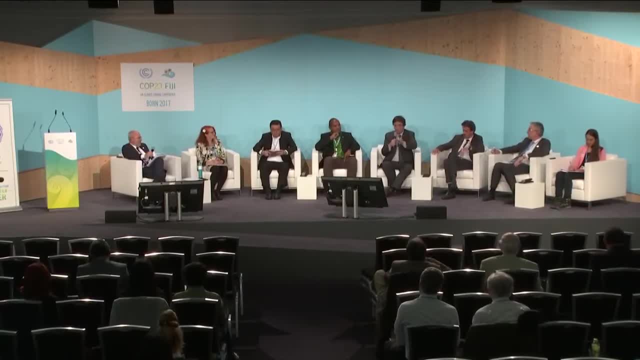 regularly every five years on a point sampling system: soil organic carbon levels. It's a very expensive system. so if you ask me who could host it in the European Union, there is the European Commission, but I'm not sure globally who could do this. maybe FAO. 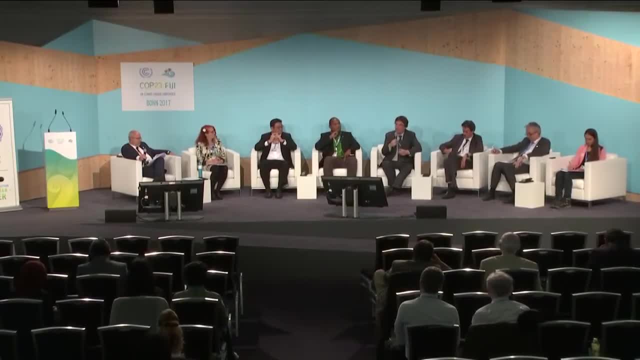 But I don't believe that this is really the solution. I think you need to involve the local land owners and the local actors, so the farmers, in the data collection process as well. I don't believe in a top-down approach so much anymore. but 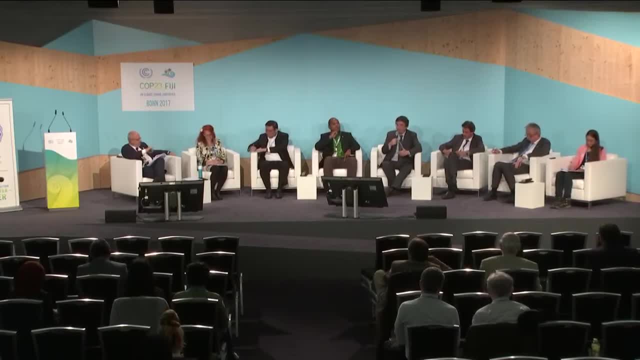 maybe it's my own experience in that. Finally, I would like to say a few words on the lady that was raising the issue that we should not always think only of soil, organic carbon, as the solution for everything. I could not agree more, even though I'm here pleading for 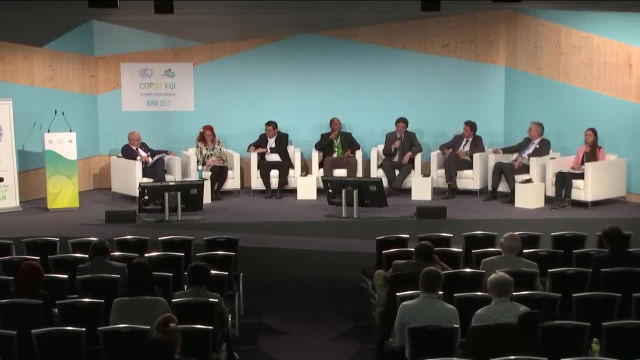 soil organic carbon in this meeting, but definitely you need to consider this in the broader context of what is going on on this planet, And so you cannot consider soil organic carbon as a simple solution for all the complex problems we have. You need to consider all the 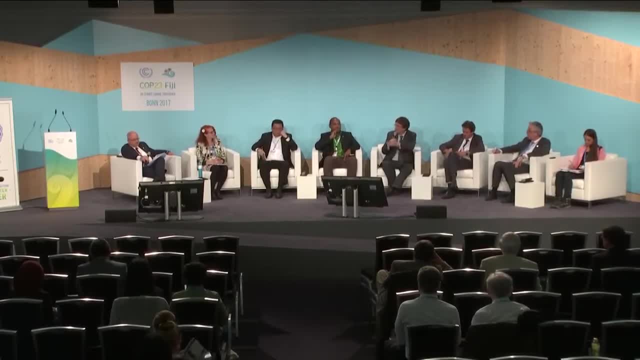 interlinkages with other issues. Many of them have been mentioned during this debate now, but this is really important Now. of course, you wanted to hear about money and this is, of course, the wrong person you're asking, but I can tell you that 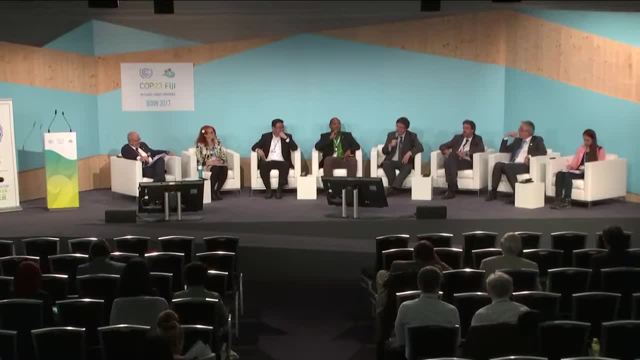 in the European Commission, we are having a very intense debate right now on this issue, particularly because in-house, we have a discussion on our own common agricultural policy, of course, but also on all the development aid that we invest globally. We are one of. 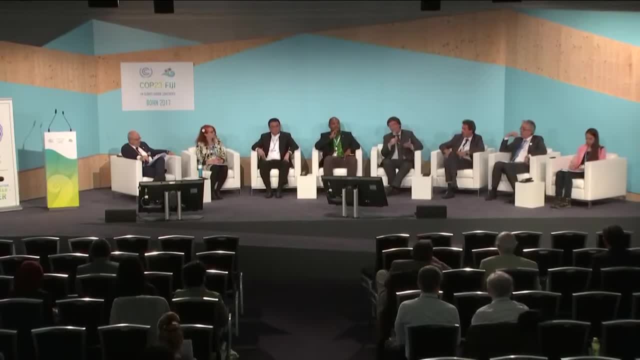 actually the biggest donors globally. So it's a topic that is under discussion because we very much believe it's an important topic. That's why, also, we strongly supported the Global Soil Partnership and its establishment. I hope that we will get more and more momentum also. 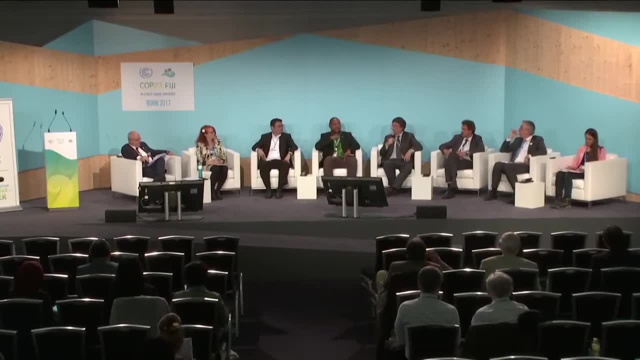 from other sides of the world, not only from Europe, because I think everybody should work together on this, not just in one part of the planet, but it's a global issue and it should be addressed globally. Thank you very much, Luca. 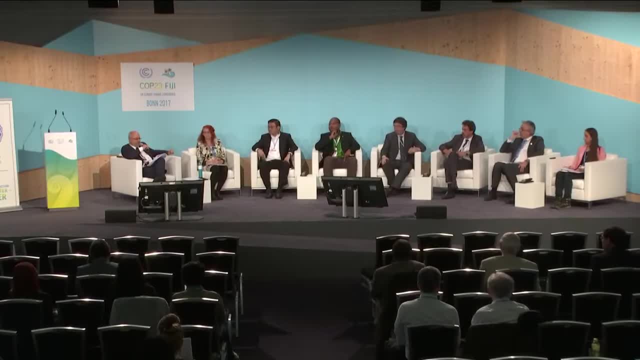 And I would like just to recall very important points that he raised: The protagonic role of France and Minister Lefort in COP21, who raised the importance of soils, and we are an effect of that being here today at this level in COP. so this is thank you. 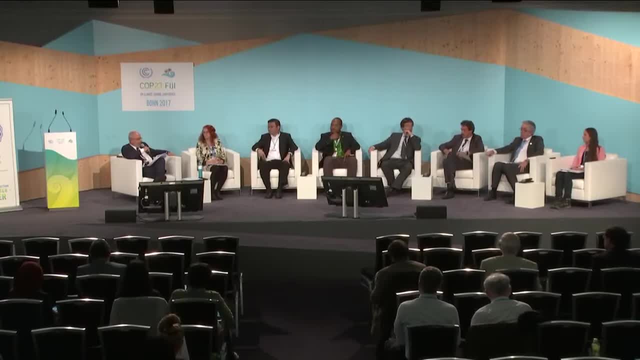 very much for reminding us of the importance. And then the Moroccan government also, in COP22, put a protagonic role on soil and we are very hopeful that the momentum continues. Now the Estonian Presidents in the European Commission, in the European Union, also put soil in. 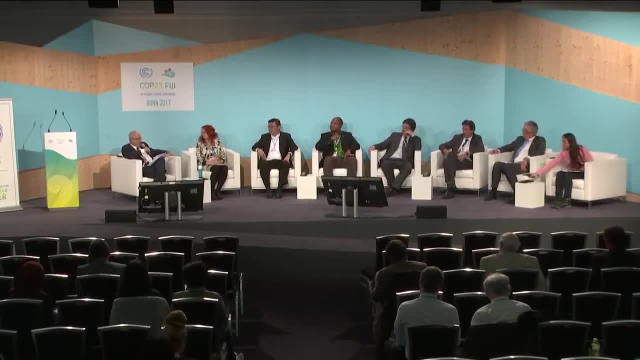 their agricultural agenda as the number one point of debate. It's on soil contamination. Now, as I'm an FAO and Luca mentioned that, who could host the cost could bear the cost of having these global sampling systems. and if people say that, 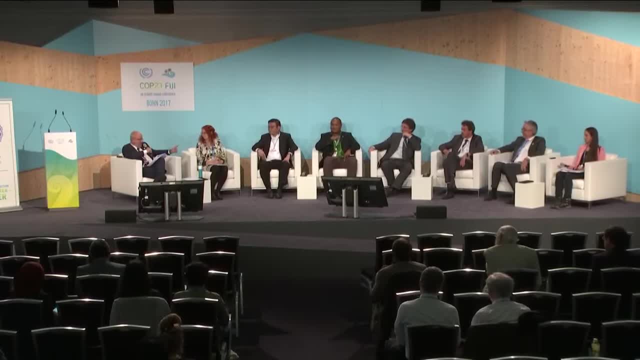 you keep silent. you say it means yes. I have to say something, because we have the same perspective of you. Building country capacity and countries having the capacity for monitoring and assessing their own levels is the only way of coping with a dynamic map. There will be no global 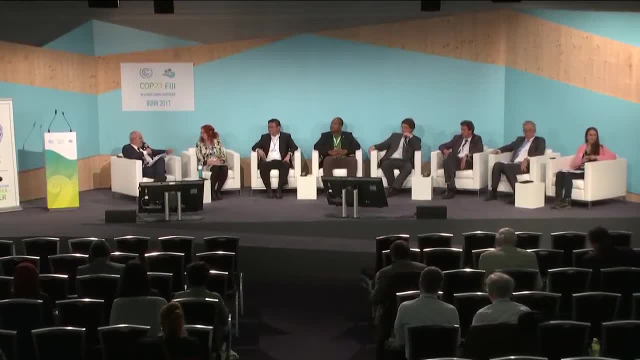 sheriff of the soil carbon of the world. It has to be country by country, producing, generating the data and providing it in a way that we can interpret globally, We can understand and compare, But it's the solution is local, The solution is national. 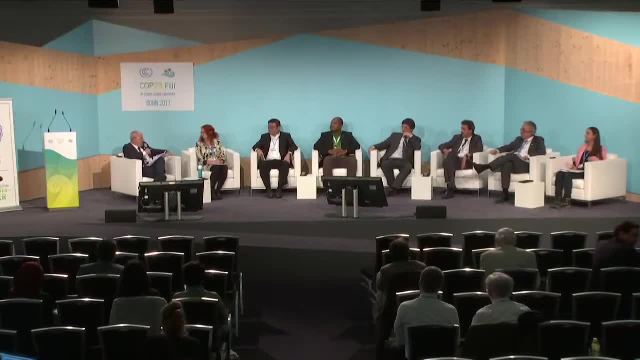 That's the only way that, and this is the way we are generating the global soil organic carbon map that will be released on 5 December that you mentioned to us. I think we did a very big round here and we have to bring this to. 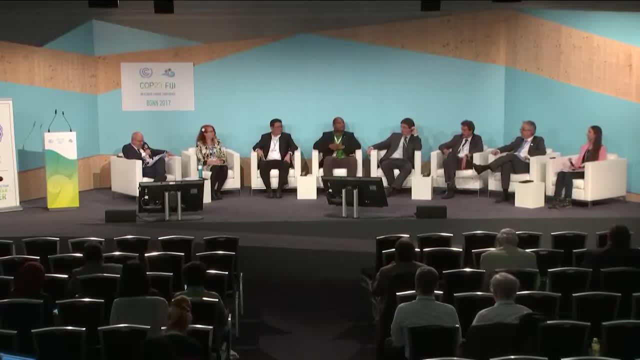 a national, to the farmer's perspective, and Terran Giacomini, from the National Farmers Union of Canada, a member of Via Campesina, has been listening carefully and what will be the take-home message for the National Farmers Association? you? 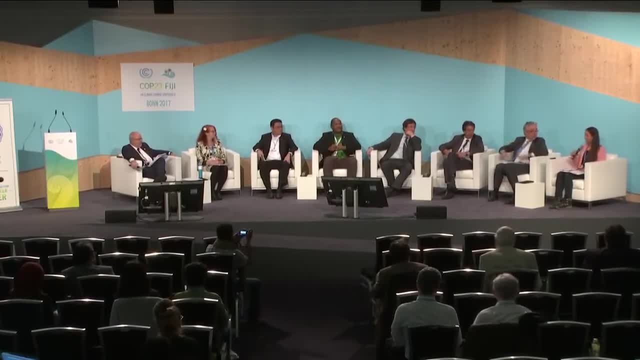 union and for yourself. So first of all, thank you. I appreciate being included in this panel. I think I'm going to frame some points that I've made after listening to all of you, based on some of the work we've been doing. 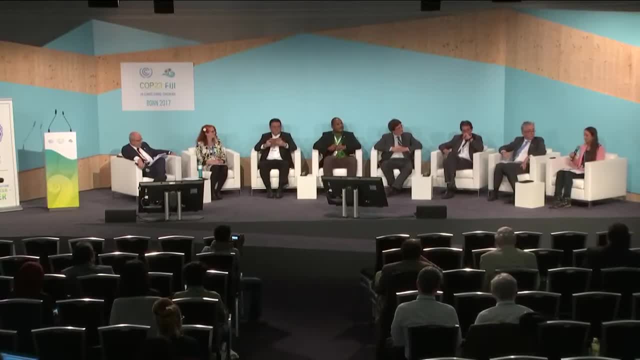 in the Via Campesina around climate change, and I think the main conclusion is really that I think what we're seeing is sort of two different perspectives on both the problem that we're facing with climate change and the solutions- how to approach the climate crisis. 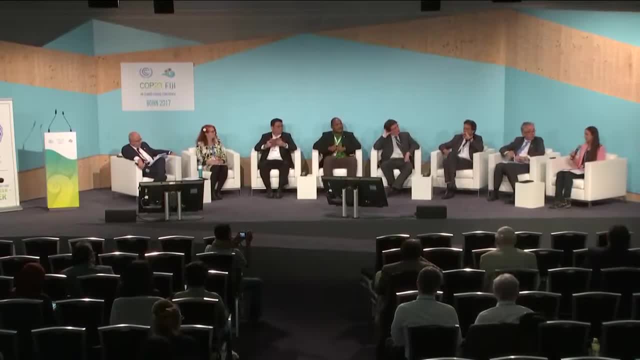 And from the perspective of Via Campesina. climate change is a systemic crisis. It's a problem of politics and economics. It's fundamentally a systemic problem that cannot be solved just with technical fixes or new technology, And we see the solution as rooted. 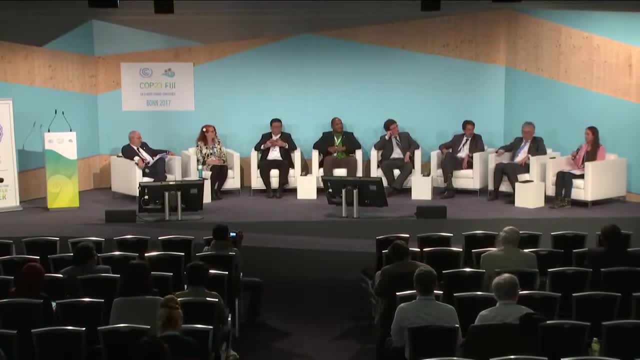 in agroecology and food sovereignty, which means more power for grassroots organizations of farmers, indigenous peoples, peasants and fisherfolk around the world to have real input into the direction of the decision-making that we take on climate change. So, from this perspective, I think 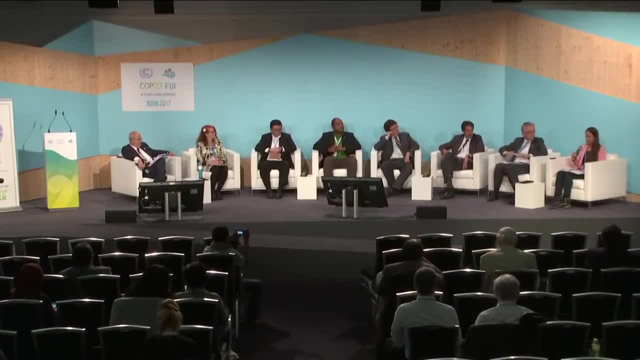 we see two concerns with the approach in the Paris Agreement with respect to what's called the principle of compensation, And we think that this approach is flawed because it views soil as a means to offset emissions and therefore avoids discussion about how to take real action to reduce. 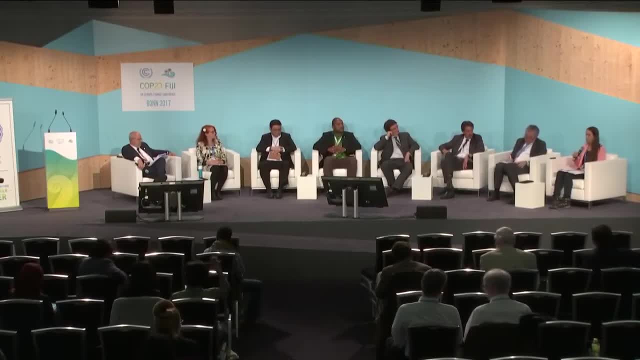 emissions at the source, Both in agriculture, when it comes to phasing out fertilizers and pesticides, or unnecessary emissions in agriculture and in energy, when it comes to actually keeping fossil fuels in the ground. We ask that the negotiators not view farmers as plumbers, you know. 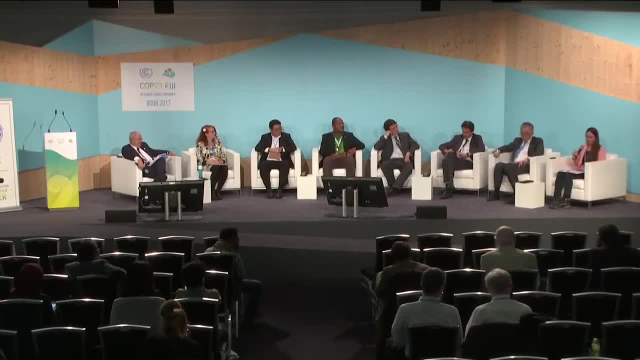 drawing down carbon from that is emitted by the world's biggest corporations, including Exxon and Bayer and Monsanto, who are most responsible for the excess emissions in the atmosphere, But rather to view farmers as primarily as food producers, People who care for the land and love the land. 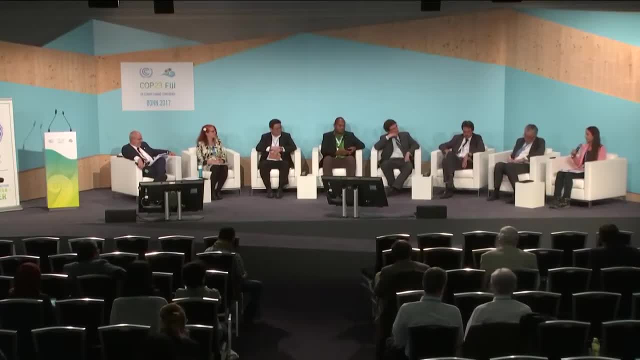 and, primarily, do not view soil as a carbon sink but as, like a child, They view the land as they love the land. We love the land. So it's not just a carbon stock. That's not what we're talking about. That's not the perspective. 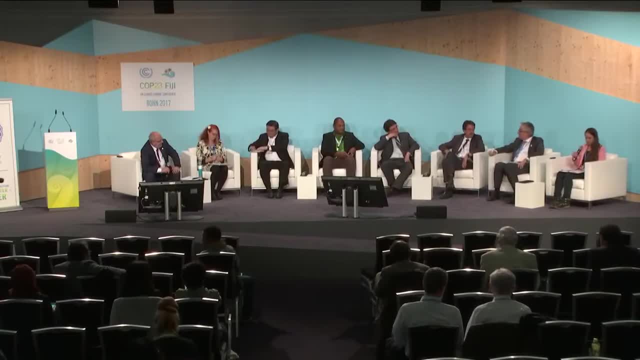 I think the Via Campesina members are very critical of programs including the Global Alliance for Climate Smart Agriculture Which, in the absence of clear criteria, does a balancing act between promoting agroecology and promoting the use of expensive and polluting genetically modified seeds and their herbicides. 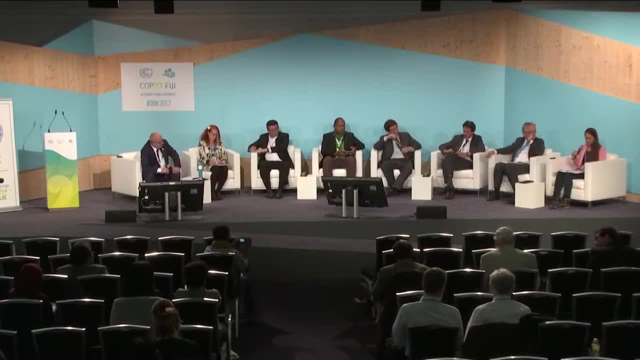 like glyphosate, As well as other technology fixes to address what we know is a systemic problem. 60% of the members of the Global Alliance for Climate Smart Agriculture are, in fact, fertilizer and pesticide companies. This concept of climate smart agriculture is, we see. 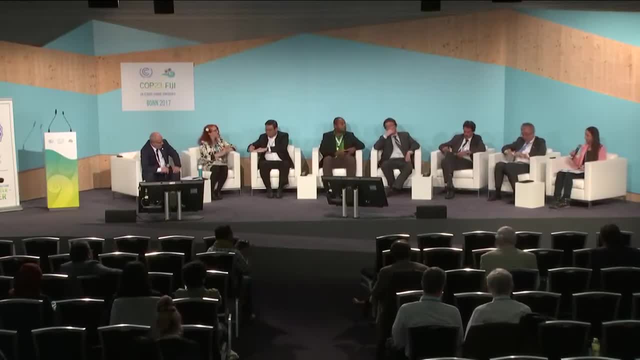 as an empty shell that agribusiness, industrialists and biotechnology companies hide behind while continuing to pump dangerous emissions into the atmosphere. So that's the first point related to compensation versus cutting emissions at the source. Okay, So the next concern has to do with the inclusion of 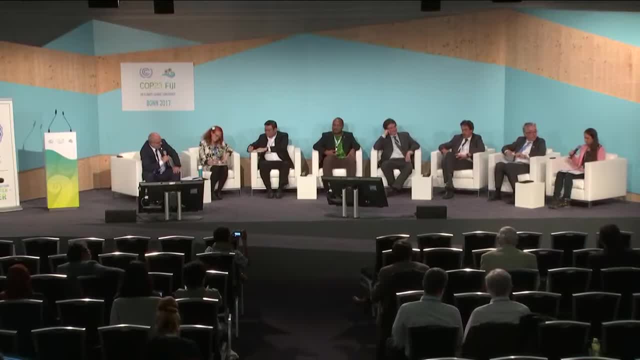 soil carbon in carbon sequestration markets, Which I think was raised earlier. So from the perspective of small scale farmers, I think there's a real danger with soil carbon sequestration in increasing the pressure on land and increasing financialization of nature By putting 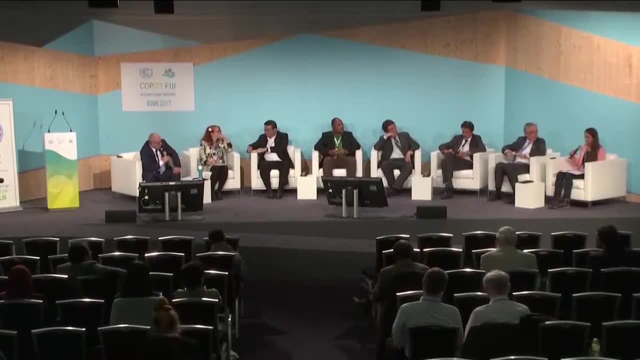 a market value on soil carbon. through compensation as a tool to combat climate change, you increase the pressure on the land And the small scale farmers, who are already victims of climate change, are doubly threatened If we are to encourage investment in agriculture to sequester more carbon. 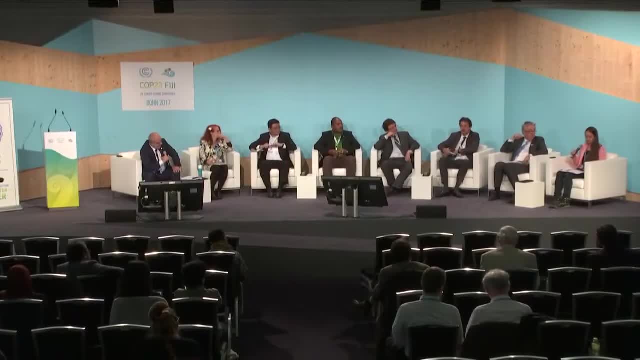 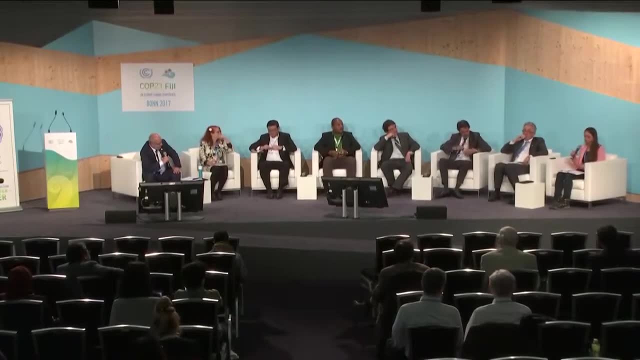 especially from private sources, which with much greater expenses of land. much greater expenses of land will be needed, with an increased risk of land grabbing, which is already a major problem, especially in Africa. The danger will be multiplied by the race for land with paired mechanisms like REDD+. 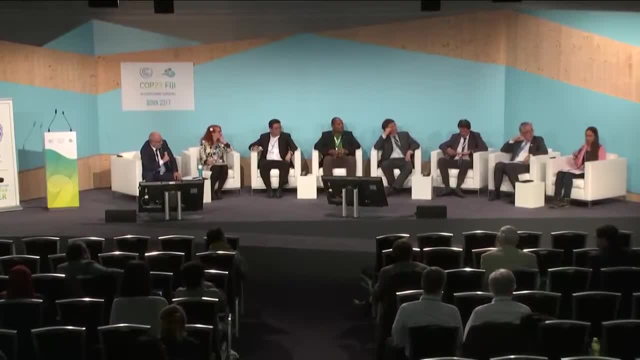 linked to carbon finance, So we see this as a false or a business as usual solution. that's not really a solution, but just a way to make money from climate change. Tehran: we are seriously encroaching the other sessions time, so you have to wrap up. I'll wrap up right now. 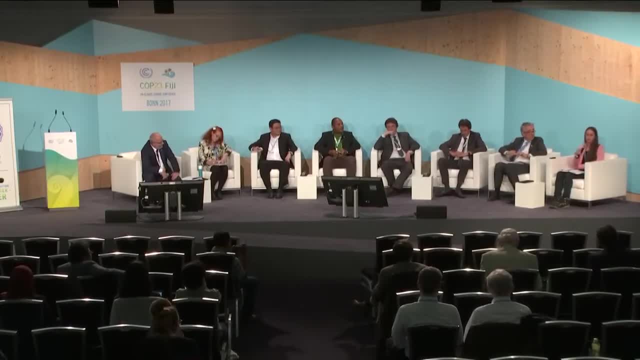 So the bottom line is we cannot let already highly concentrated corporations use climate change to justify making more profits, And we recommend that strong public policies be developed where based on food sovereignty, where the soil and the land is in control of peasants and farmers, and where these climate negotiations 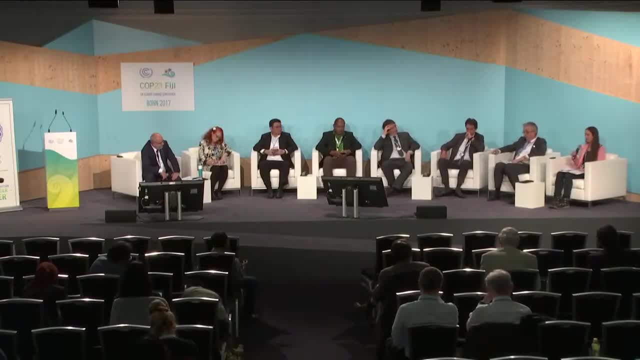 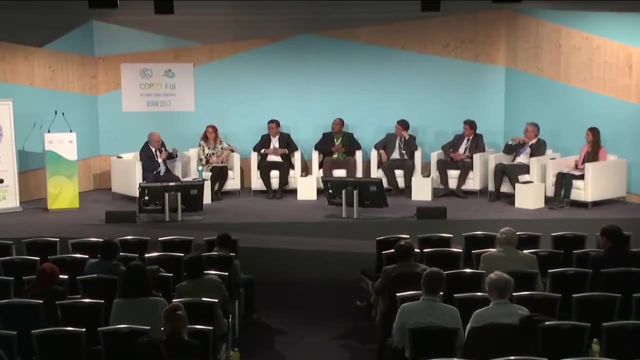 are not used as a mechanism to promote the financialization of nature and land grabbing. I think the applause speaks for itself. Would you like any key message on the soils, specifically that we have been discussing here, or anything? Yeah, okay, Thanks for the opportunity. 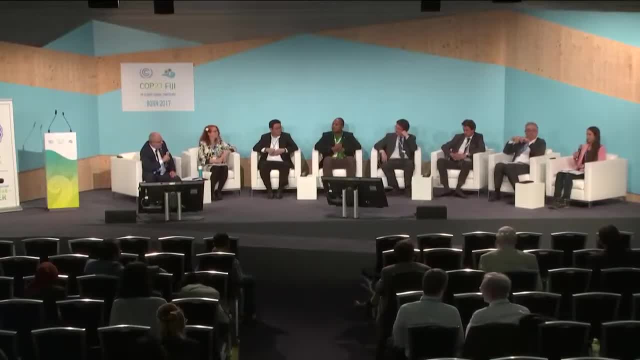 to maybe provide one or two sentences. I think that we're coming from a different perspective. Soil is not to be marketized. Soil is a source of life And that's it. Thank you so much. I think we have to come up with a round of applause for.